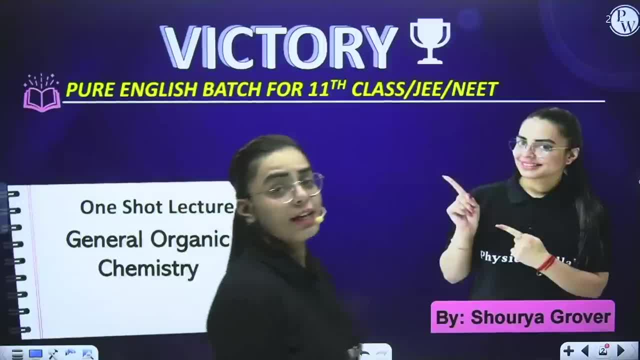 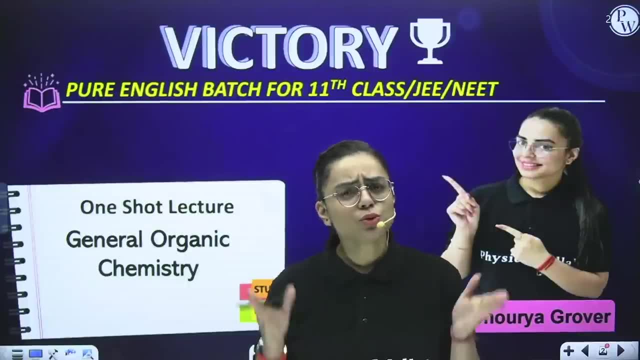 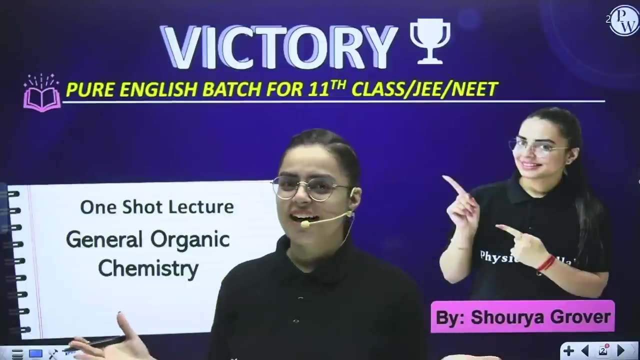 Every morning you have 2 choices: Continue to sleep with your dreams or wake up and chase them. So hello my shimmering stars. Aishwarya is going to start our one shot lecture on General Organic Chemistry Students. as you all know, in our victory batch we have already covered IUPAC and Isomerism. 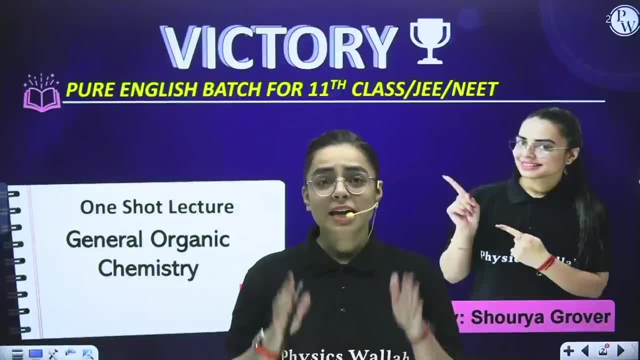 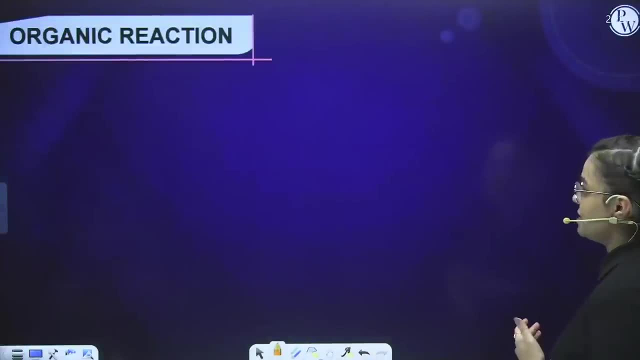 Now the third topic is going to be General Organic Chemistry, which is going to be very, very important for your competitive exams. Now, students, if I move forward in what topic we are going to start today is, First of all, we need to know why there is a need for General Organic Chemistry. 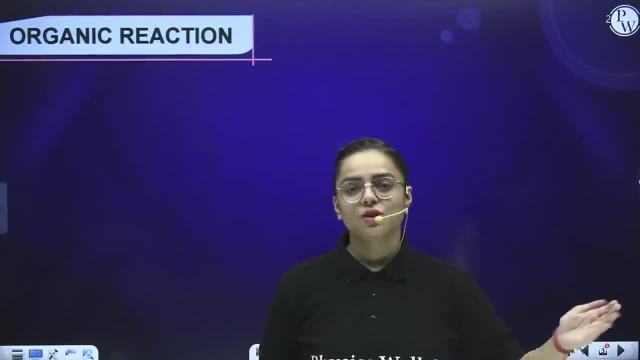 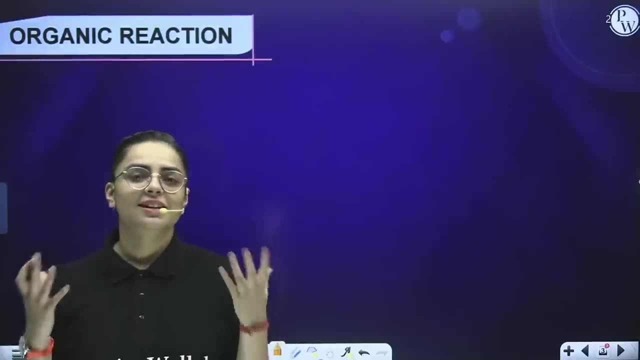 And how we are going to proceed in this further lecture. So, students, first of all, the need for General Organic Chemistry arised due to organic reactions. If I talk about a simple organic reaction, I would say what comes in my mind. In my mind comes that reactants gives product. 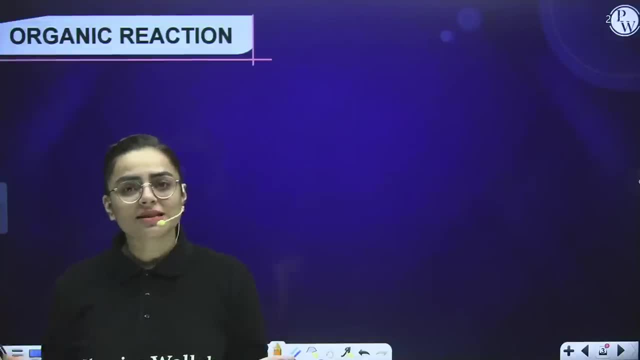 What happens in reactants: Old bond breaks and new bonds are made. that is the product formation. So if I talk generally, what do you mean by that? What do you mean by any reaction? I would say generally: a chemical reaction involves the reactant in which bond breakage occurs. 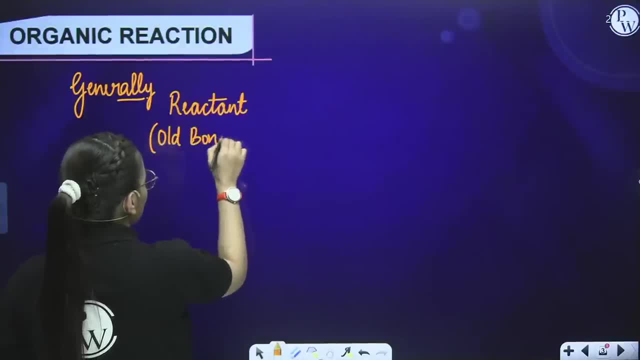 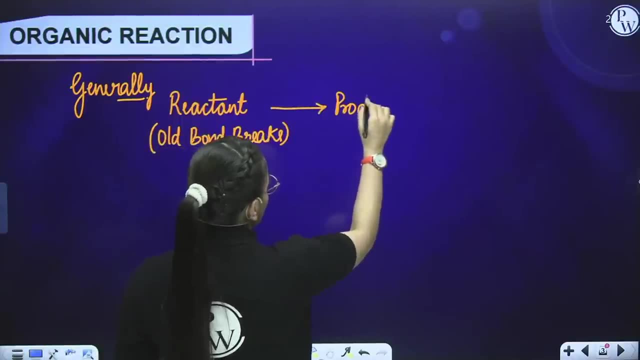 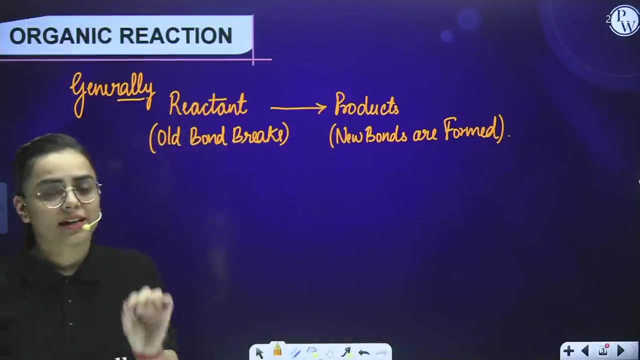 That means old bond breaks, and hence we get products in which new bonds are formed, But in actual students, this is not the correct order of you know the organic reaction. How does an organic reaction occurs? First of all, we require a substrate. What happens? 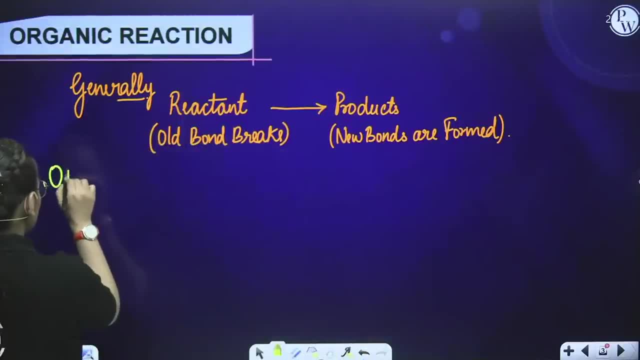 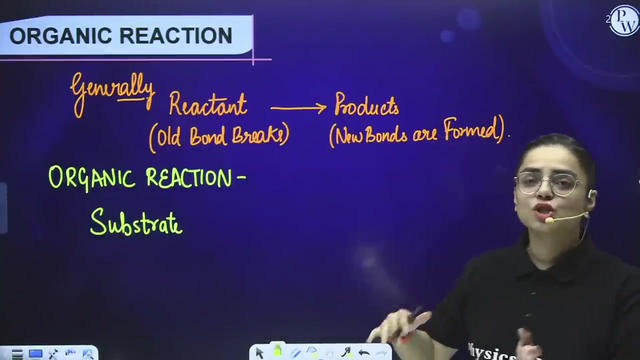 How does an organic reaction occurs? This was our basic. you know the definition, I would say, for organic reaction. Now, what actually is organic reaction? I would say we require substrate. What we require Substrate. Now there is an attacking reagent which attacks on the substrate in the presence of some medium that is known as solvent. 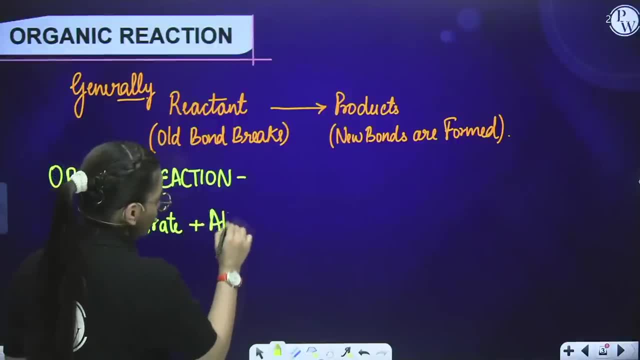 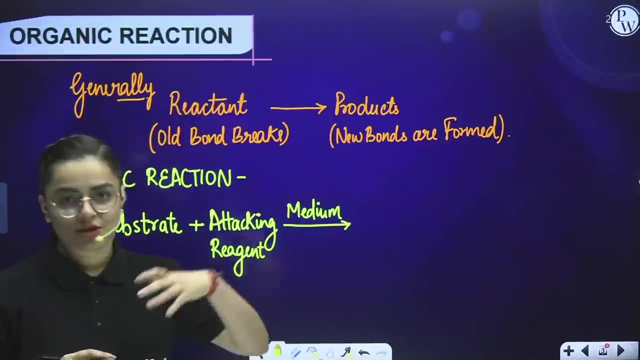 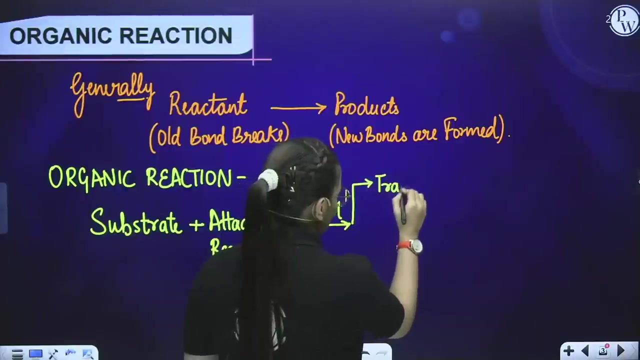 So what happens On substrate attacking reagent attacks in the presence of medium Which can either lead to the formation of transition state or to the formation of intermediate first, Which can either lead to the formation of transition state or it would lead to the formation of intermediates, or you would say reaction intermediates. 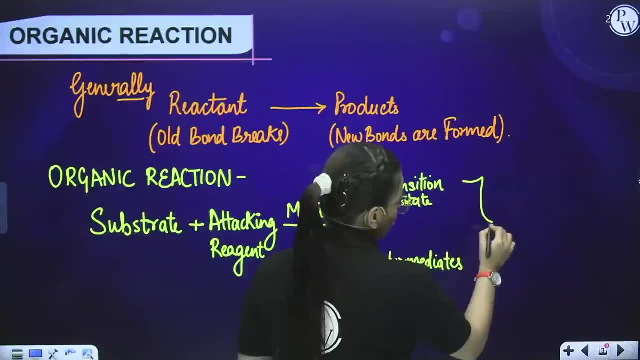 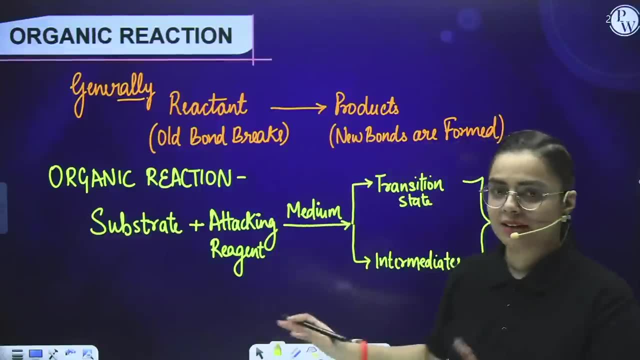 It's the same thing right, Which further students, Which further gives us product. So this is the actual meaning of organic reaction, or how does an organic reaction occurs? Now, if I talk about substrate or attacking reagent, Now which substrate I should use or what kind of attacking reagent is required for, in particular, organic reaction to occur? 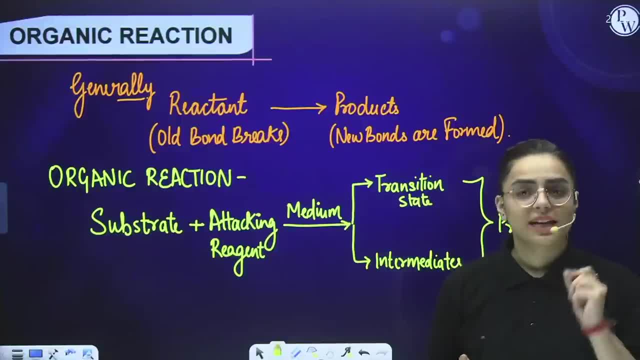 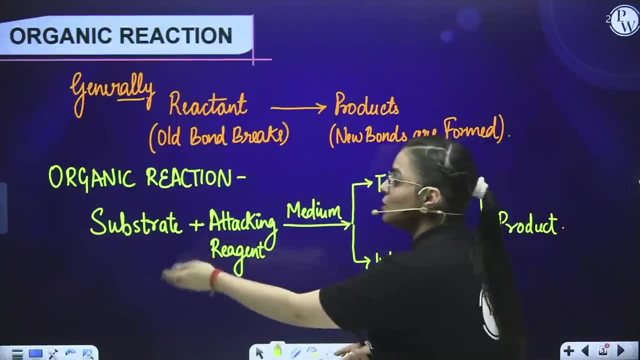 I would say this all depends upon electron density. If the electron density is high or the electron density is low, The attacking reagent will be with respect to the substance. The attacking reagent will be with respect to the electron density it would attack. 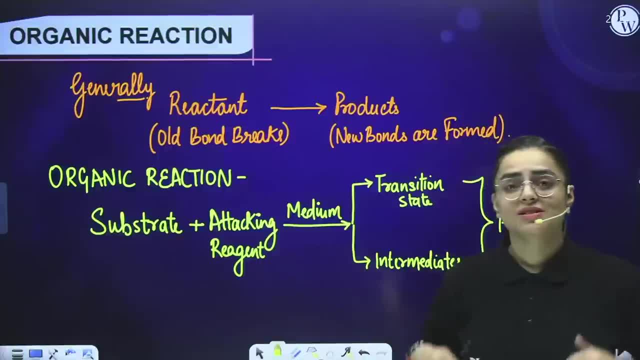 If I say the electron density of the substrate is high, then the attacking reagent which is attacking on the substrate will have electron density low. And if I say, here, the substrate which is present has electron density less, Now the attacking reagent which is going to react with it will have electron density more. 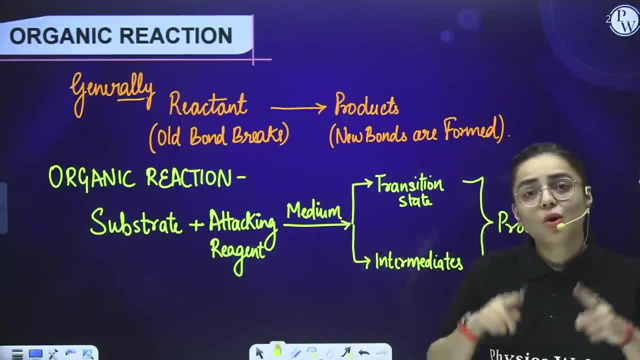 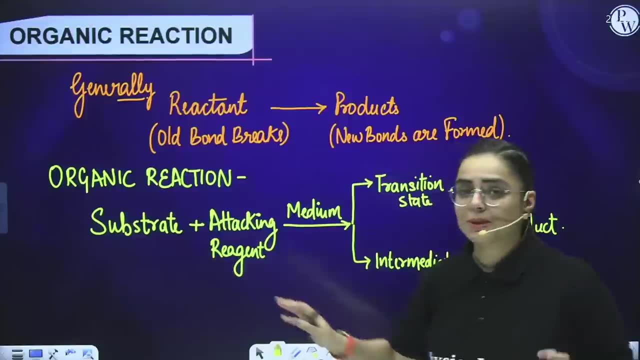 So it is vice versa for both of these cases, right? So this all depends upon what Electron density. Now, what we are going to do Now, what we are going to see. first of all, we are going to study about substrate, That means in the substrate. we are going to see the electronic displacement concept. 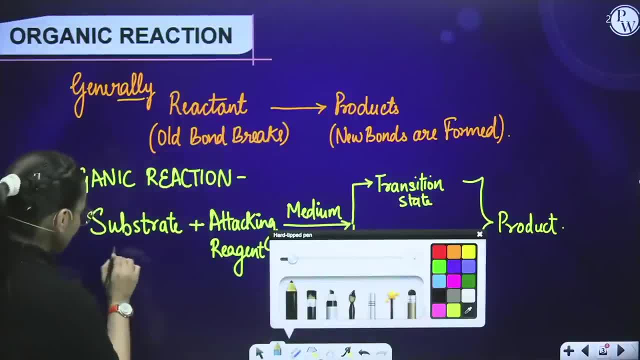 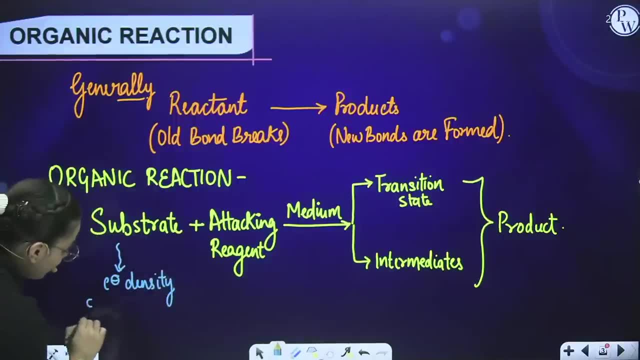 What we are going to see. We are going to see under this: first of all, I am writing electron density because it depends upon electron density. Second thing we are going to cover here about electronic displacement. We are going to cover about electronic displacement. Then, as I told you, that, depending upon the substrate, there is a something I would say attacking reagent that is going to react with it. 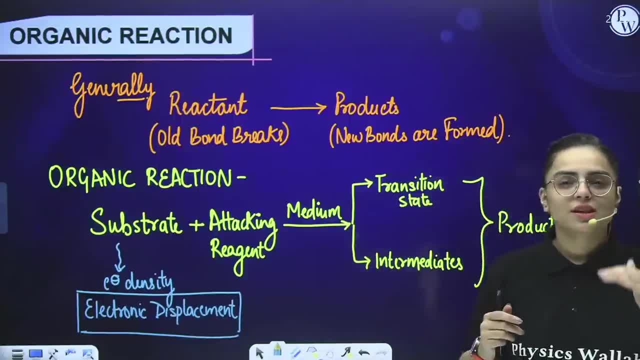 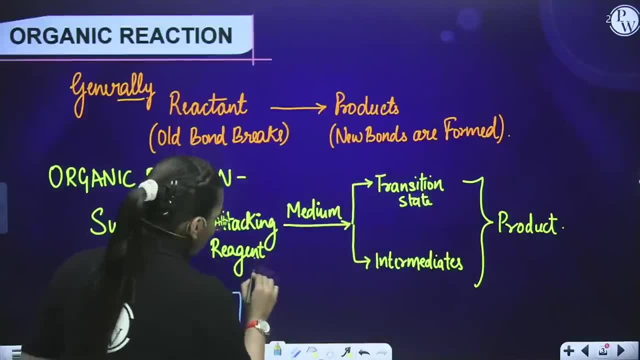 So if electron density students, if I would say it is less, then electrophile will attack, if it is more, then nucleophile will attack. So in attacking reagent topic we are going to study about electrophiles and nucleophiles. Here we will cover these two things. 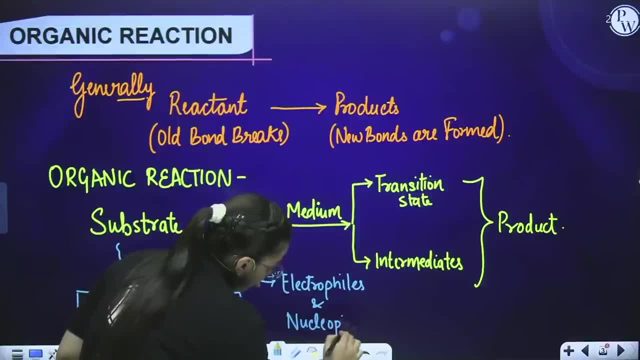 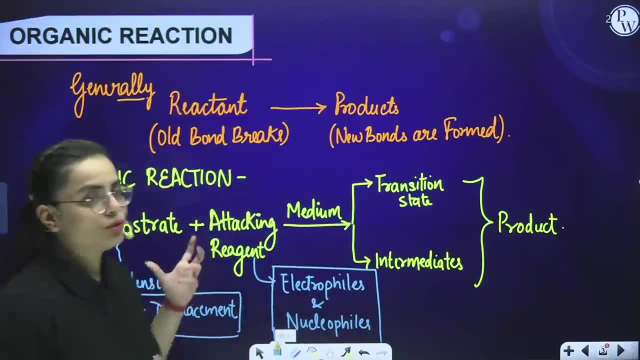 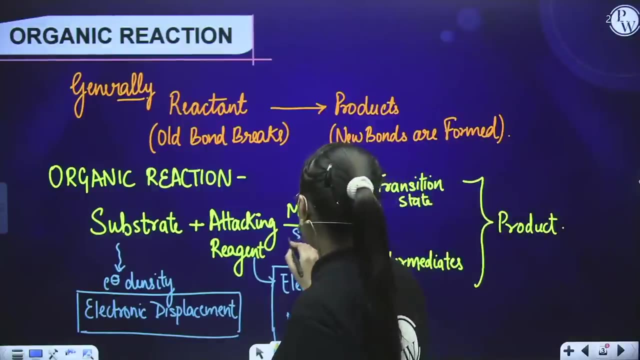 So we are going to study about electrophiles and nucleophiles. Here we will cover these two things. So we are going to study about electrophiles and nucleophiles. Now, if I talk about the medium, here we are going to study about the solvent in which it is going to react, right? 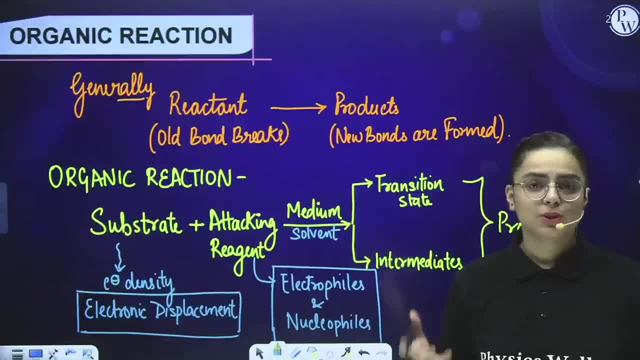 Here we are going to see about the solvent. Now the next step which comes: the transition state, or I would say intermediate. now, what is the transition state? again, Where old bonds are broken and new ones are made right. And if I talk about intermediate, 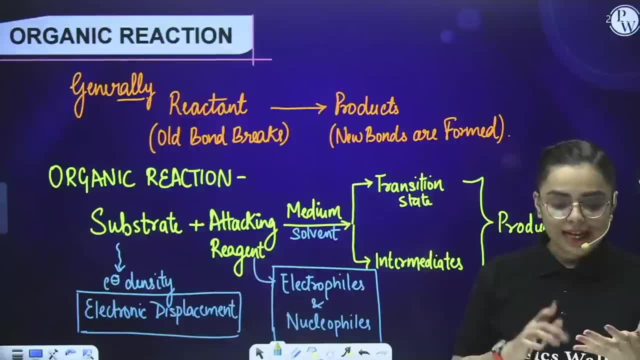 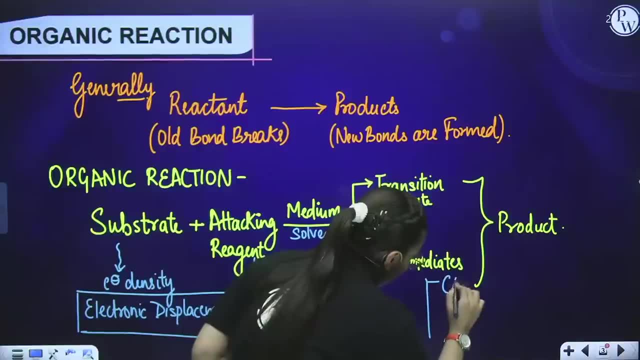 Which is going to be the very most important topic in the GoC. in the GOC, that is intermediate. it can be carbocation, it can be carboanion, it can be carbon free radical. So here we are going to see the three categories. that is carbocation, the second one, we are 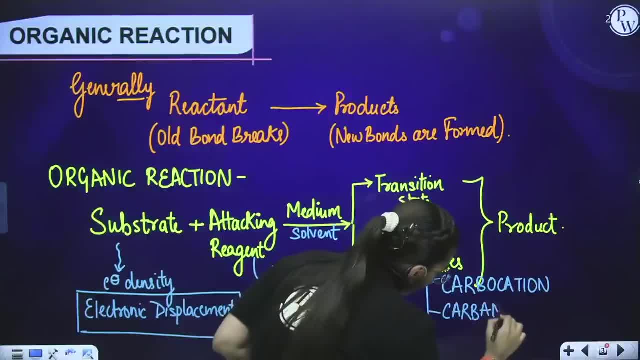 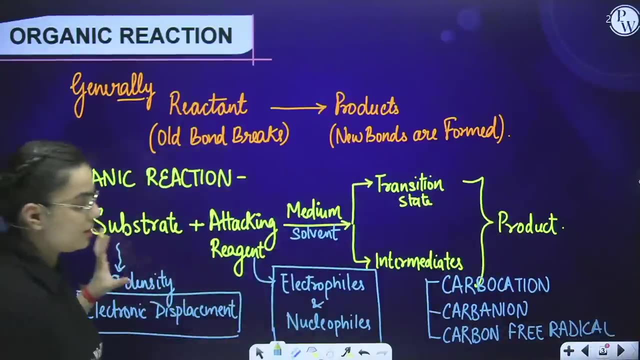 going to see is carboanion and the last one we are going to see is carbon free radical. So this is going to be the- you know, the wave in which we are going to study the GOC. First of all, we are going to study about electronic displacement, then we will move forward towards 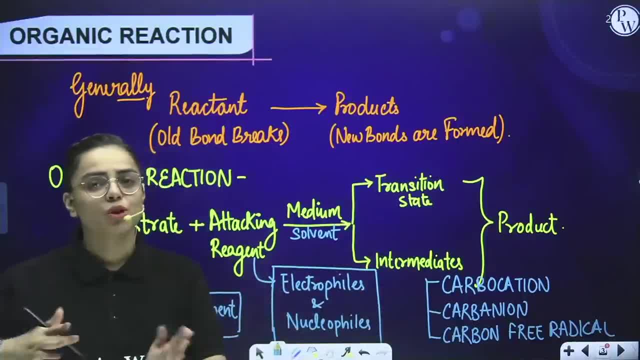 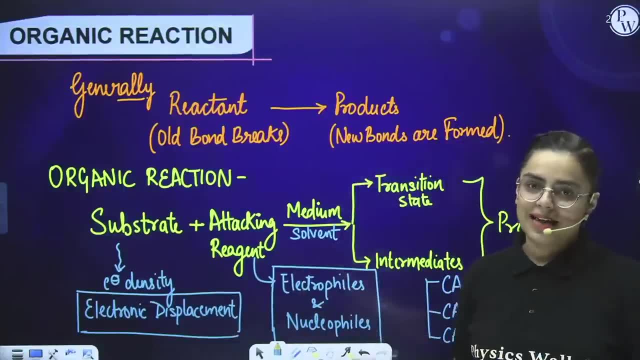 electrophiles, nucleophiles, and further towards the carbocation, carboanion and carbon free radical. So, one by one, we are going to understand the general concept of any organic reaction. right Now, see, students, if I talk about the very first concept, that is, electronic displacement. 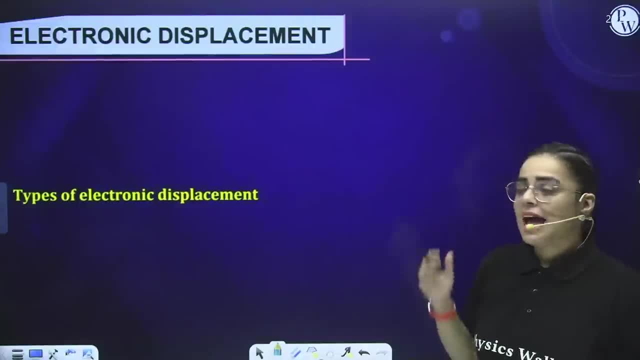 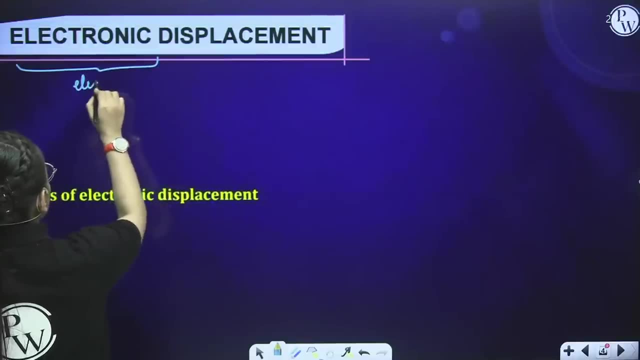 as the word itself says, Electronic refers to the electron and displacement refers to the movement. So what is here seen? electronic refers to what it refers to, electron, while displacement refers to what movement. So what we are going to see here, we are going to see the movement of electron. we are going 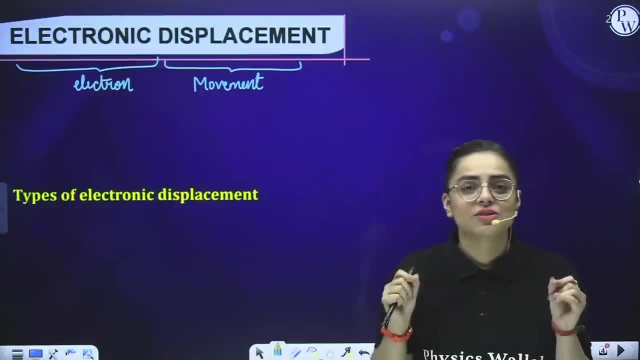 to observe the use of arrows in the general reactions You would have seen. in many of the cases while solving the question papers or while attempting the questions, you observe that we generally observe that there is a use of arrow in resonance. you have seen right, So I will tell you how to use arrow, in which direction or how we are going to see the movement. 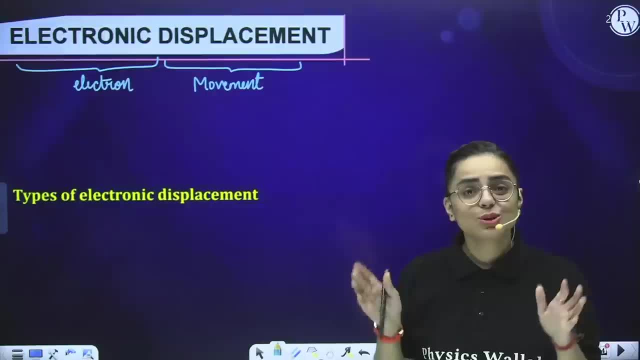 of electron from one position to another position, How the electron movement is being shown with the help of certain diagrams. So, one by one, we are going to understand the very basic concepts of organic that we need to understand, and if we get this basic concept, then further organic chemistry is going to 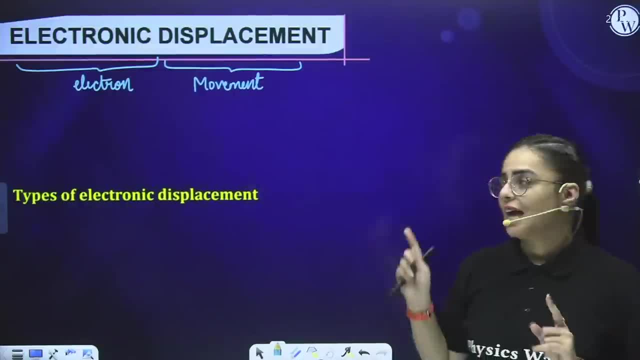 be very, very easy for you people, Now students. as I said you, electronic displacement is the movement of electrons that we are going to see Here. we are going to check about electron density: Where is electron density more or where is electron density less? right, 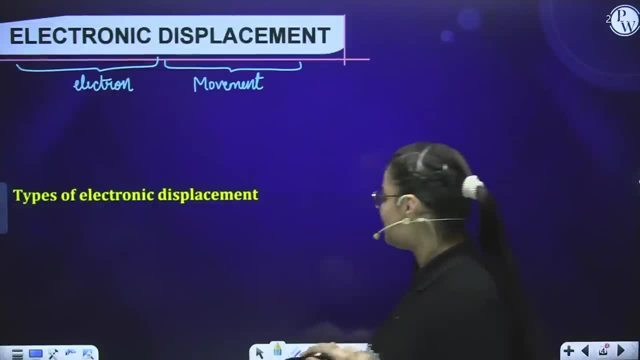 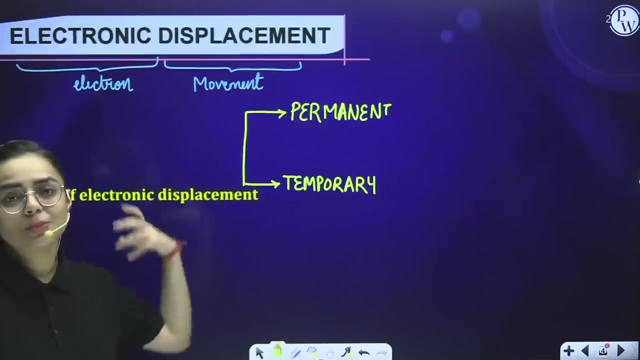 Now, if I talk about the types of electronic displacement, that is of two types. Now, this is of two types, students. one is permanent, one is permanent and another one is temporary. Okay, One is permanent and another one is temporary. Now, if I talk about the kind of permanent effects, 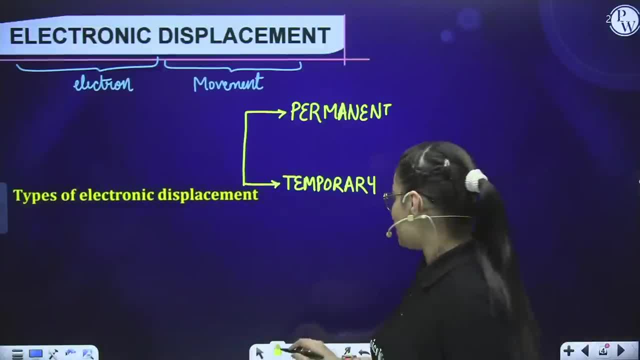 Now these are further classified into three subcategories. Now, what are these three subcategories? The number first that we are going to start today is all about inductive effect. First is inductive effect. Inductive effect. The second is inductive effect. 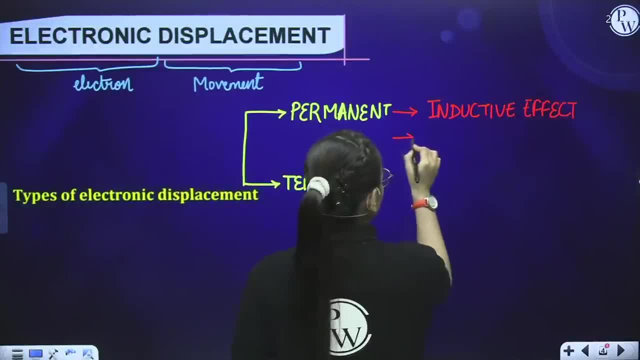 Inductive effect. Inductive effect, The second that we are going to study over here is going to be resonance, or mesomeric effect, or mesomeric effect. and the third one, which we are going to observe over here, only that, is going to be hyper conjugation. 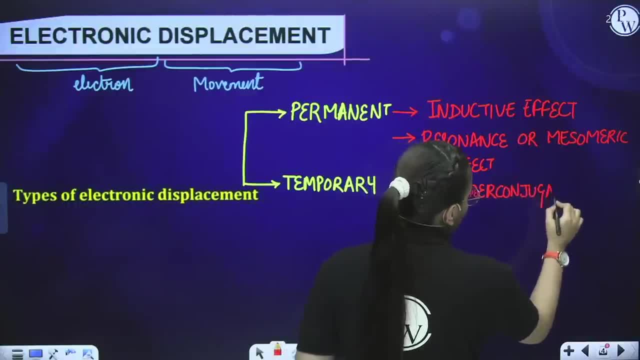 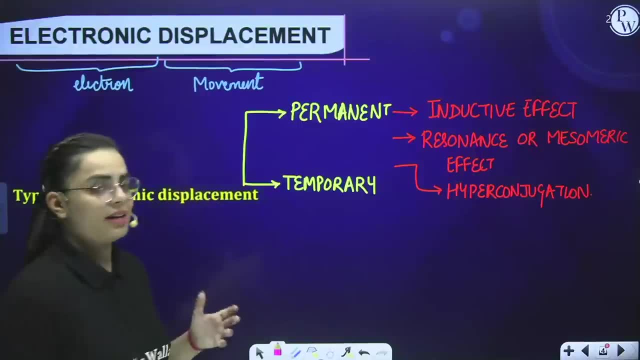 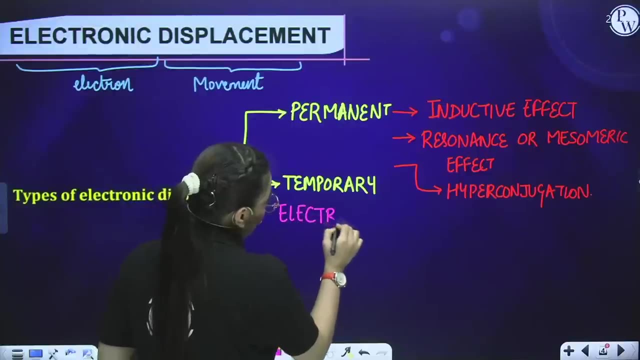 Hyper conjugation. Now, if I talk about the temporary effect, Now, the temporary effect, students, if I talk about the temporary ones, the temporary ones are classified into electromeric effect. It contains electromeric effect. Okay, now, as it is temporary, we are going to say here only at a certain limit of time. we 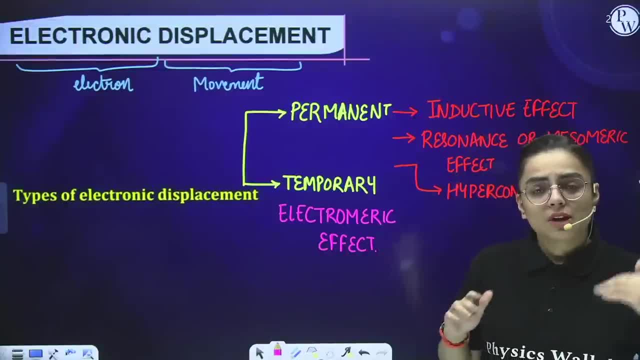 see, the attacking reagent is attacking, So we will see what is the permanent effect that lasts for long time. What is the permanent effect? What is the permanent effect and temporary is the one which doesn't last for long time. so these are the types of electronic. 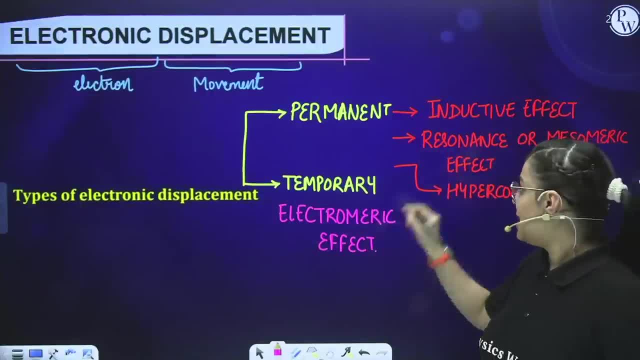 displacement, which are further classified into permanent and into temporary. permanent are further classified into what it is further classified into inductive effect, which is represented by capital i. if i talk about resonance or mesomeric effect, i would say it is represented by m or r, okay, and if i talk about hyper conjugation, it is represented by h or u. 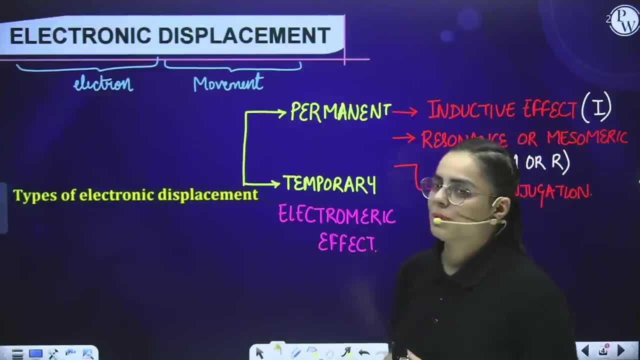 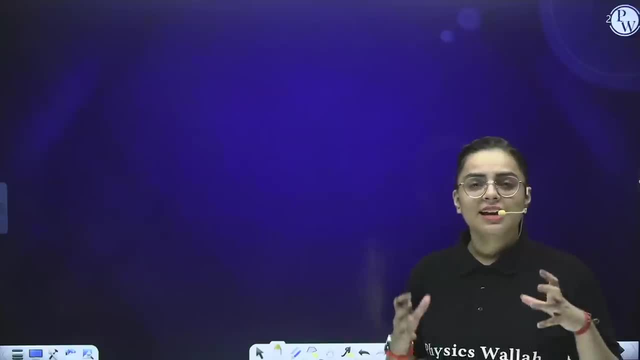 directly right, hyper conjugation, right. and the last one is electrometric effect, which is a temporary kind of effect. now, further moving, further moving to the next topic, i would say: let us take some general knowledge that is going to help us in the organic chemistry today. okay, so, 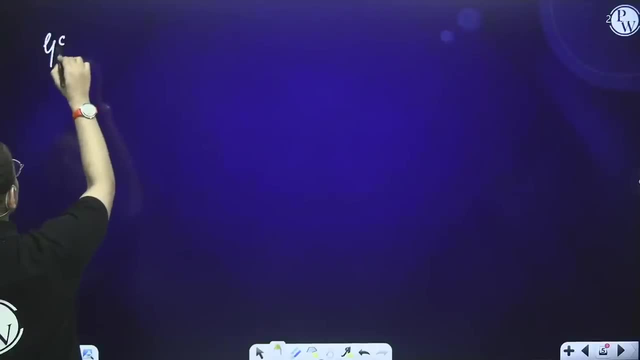 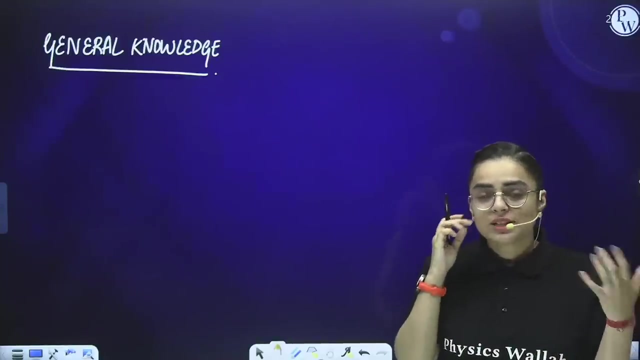 what is the general knowledge that we require here? what is the general knowledge required over here? now, here i will be talking you about electronegativity. what do you mean by electronegativity? first of all, i want you people to answer me. electronegativity, as i've already explained you in some of the cases that 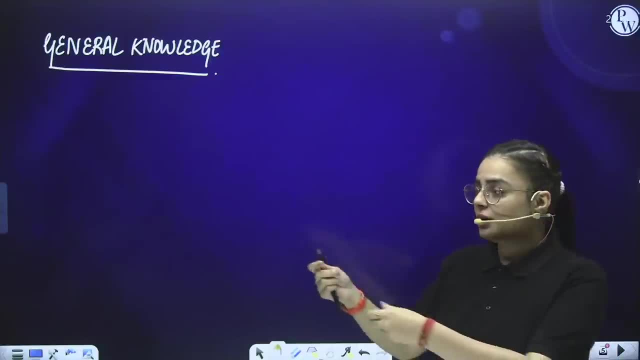 electronegativity is basically, you know, the attraction of certain pair of electrons, the tendency to attract certain pair of electrons. that is electronegativity, right? so according to electronegativity, if i say there are two atoms that are bonded, a and b are the two atoms. now, if 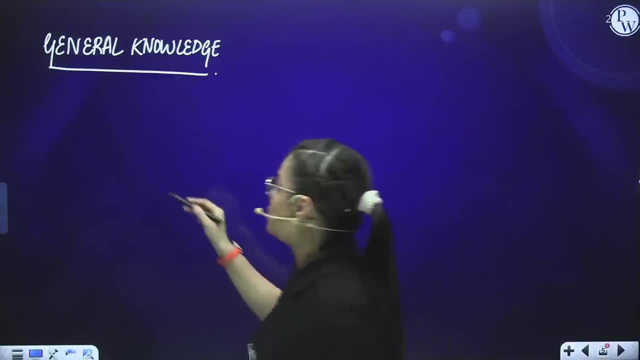 i would say a and b are bonded with each other. if i would say a and b are bonded, then how many electrons are present between this bond? you will say, ma'am, two electrons, because one bond contained two electrons. yes, one bond contained two electrons. that means here: which kind of bond do you observe? here is. 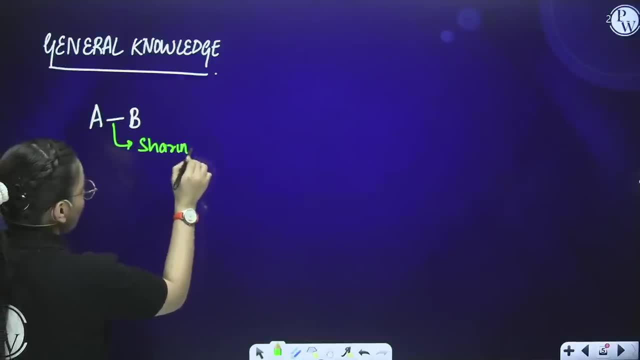 sharing of electrons. here is sharing of electrons. right now. this sharing of electron occurs, in which case in covalent bond. so this is a kind of covalent bond, right ma'am? okay, now let me tell you one more thing, students. if i talk about electronegativity in, and if i say if i have this a b molecule with me, 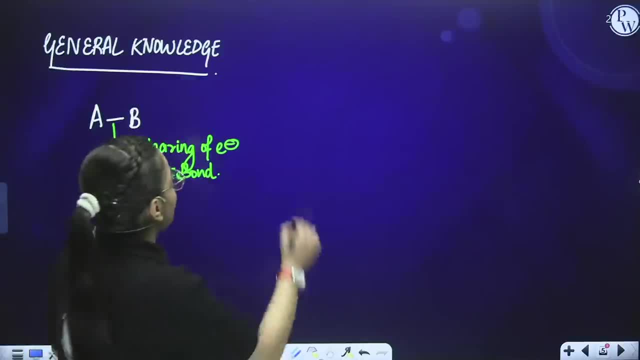 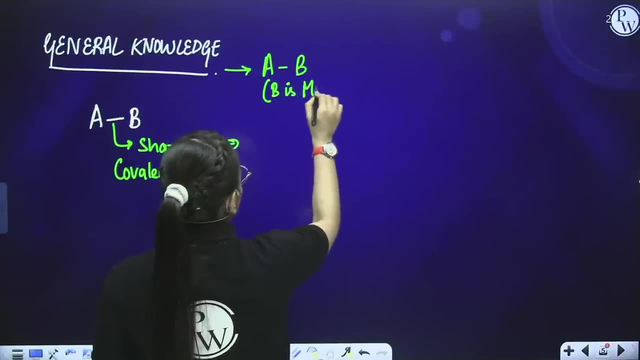 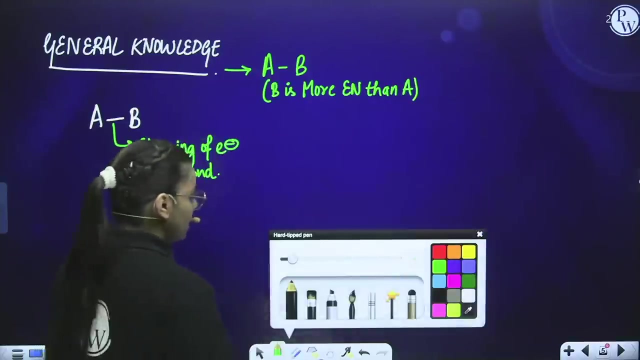 and b is the more electronegative atom. so what would you say if i say in this: a, b, b is more electronegative than a. so what kind of thing that you observe over here? you will say that, ma'am, if b is more electronegative than a, then that means that b has more tendency to attract electrons. 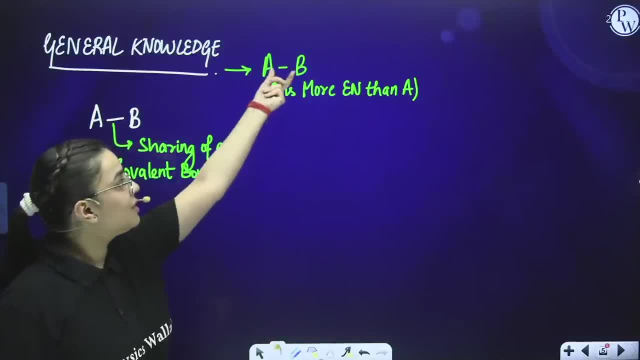 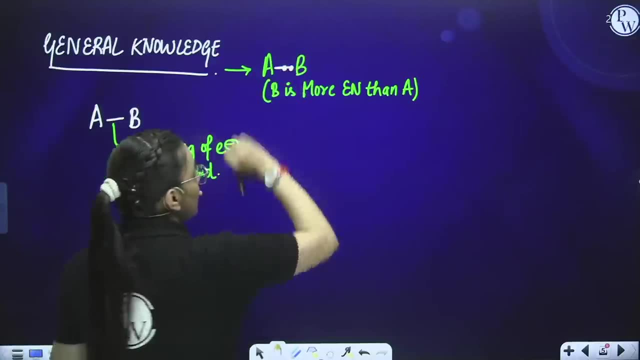 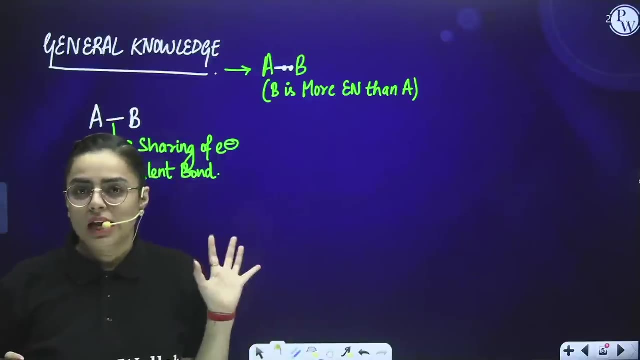 the electrons, the shared pair of electrons. now there there is a bond that contains two electrons. now what will happen? there will be a shift of electrons towards b. towards b. it is sharing with a. no doubt it is sharing with a, but there is a kind of pull towards b. why there is a pull towards? 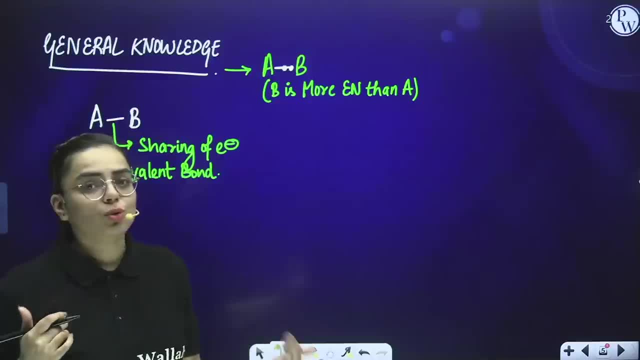 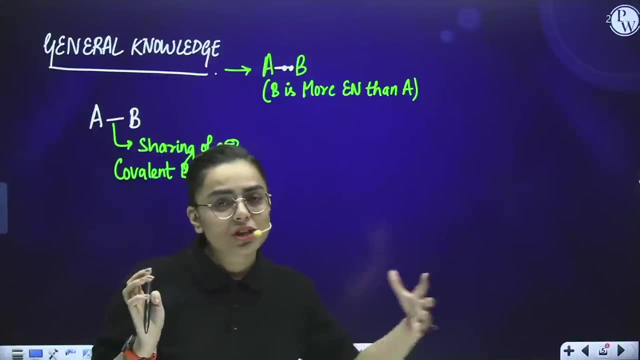 b because b is more electronegative. due to the electronegativity tendency, it will attract the electron towards itself. it will not break the bond and separate, no no, it will just attract, it will just pull the electron towards. so we can see a bit of shift of this electron towards b. first it was 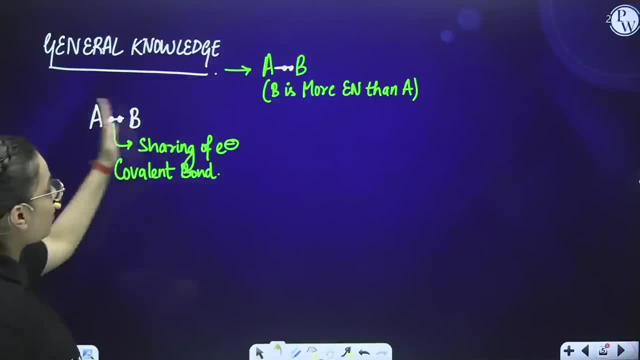 seen that electrons are present in such a situation, but now it is shifted towards this. now when, when you are, you know when electrons are approaching towards you, you will attain which charge. you will attain negative charge, and when electrons are moving apart from you, which kind of charge. 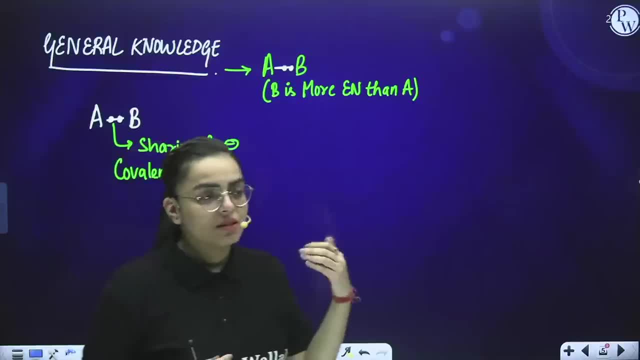 do you develop positive charge? you know that no, when there is a deficiency of electron, positive charge arises. but when you know you have electron, you have a particular kind of electron, then you uh gain, which charge negative. so here b you know, has a shift of electron towards itself, so it will acquire partial negative charge, while 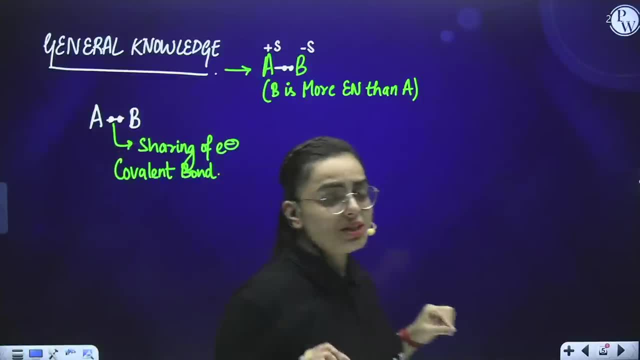 a will acquire partial positive charge. now, this is the basic thing that i want you people to understand: the charges, this is what this is, the polarization of sigma electron here. what is happening here? what is happening here is polarization. here is polarization of sigma electrons. why i said sigma electrons? because it is a sigma bond, it is a 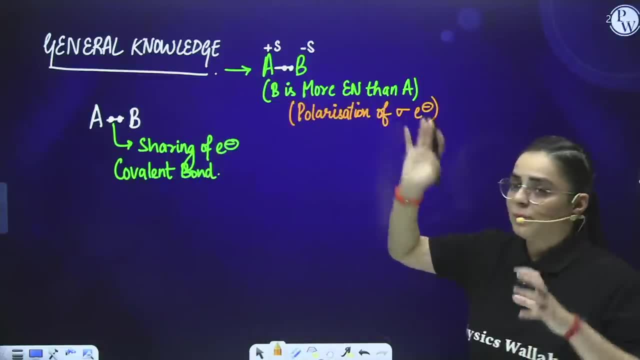 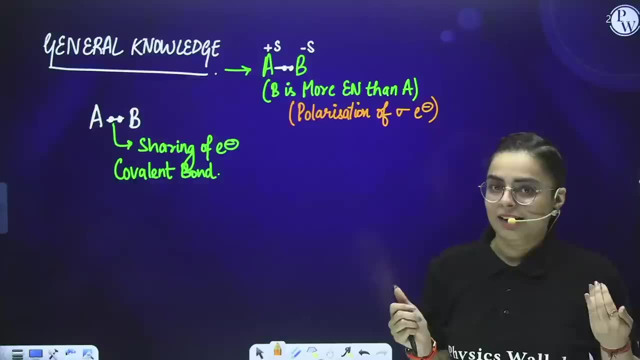 single bond. right now electrons are polarized. that means poles are arising, positive and negative poles are being arise. so here there is a shift of electron towards b a little more than a right. so here bond is not broken, but there is a shift here. what was happening here was a sharing of 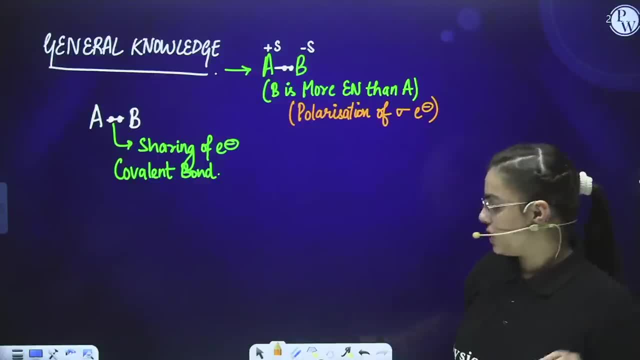 electrons, and that was the covalent bond. now let us take one more example, let us take one more understand, uh, one more concept in depth. if i say, if i say carbon carbon, carbon carbon, and here fluorine is attached. now you, all people should be aware of this thing, that you know, here fluorine is attached. 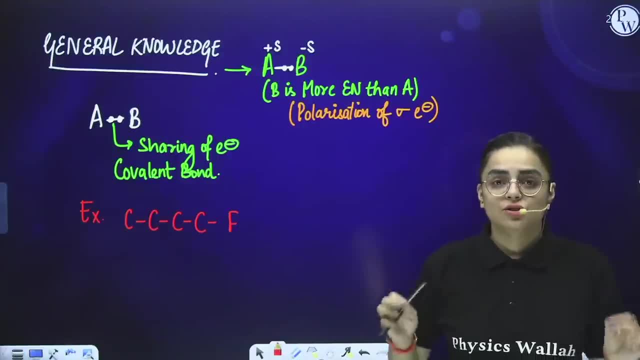 sorry. so fluorine is what? fluorine is more electronegative atom than carbon. this is the basic thing that you need to keep in your mind if you have your inorganic concept a little bit weak. so i am directly telling you that fluorine is more electronegative than carbon. okay, now if fluorine 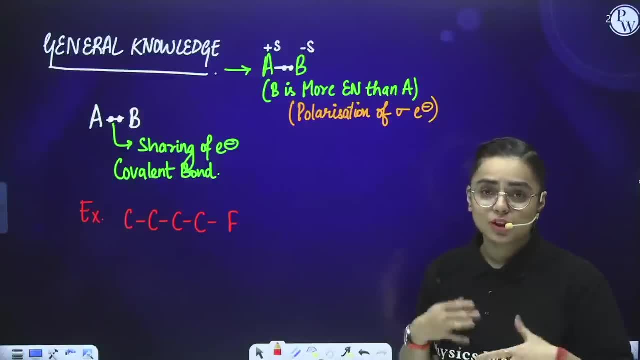 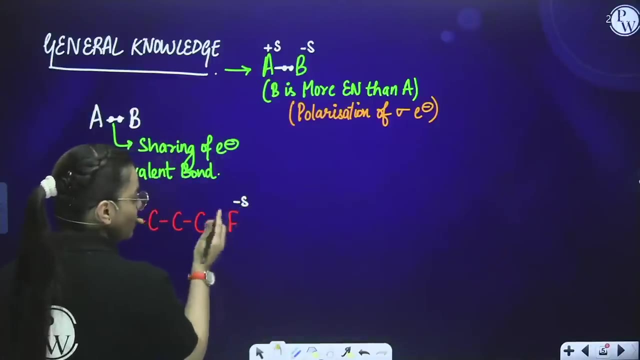 is more electronegative than carbon, then it is going to attract electron towards itself, right, because it has tendency to attract, not to break the bond, just to attract, just to pull, like this b right? so if it has that tendency now here, electrons will be shifted towards this. 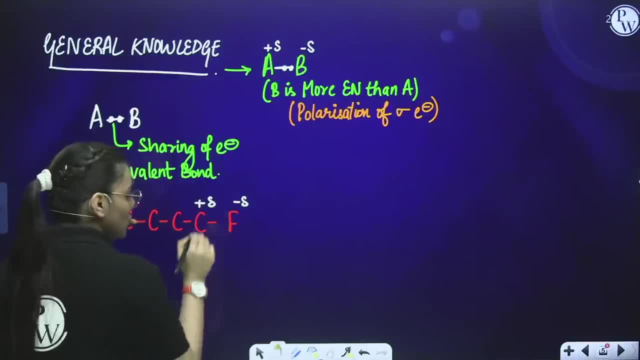 so it will acquire partial negative charge, while this carbon will acquire partial positive charge. so again here in this bond, here over this bond, i would say what is happening: polarization of polarization of sigma electrons, again here, right now. what happens over here, students? what happens over here? there is a little bit pull of electron towards the f right. another thing that you need. 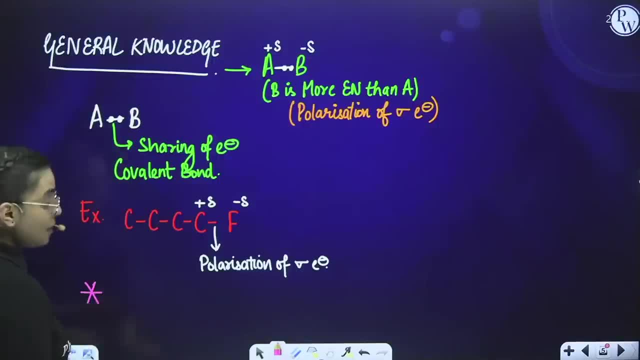 to keep in your mind while solving the question is, sometimes you don't know which is the more electronegative atom, like if we generally talk in the case of carbon. you are given different cases of carbon. then in that case you need to find the hybridization of carbon. you know the percentage. 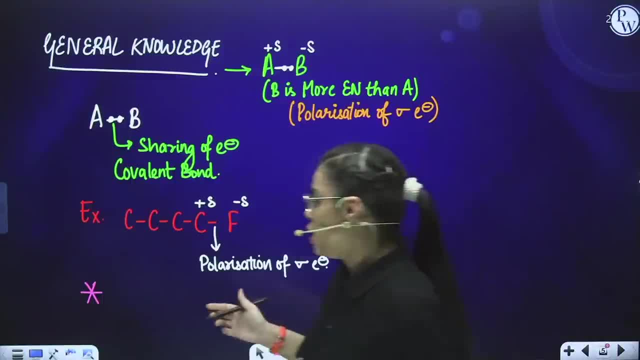 s character is directly proportioned to electronegativity. so, whenever, in the cases of carbon carbon, when you are not given any electronegative atom and you are being confused when there is a double bond or a triple bond, how you can calculate which is more electronegative? 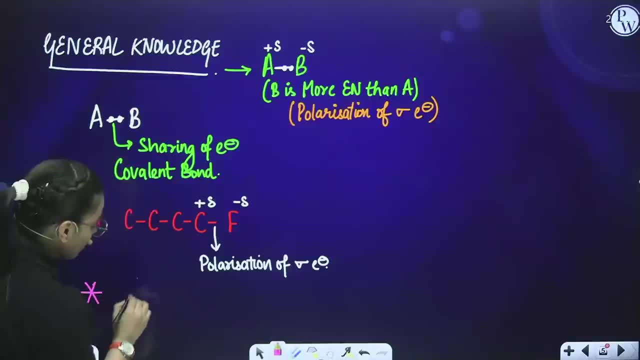 atom, which carbon is more electronegative. so, in that case, what you need to keep in your mind, that percentage s corrector is directly proportional to electronegative negativity. so, in this case, what happens, students, if you keep this point in your mind, if you keep this point in your mind, first of 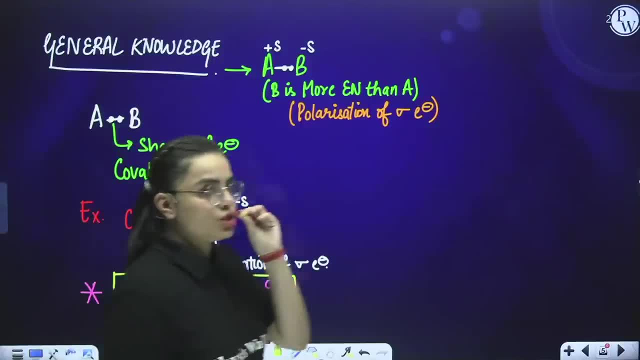 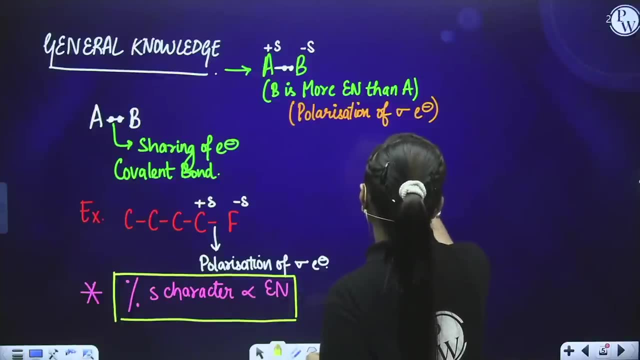 all what you'll do: you'll calculate the hybridization for each carbon atom. you know, when you calculate the hybridization for each carbon atom, you are going to get what you are going to get: sp hybridized, sp2 hybridized, sp3 hybridized carbon atom. right. 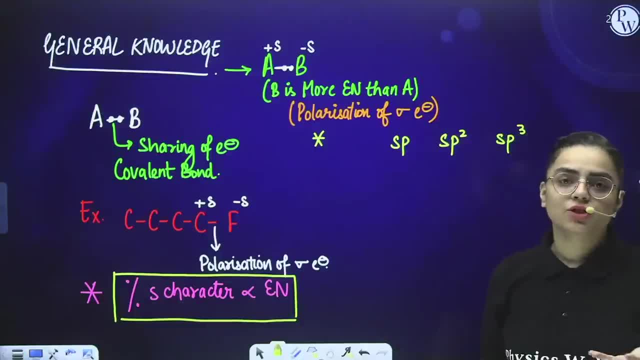 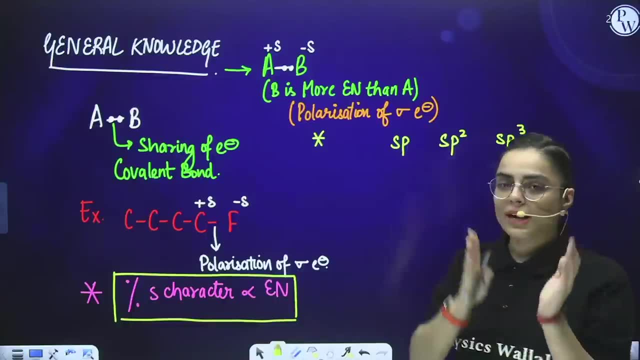 you are going to get this hybridization now, which will have more electronegativity. the question arises: which has more s character now? how to check more s character c? you know there is uh, one s, one p. that means if i divide by 100, that means 50, 50. both the characters are present. if i talk about sp2, 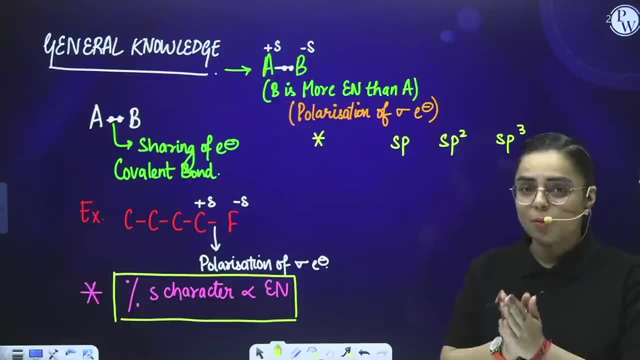 how many s one s how many p? 2p. that means total is the sum of 3. if i divide it again by 100, it is 33.3. that means individually: s is 33.3 percent. one p is 33.3. 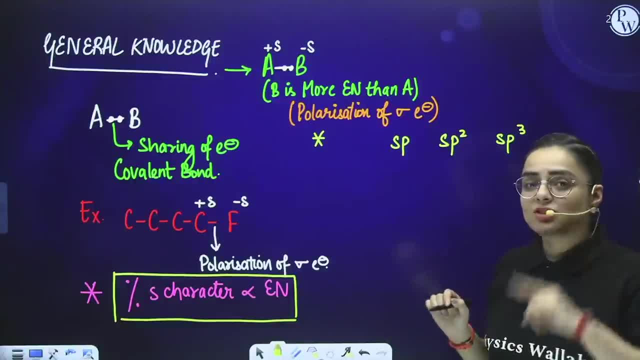 p is also 33.3 percent. if i talk about sp3, what do i observe over here? 1 s and 4, 3 p are present. the sum is 4. now again, i divide by 125 percent, comes that, if i talk here, percentage s corrector. 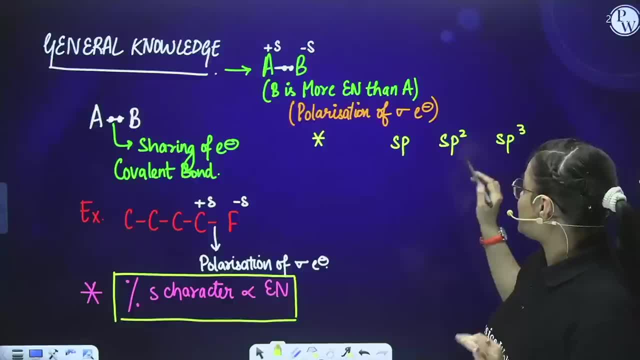 in sp is about 50 percent. if i talk over sp2 here, i would say the percentage s corrector over here is 33.3 percent, while if i talk in the sp3 kind of situation, students, we see 25 percent. so where is s corrector? more in sp, then in sp2, then in sp3. hence, as we know, s corrector is directly. 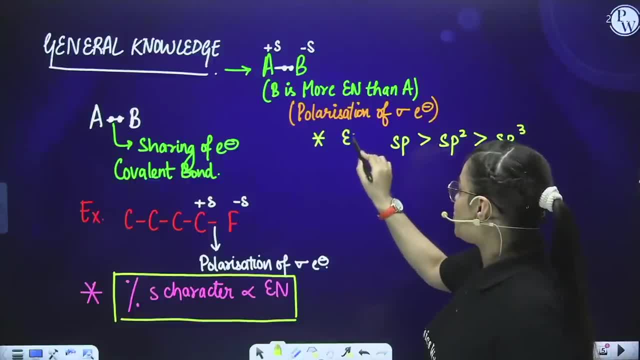 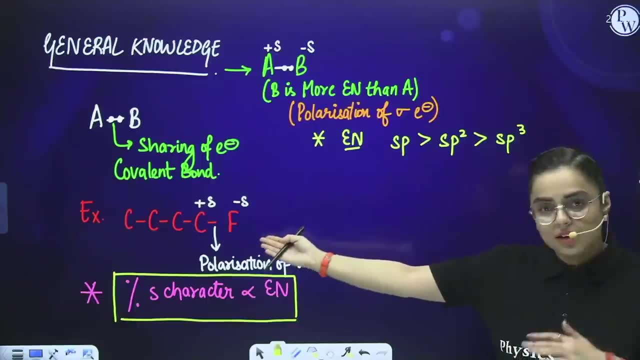 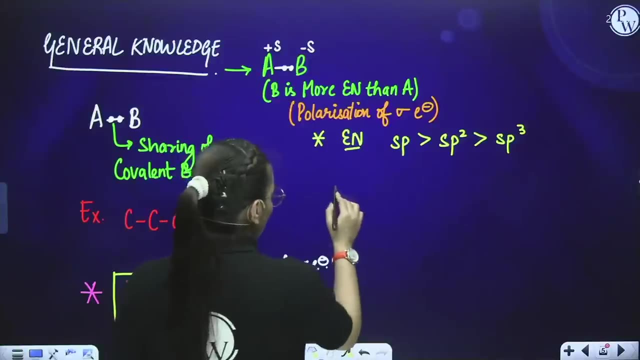 proportional to electronegativity. so the order for electronegativity is going to be this. so it's clear for you. now you are able to identify when it is given like this or when it is not given like this. okay, now one more case. one more case that you are going to observe in the coming. 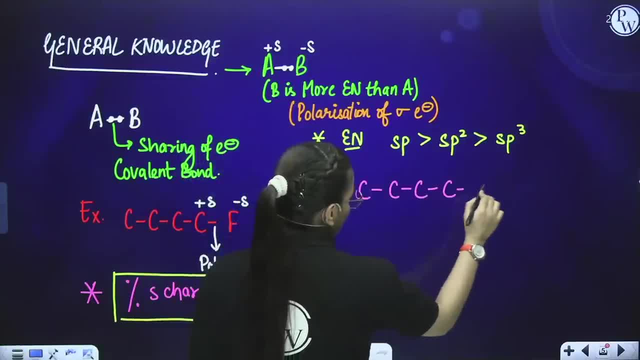 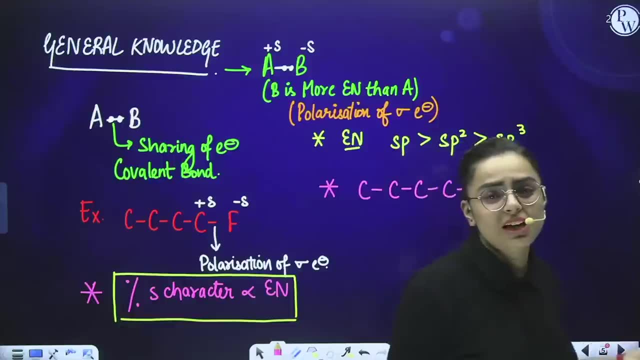 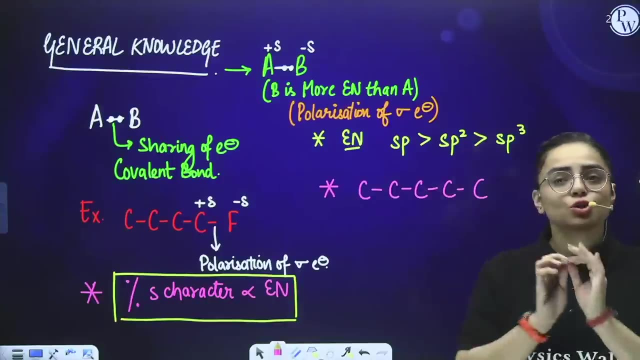 questions is, for example, you are given such a situation now. if i say, kindly, do the polarization of the sigma electrons. will you able to do the polarization of sigma electrons? so answer would be no, ma'am why? because there are same atoms present over here whenever you are having same atoms. so no polarization occurs in carbon, carbon bond. 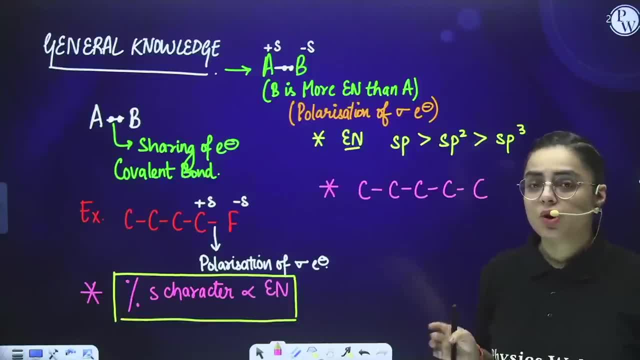 because all are same, all of the hybridization is same. so neither we can follow this concept of more electronegativity, nor we can follow this concept of s corrector, when all the you know, hybridization is equal. so here no polarization occurs. no polarization occurs over same carbon atom, over same carbon atom. clear. 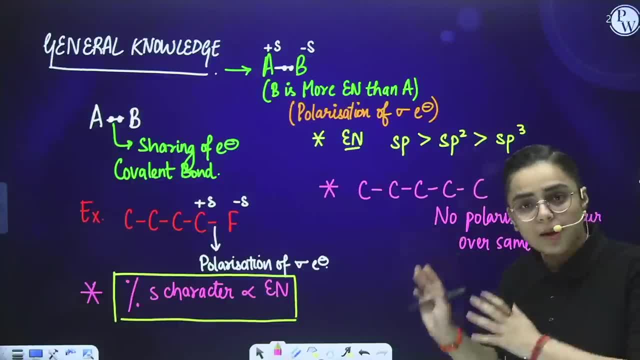 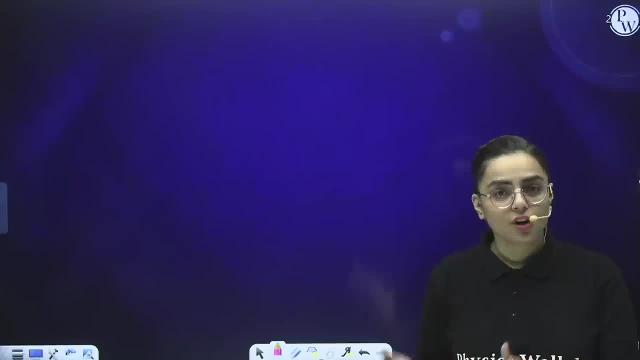 So these are the basic things that you are going to observe in the coming part. okay, Now moving to the coming part. first of all, I want you all to understand an order for electronegativity also that you already know, but let me tell you again: fluorine is the. 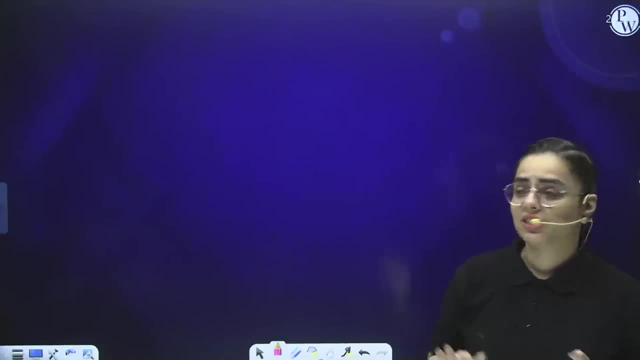 most electronegative atom. then comes oxygen, then comes nitrogen, then comes carbon and then comes hydrogen. this you are going to observe generally. so if you don't remember electronegativity concept, no need to worry. electronegativity is a tendency to attract. 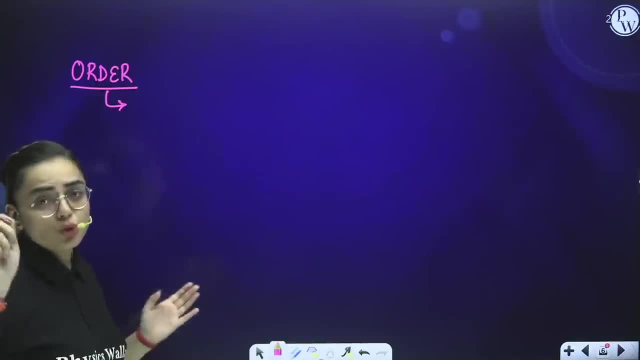 shared pair of electrons and the atoms whose electronegativity you require. I am just writing those: fluorine is more electronegativity negative, then oxygen, then nitrogen, then carbon and then is the hydrogen. So this order, if you remember. 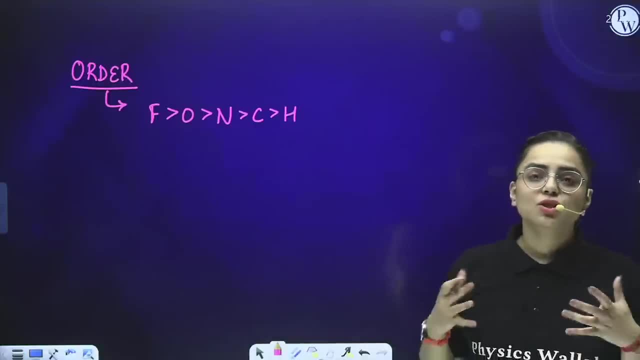 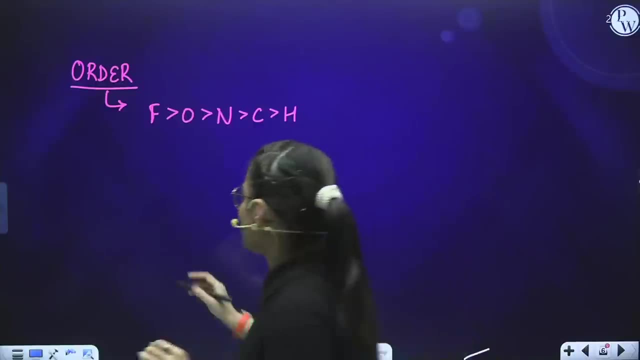 The questions are going to be easy for you people other than this, students. if I talk about, you know three cases. if I talk about three cases, the first case I would say is A negative. the first case I would say again the order for electronegativity, or I would 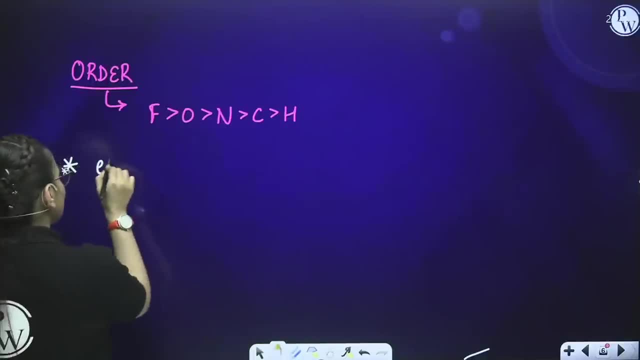 say, let us not say for electronegativity, let us say for electron density. where is electron density? more, If I say, kindly find out the order for the electron density. so what happens is I take a case of A negative. Okay, 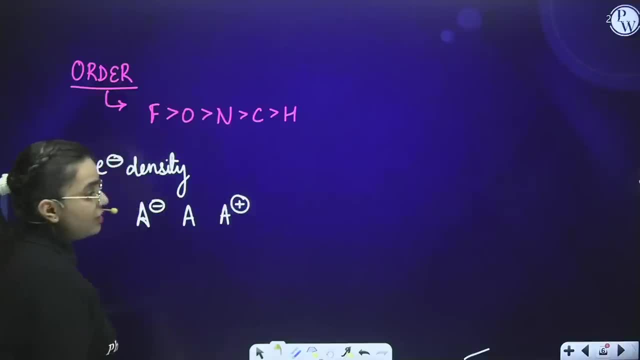 Then is A and then is A positive. Okay, As I have already told you, the one which is gaining electrons carries a negative charge. the one which is losing electrons is carrying a positive charge. so if I ask you, whosoever is having electron density, more kindly tell me, so you will say, ma'am, the person which 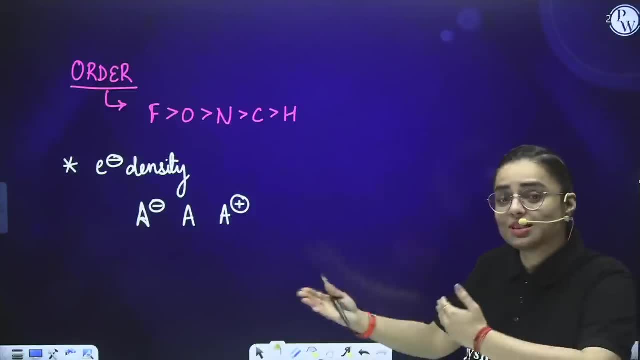 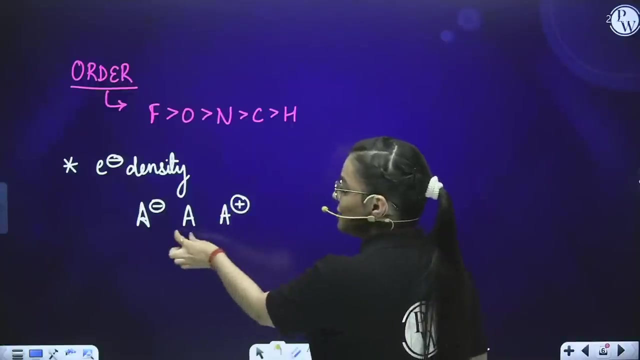 is gaining negative charge will have more electrons because it is gaining electrons. so it is acquiring negative charge and the atom which is losing electron basically acquires what charge Positive, So it is getting moved far away from that atom. That means here electron density is very less. this is neutral. this is neutral and this. 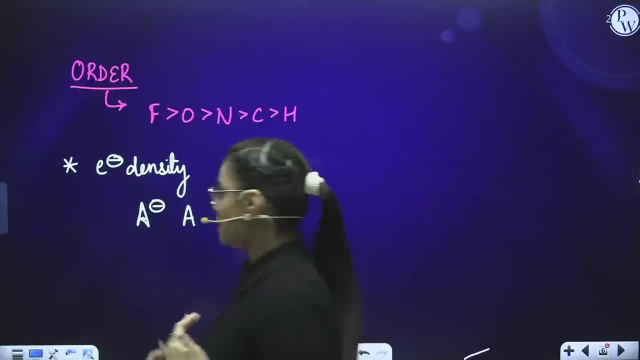 one is the case in which electron density is more, because it is gaining electrons. So the electron density order is going to be this Now. this will also help you in the coming part. So this is all about. you know the general concept that you need to keep in your mind. 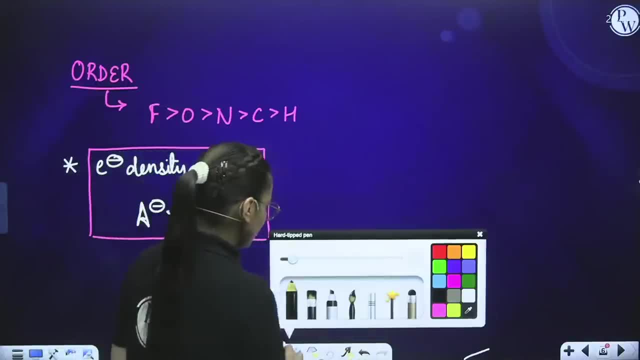 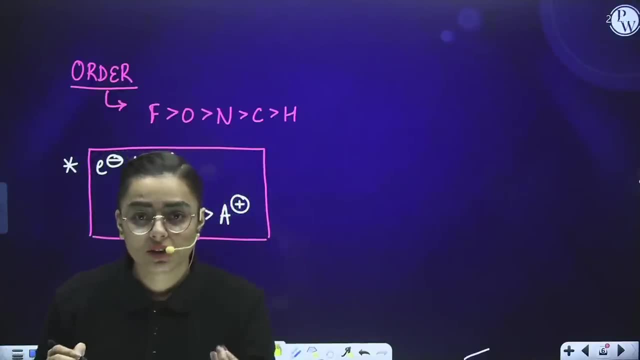 Other than this, as you have seen, I have already done one case of the polarization of sigma electrons. I have taught people to you: know, put arrows, learn to put arrows. in which direction? Now see over here I am taking this case again: carbon, carbon, carbon, carbon, carbon and 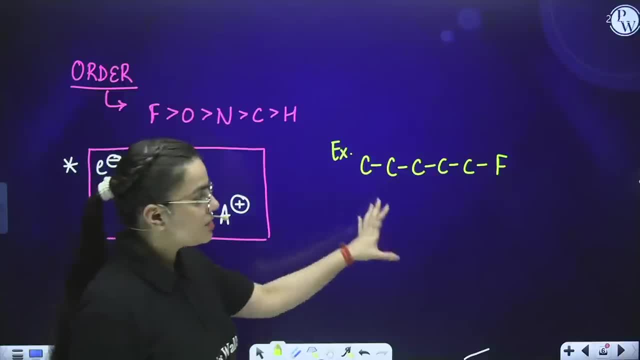 fluorine. I have this case with me, right? This was the single case. but now what different I am going to do over here is I am going to add two more fluorine atoms over here. Now, kindly, you know, first of all, put the charges over here. secondly, try to put the arrows. 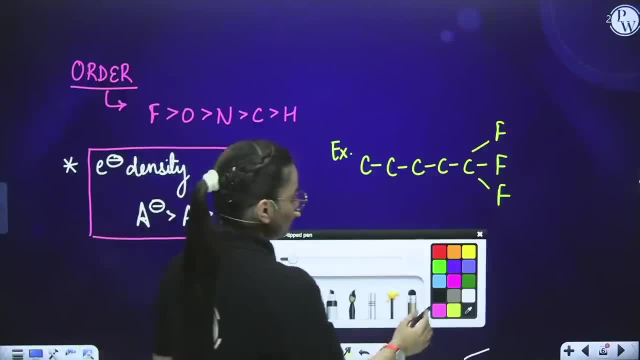 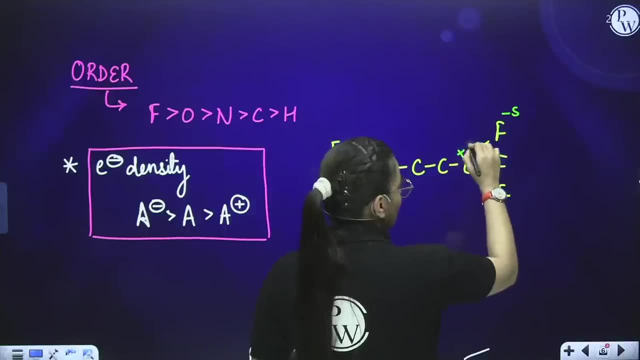 Now, if you want to put the arrows, put the arrows Now. if I want you to put charges over here, what you will do is you will say: ma'am, fluorine is more electronegative, so it will acquire partial negative charge and carbon will acquire. 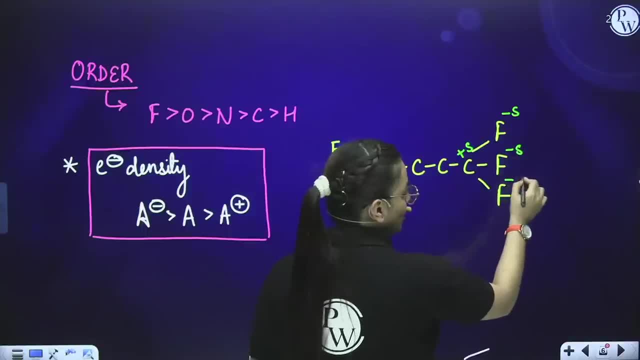 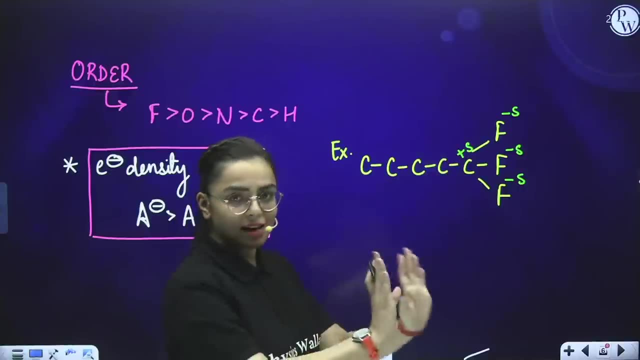 partial positive charge. Fluorine is more electronegative, so partial negative, partial negative. right Now, what happens over here, students? if fluorine is more electronegative, it is attracting electron towards itself. So the arrow will be in this direction: towards fluorine. learn to use arrow, it is going. 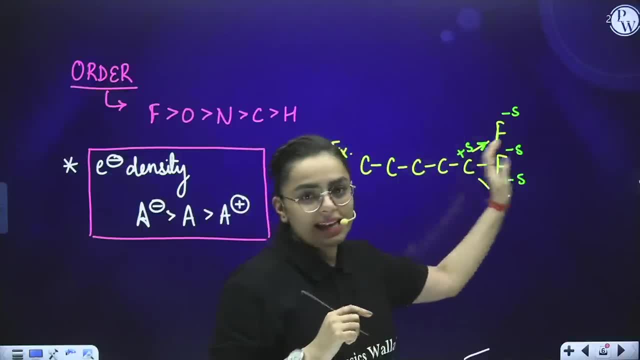 to help you a lot. okay, It is, you know, gaining or out, Gaining or a pull of electrons is moving towards fluorine, so the arrow is moving towards fluorine. Now, in this case also, an arrow is moving in this direction, towards fluorine. an arrow. 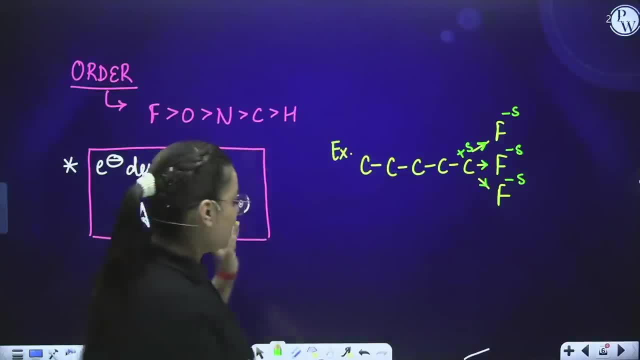 is moving in this direction, towards fluorine. Now, what happens over here, now, when there is a group of fluorine atoms? when I have kept over here, what do I observe? This? carbon is now electron deficient and, due to three fluorine atoms, it is feeling. 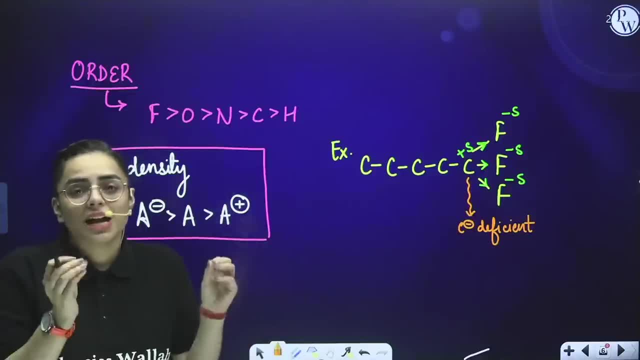 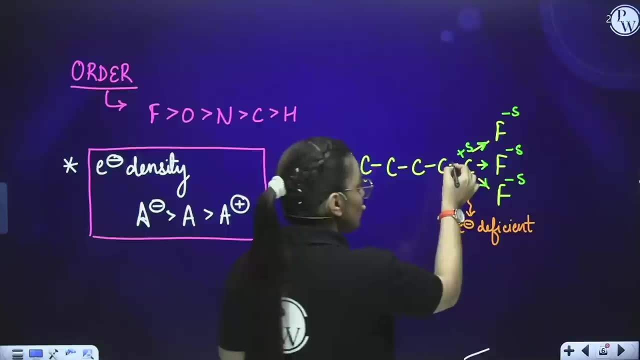 more electron deficient, So it requires some kind of electron, Okay, To stable itself. what does it do? It will take some electrons from the next carbon which is attached to it, So it will take some electrons from here and hence when it is giving electrons to this. 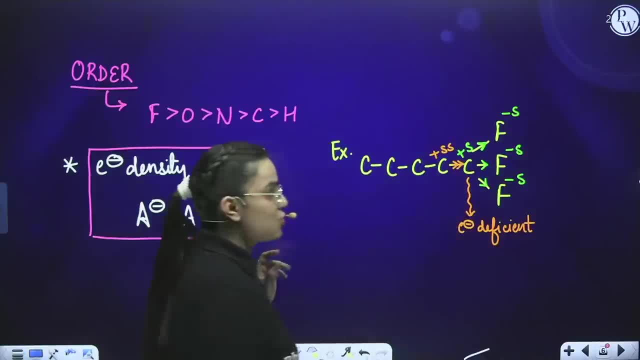 it will acquire. what partial, double partial charge. Now, why does double partial charge occur? because the first carbon, first carbon, was making a bond with fluorine atom, which was more electronegative. So the electrons from the first carbon are moving towards fluorine. 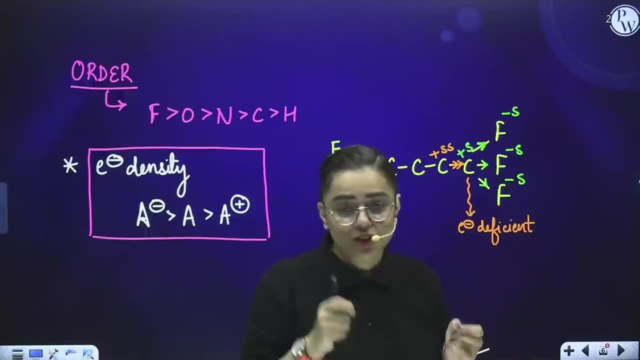 So both of these charges has a partial positive or partial negative charge. But when I talk about the next carbon atoms, then these will acquire double partial charge. Now, if I talk about the third carbon atom, as it has gained some electrons from this carbon, now this carbon is electron deficient- it will acquire what it will acquire: some. 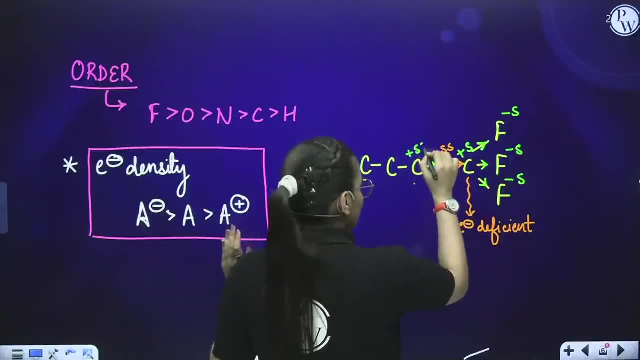 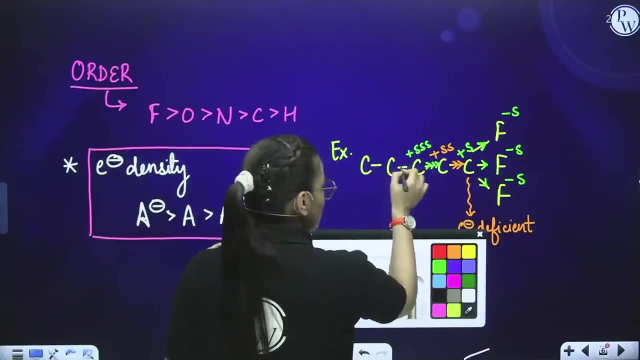 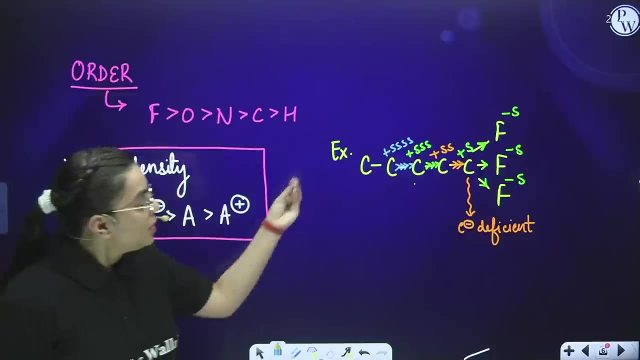 charges from the another one. So it will acquire triple partial charge, positive charge. Now again, this is now electron deficient. it will take more charge over here. it will acquire four times partial positive charge. Now, ma'am, you are taking all the charges to stable another another carbon till when? 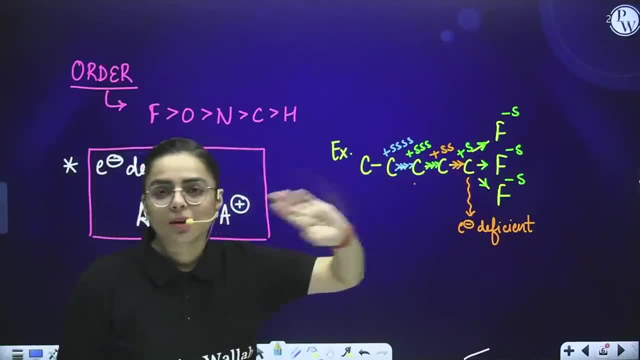 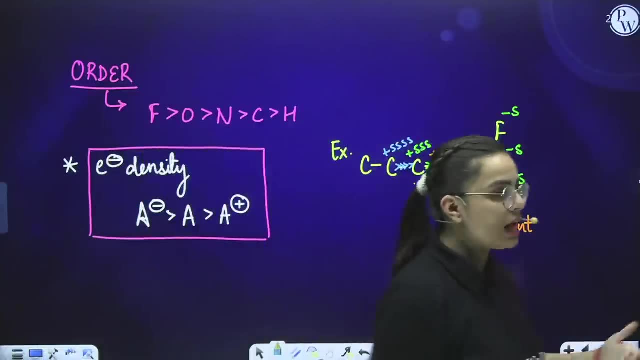 this process will carry on. So it is up to only four carbon atoms, not more than four carbon atoms. this process is carried forward, clear. So you need to keep in your mind, first of all, how to you know make charges, how to develop. 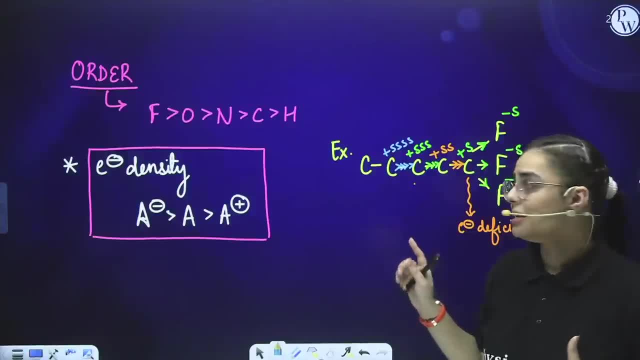 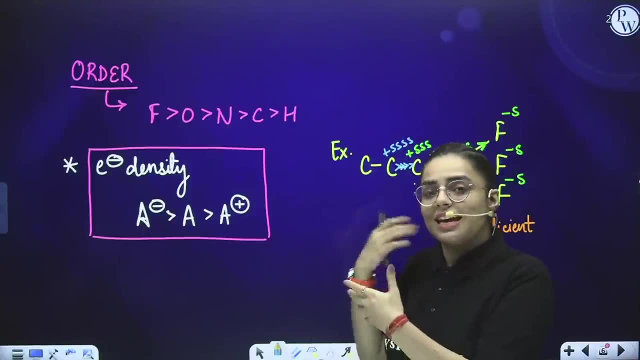 charges over here. another point: you have to keep in your mind that how to use the arrow, in which direction arrow is kept. whosoever has more electronegative or whosoever gains electron, the arrow moves in that direction. This was the basic knowledge that we require in the upcoming topics. 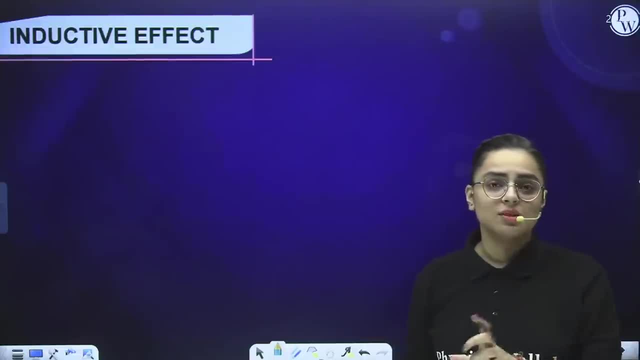 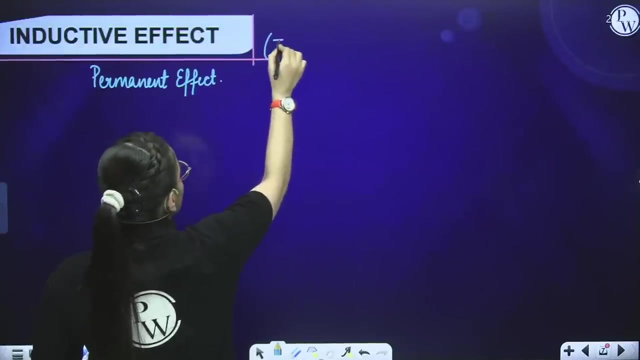 Now, the very first topic that we are going to start in the electronic displacement is inductive effect. As I have already told you, inductive effect basically is a kind of permanent effect. Inductive effect is a kind of permanent effect. it is represented by capital I. it is represented. 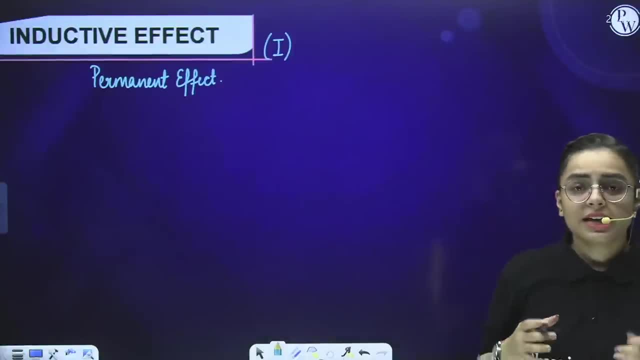 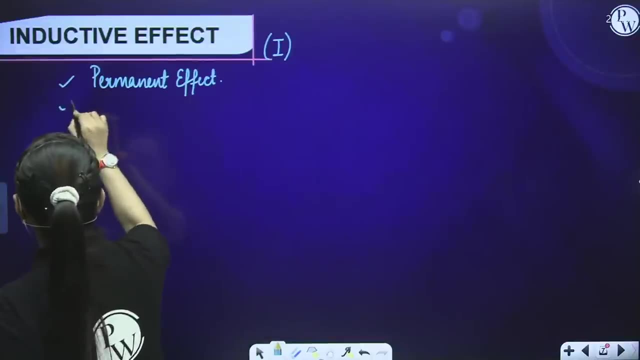 by capital. I Now, what do you mean by inductive effect? Inductive effect: here it is distance dependent. permanent effect: ok, So first of all it is permanent effect. second thing, it is distance dependent. it is distance dependent. that means it depends upon the distance, as we have already seen in the previous. 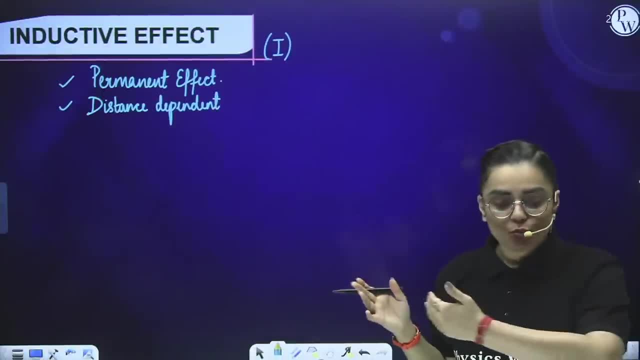 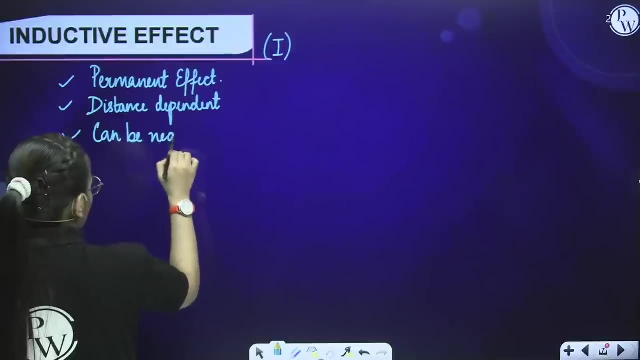 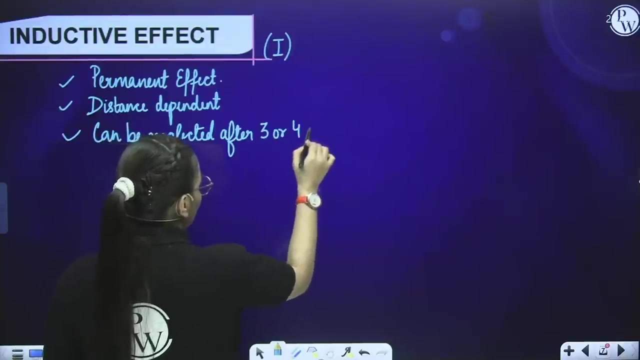 case when there was carbon, carbon and fluorine, it was moving till the fourth carbon atom, right, Ok, now it can be neglected after three or four carbon atoms. after three or four, you can neglect this effect, So it can be neglected, can be neglected after three or four carbon atoms. carbon atoms: 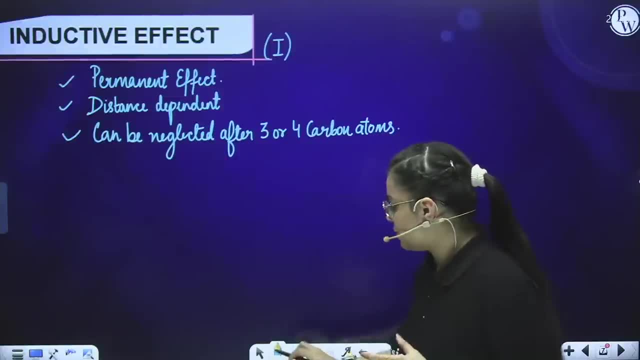 Clear students. Now let us talk about the inductive effect in such a way, which we have already discussed. But to give an example over here, the very first example arises as of carbon carbon, carbon carbon and fluorine, Ok, Fluorine, this we have already discussed. students, 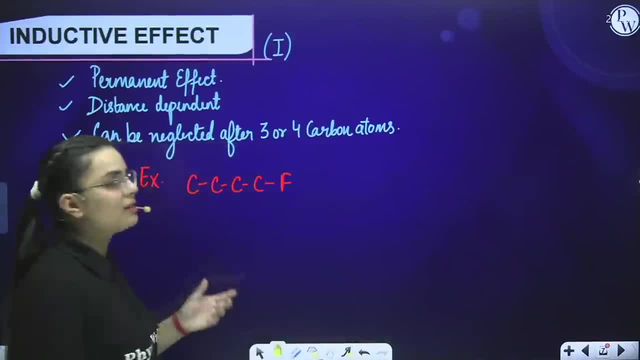 Now my question arises: why does here the polarization of sigma electron takes place? Now, the answer is due to the difference in electronegativity here, here, due to difference in difference in electronegativity, electronegativity, difference in electronegativity. 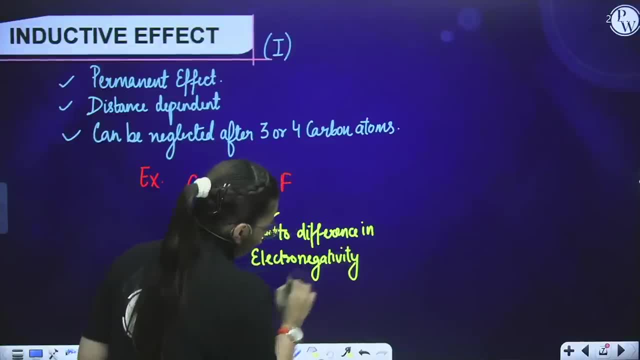 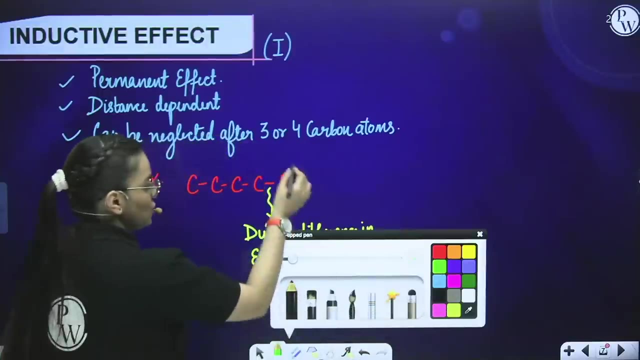 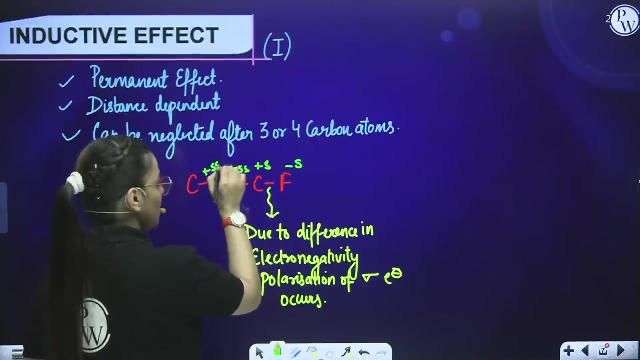 Ok, Polarization of polarization of sigma electrons occurs, due to which they acquire partial positive or partial negative charge. This will acquire partial negative. this will acquire partial positive. This will acquire double partial positive. this will acquire triple partial positive. Now to make arrows. we know that it is giving electrons. you know the pull is towards fluorine. 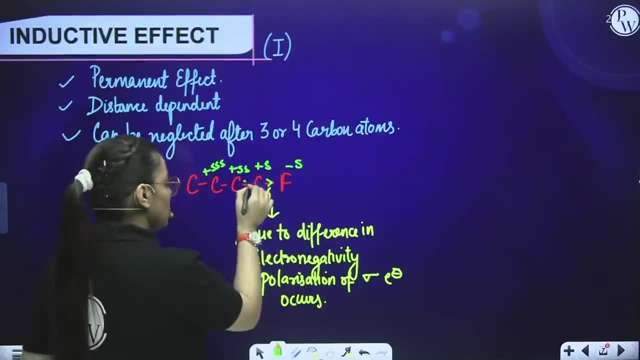 so it is giving electrons. Ok, Now the pull is towards fluorine. now the pull is towards this carbon, because it is electron deficient and it needs electrons. pull is over here, right? So this was the usage of arrow and this is the concept that we are going to use. 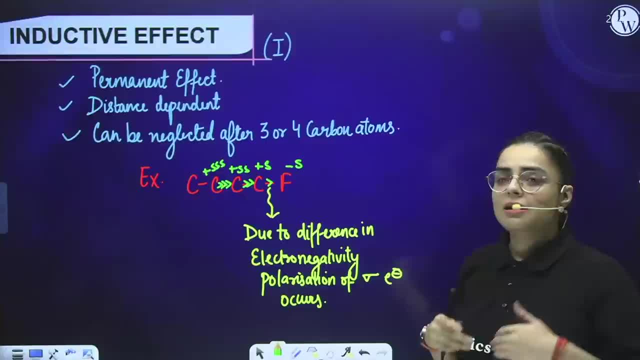 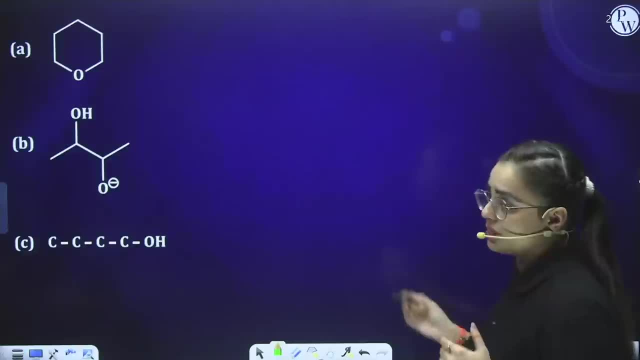 In other words, if I would define inductive effect, all I would say is that here the polarization of electrons, sigma electrons, takes place. clear students. Now, if I talk about this case, I want you all to do what you all to kindly mention. 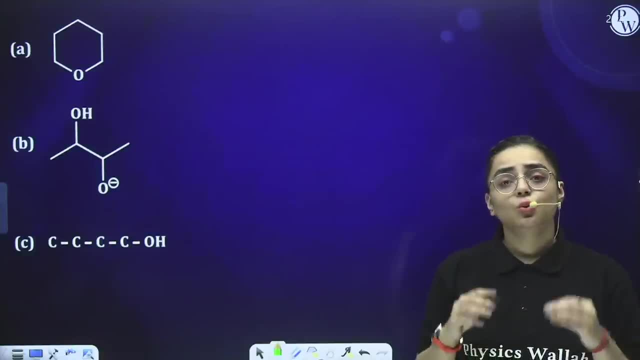 the charges. And the next thing is to kindly mention the arrows. How to use the arrows? I want you all to mention the arrows. Now see, in this case, we know that it is a bond line notation. it contains carbon, carbon, carbon atom all over here, right? 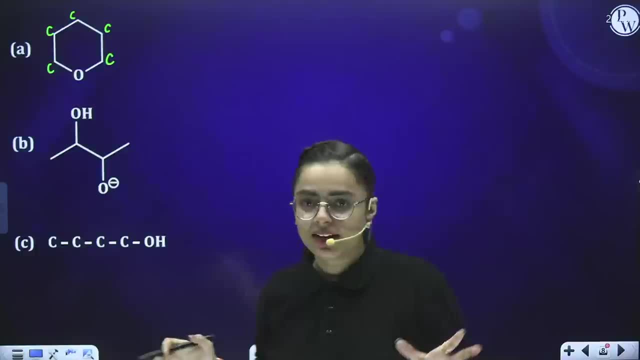 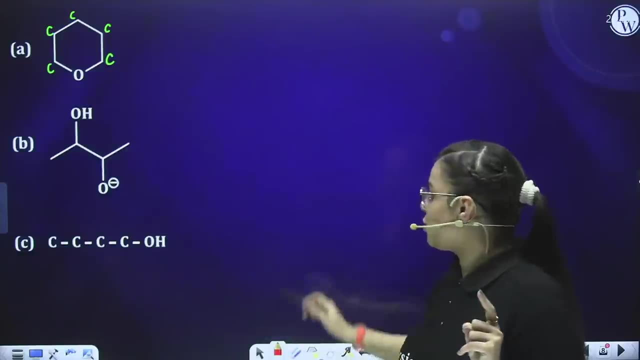 And we have this oxygen atom over here. it is basically hetero atom, right? So we have this oxygen in between these carbon. Now, what happens over here? as I have already told you in the general knowledge which we have discussed over here, the concept of electronegativity- 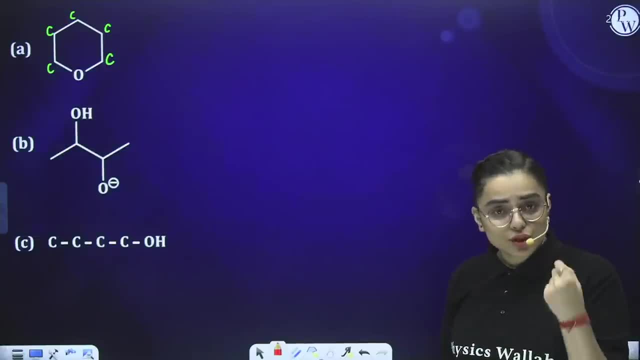 Oxygen is more electronegative. Ok, More electronegative than carbon. If Oxygen is more electronegative than Carbon, then it has a tendency to attract the shared pair of electrons towards itself. Now, if it has the tendency to attract the shared pair of electrons, electrons will move. 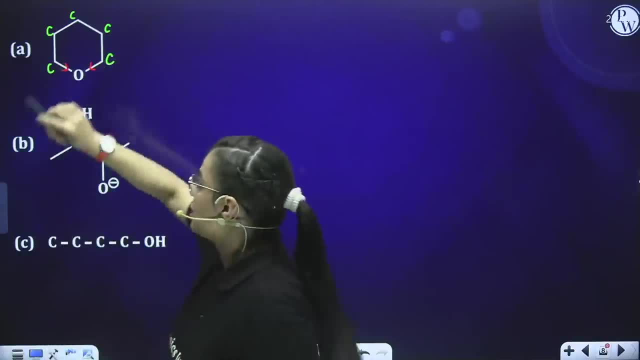 in this direction. it will move in this direction. Now this first carbon. both of these carbons are electron deficient, so they want electrons to be stable. Now they will gain some electrons from this carbon. now the arrow will move in this direction. 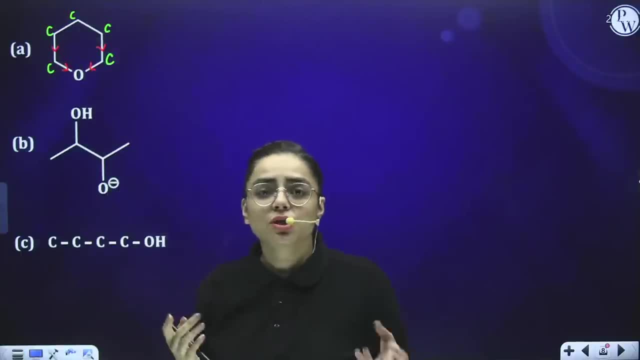 Now what happens? these two second carbons are now electron deficient. they want more electrons to be attracted towards them, to be to become stable. now the electrons will move in this direction, you know. so this is what. this is the usage of farad that you need to understand over. 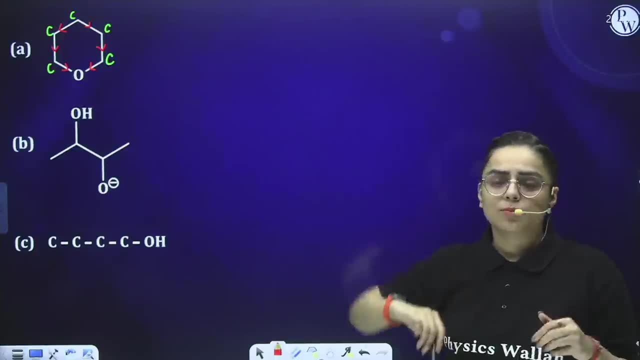 here now what happens over here here? minus i effect comes now what i am talking about. minus i man, we don't know about this concept. what is minus i? till now, we have just studied what is inductive effect. now, a certain term i want you all to understand is that inductive effect is further. 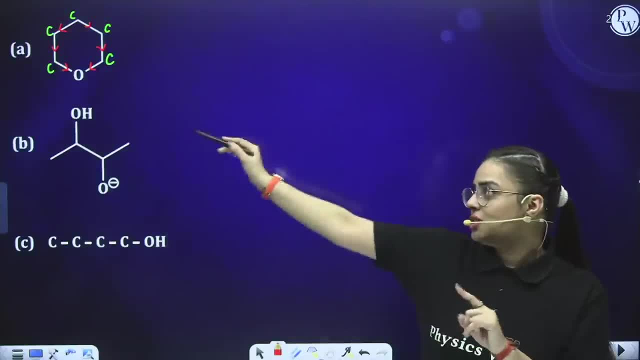 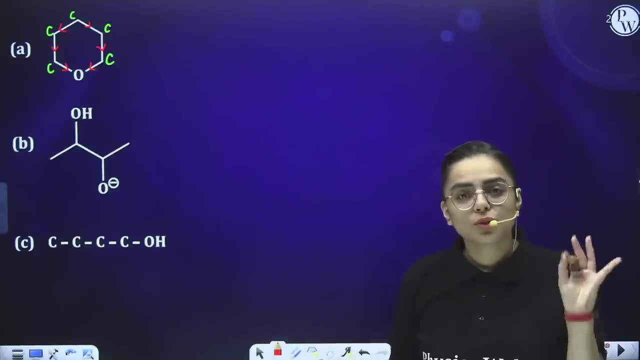 categorised into two types, which we are going to see. it's just i am going to tell you with the help of examples here. just i want you people to make arrows. if you learn how to use arrows, how to make charges, then it is easy for you. now let us make charge over here. if i say it acquires electrons, 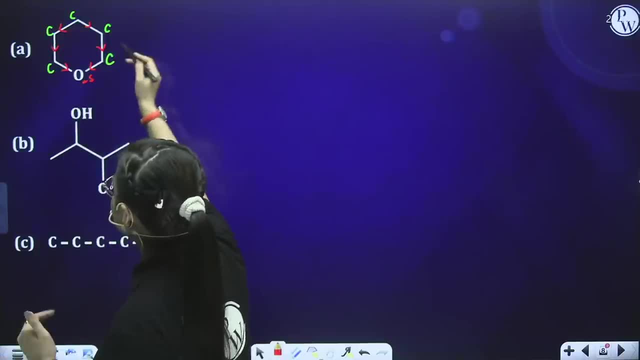 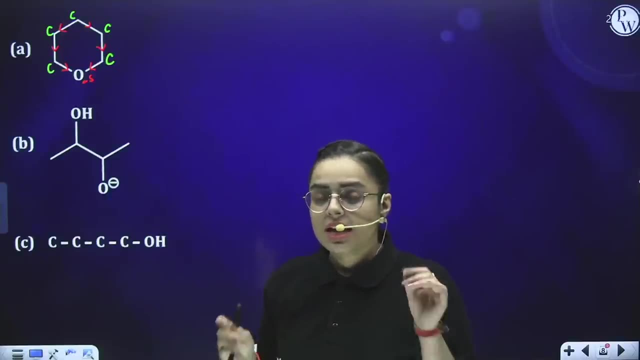 it is a partial negative charge rises over here and this carbon, you know it, it basically you know- get apart from the electron. there is a distance between the electrons. now it will acquire what it will acquire: partial positive charge. this is the first carbon, so this will also acquire partial positive. 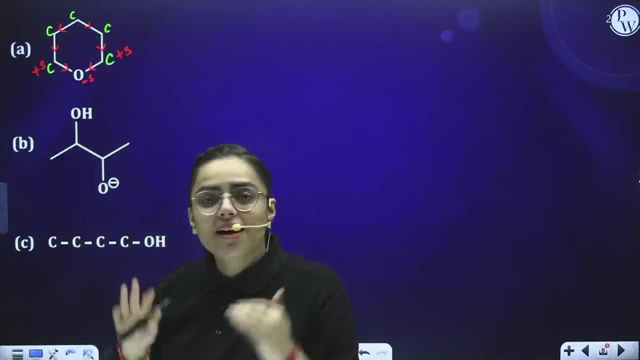 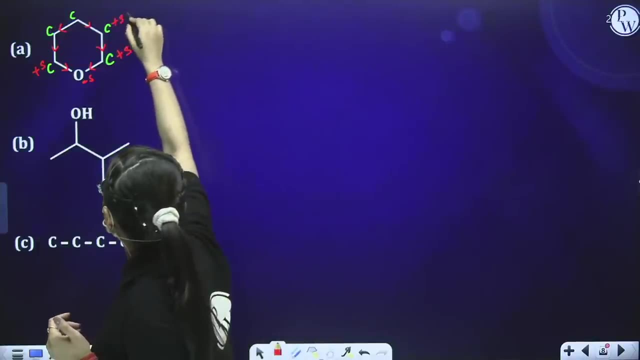 charge. if i talk about the second carbon atoms, now these are again giving you know they are aparting from the electrons, because the first carbon atom needs electrons. so here it will acquire double partial positive charge. it will acquire double partial positive charge. clear now, here, if i talk in this case, it is a kind of a different concept, if you see, if 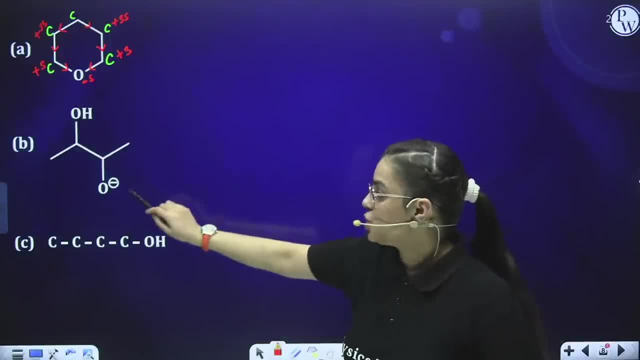 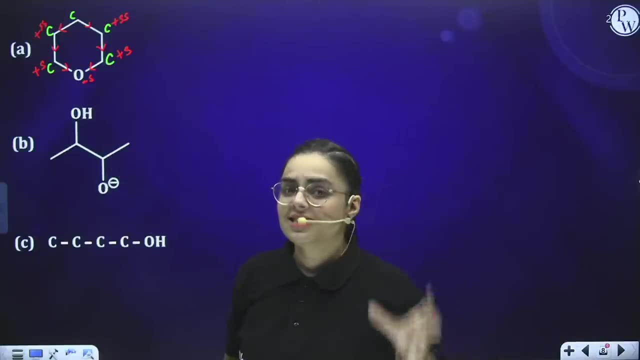 you talk about. oh, here is oxygen, right, but here is o negative. there is a difference between both of these. here is oxygen, and you know that carbon is more. carbon is less electronegative than oxygen. so it if carbon is here, here, here, according to the bond line notation. so i would. 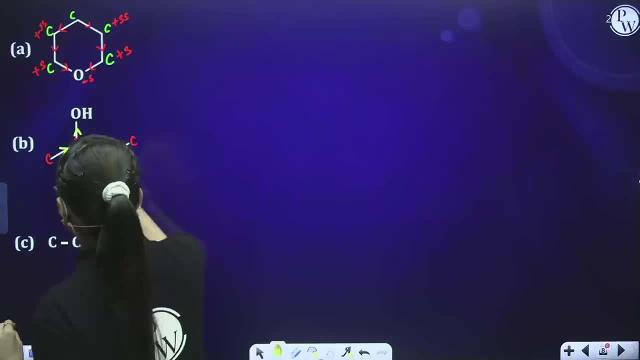 say, carbon is less electronegative, so towards oxygen. the electrons will move like this, like this: this carbon is: there is a shift of electron towards oxygen. now it is electron deficient, so it is gaining electron from both of the ends. now, if i talk about o negative, as i have already, 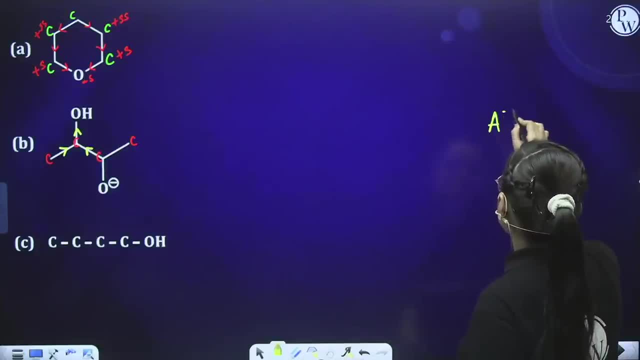 told you in the general knowledge concept that you know, if you talk about the second carbon atom, it will acquire double partial positive charge when you are having a negative a or a positive. in three of these cases, which has more electron density? i have already discussed with you this- will have more electron density. 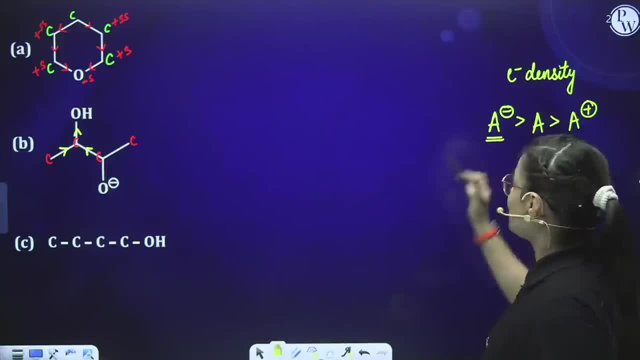 than this, right. so here, what we are observing that a negative, basically, is having more electron density, and if someone is having more electron density, it will donate its electrons. so what happens over here now? this o negative students, this o negative will donate its electron to carbon because it has more electron, you know density. so the direction over here is this the direction. 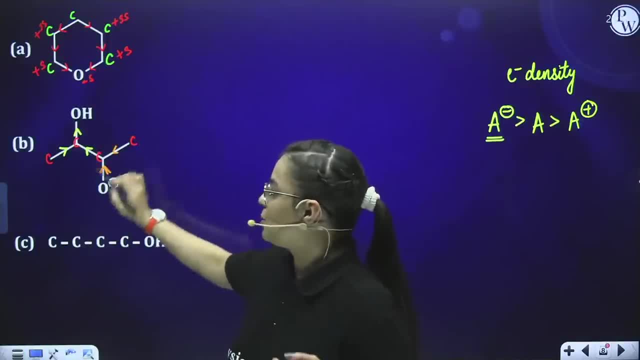 over here is this and over here is this because this carbon is also donating to this carbon. so it is a different kind of thing that you are observing over here. in one is o h, you know, which is having a pull of electron towards here, and one is o negative, which is, you know, giving electrons. 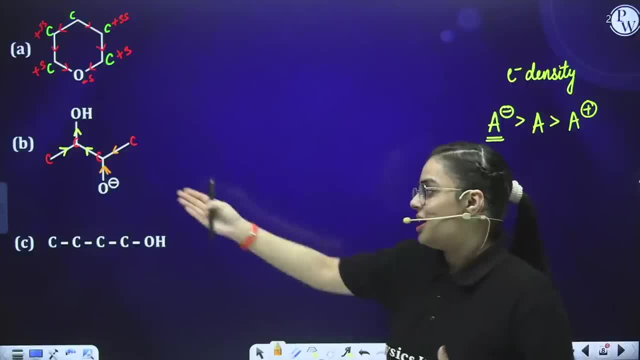 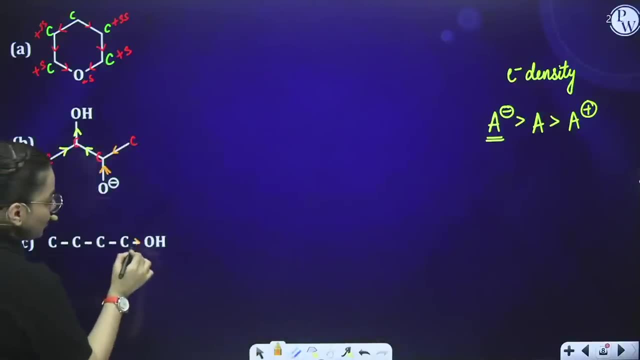 pull towards carbon atom because it is already. it already has more electron density. clear. now let us see this case. here is simple o, h. so i would say carbon is less electronegative than oxygen. so oxygen will have a pull of electron towards itself, will gain partial 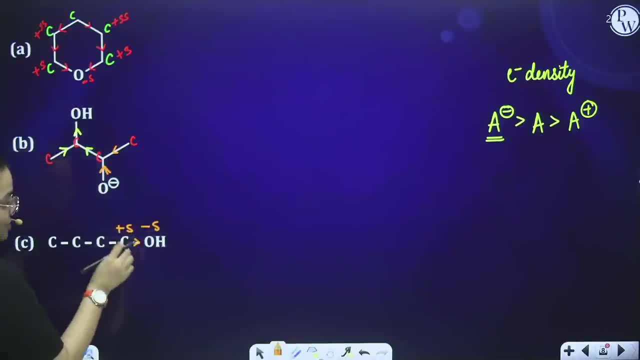 negative charge, this will gain partial positive charge. hence this carbon is now electron deficient, so it will take a pull of electron from the another carbon, so will carry out the double partial positive charge, and the third one will carry triple partial positive charge. so now you are being able to, you know, put the arrows, and which is all required for the 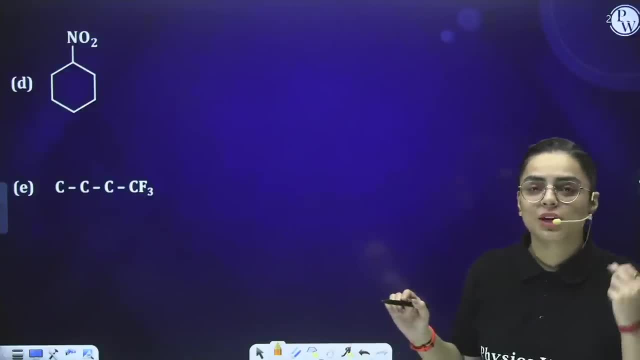 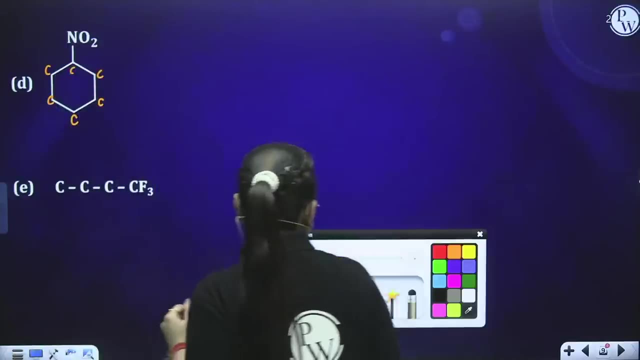 upcoming concept. now comes this case. if i talk about this case, what happens? we know that this is basically the bond line notation here: carbon carbon, carbon, carbon carbon will come right. if i talk in detail, i would say nitrogen is more electronegative than carbon, hence nitrogen. 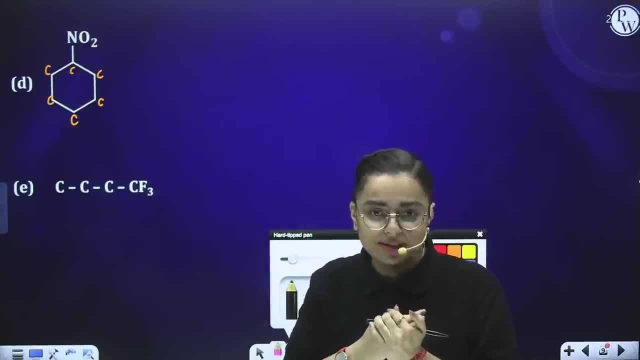 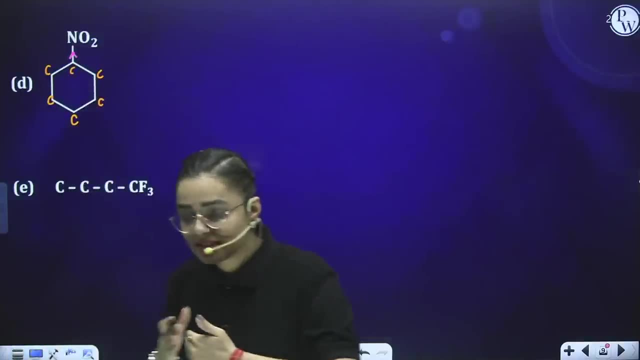 has the tendency to attract the shared pair of electron towards itself. now, if nitrogen has this tendency, this will attract. okay, now this carbon is electron deficient because it has given some part of electrons, because it is a far more distance from the electrons which it was sharing. equally, now it is at a far more distance, so it is electron deficient. 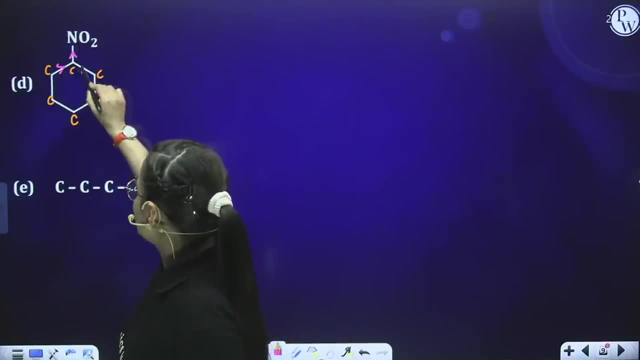 so the kind of happens, which happen, which can be a significant problem in asiatic. y como tenemos electron, so it can be taken as electron y como tenemos electron, such a common problem. but i will show to you how to see it as carbon. once again, this: you have to calculate it in terms of the concentrations. 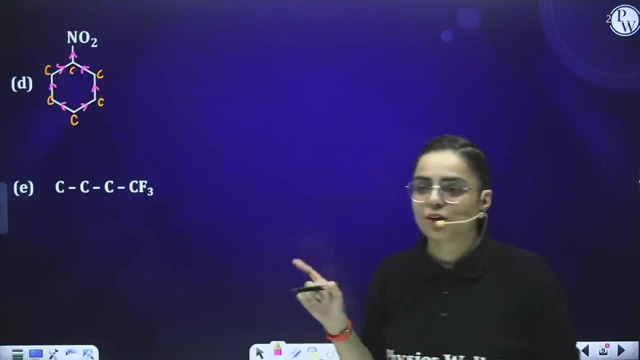 of it can be calculated. if you will look here, there areiği ve tapce of this one. adesso talk about this case. this a par from another carbon, and here in case, 600. so to take look at this, we have already covered this same thing. ok, actually every. 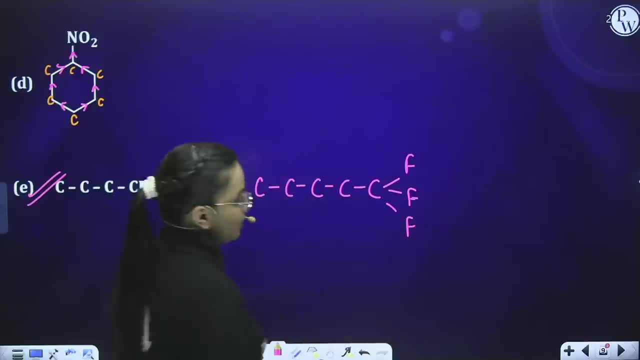 day and you should sign your cards on your hard copy. okay, right Y may be even. see this case. you alway not have to do so again and again. if you have, you would also missed out very little time for this case. see that you see the same Ellen cells as a factor. 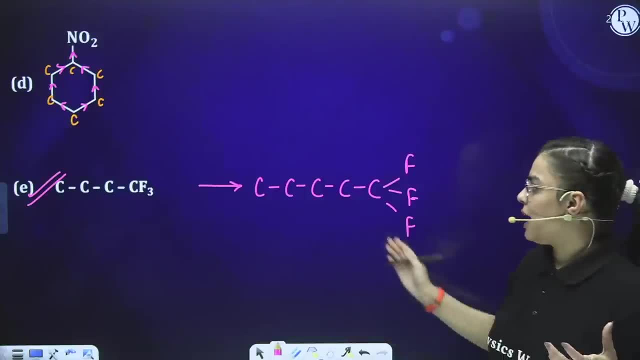 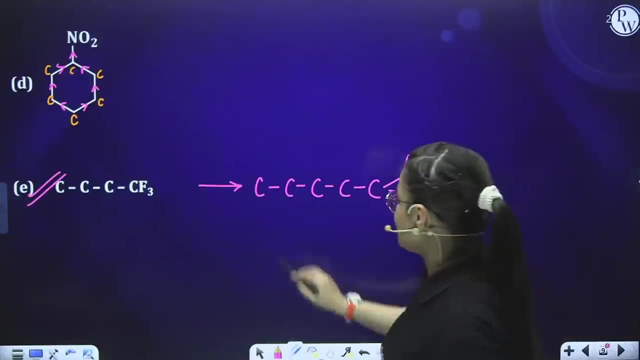 or molecules in this concept. most likely it will not be a coincidence, for this is going, and again because you already know this now, i have used here five carbon atoms. you can use three carbon atoms. it is the same thing, so no need to worry about it. okay, because this concept. 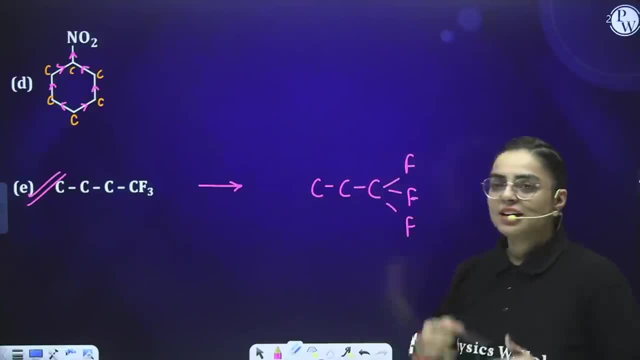 is, you know, is valid up to three carbon atoms. so if you are going to write, uh, four carbon atoms or five carbon atoms, so that doesn't make sense because it will be valid up to only three or four carbon atoms. clear, students. okay, now moving to the types of inductive effect. all i would say 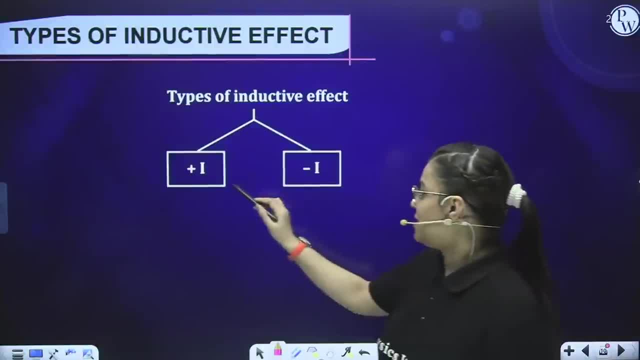 is inductive effect basically is of two types. one is plus i effect. another one is minus i effect. now, what is plus i effect and what is minus i effect? to understand plus sign in minus i, we need to understand the standard concept, through with the help of which we define plus, i and minus. 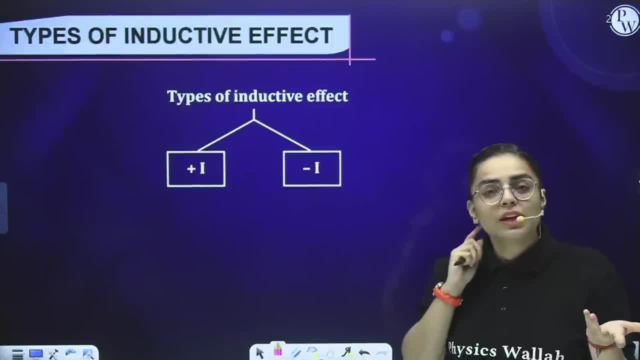 i see what happens whenever you go in market. you know, whenever you go to buy bananas, what do you do? you see there is a standard unit get kept. that is dozen, right, so you know what is a dozen. so there is a standard kept. if you want this much banana, then you. 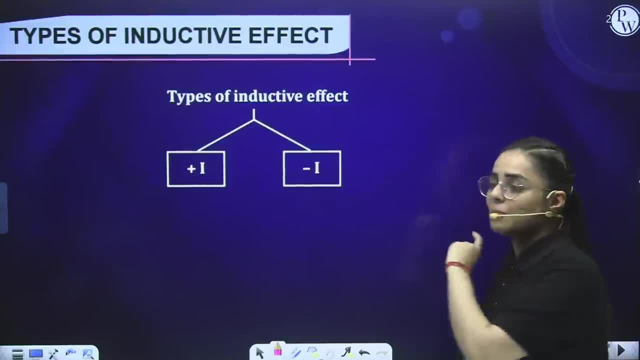 need to measure in the dozens now if i want to measure plus i and minus i effect. what i am going to do, i am going to keep a standard, with the help of which i am going to differentiate or compare the other effects, so that i could be able to define what is plus i effect or what is minus. 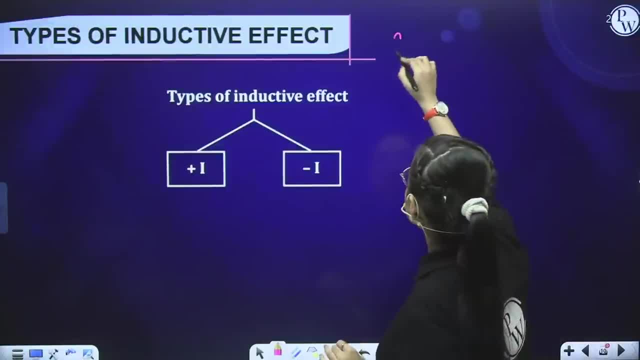 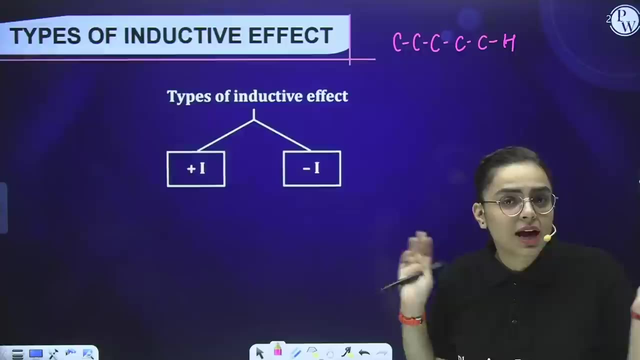 i fix. so the standard that is kept over here is simple: when there is carbon, carbon, carbon, carbon, carbon and hydrogen, so when you observe there is a bond between carbon and hydrogen, here we see that when there is same atom is all carbon atoms, we say there is no polarization of electron. but when we see here that carbon, 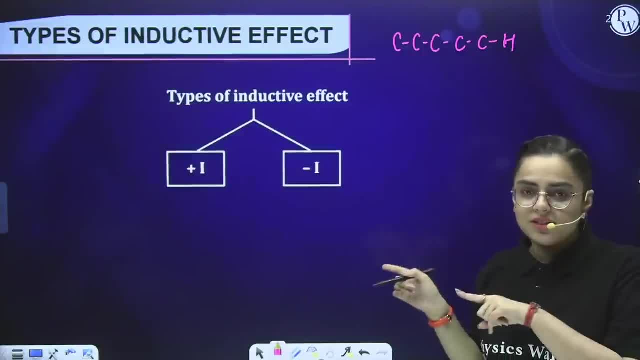 and hydrogen comes. you will say that, ma'am, here we have seen the general knowledge concept. we have seen that hydrogen is less electronegative, so you don't have to apply that concept over here, because here this is considered that it has an inductive effect of zero. that means 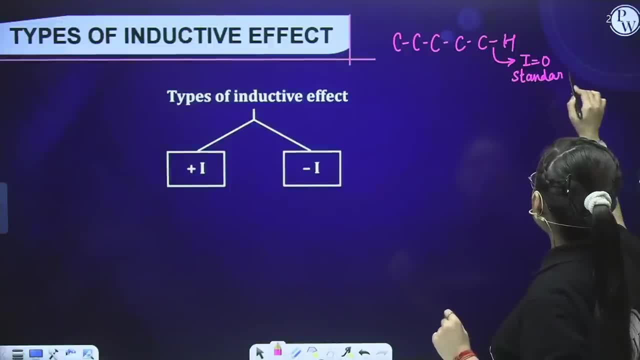 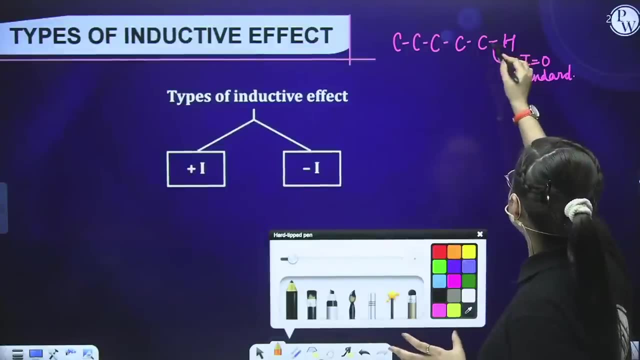 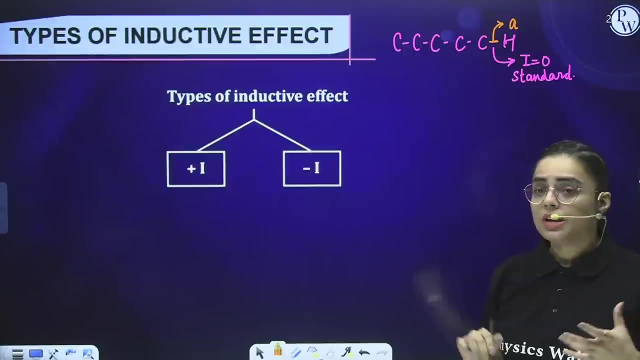 it is kept as in standard. it is kept as a standard over here that here inductive effect is zero and the bond present in between these, these, these sigma pi electrons, are basically a. let us say they are a. let us say they are a. now we are going to compare the with this. 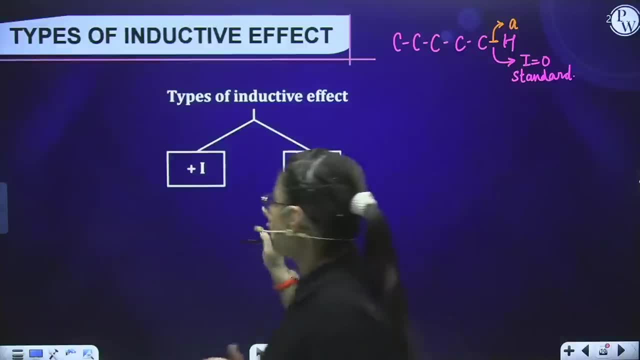 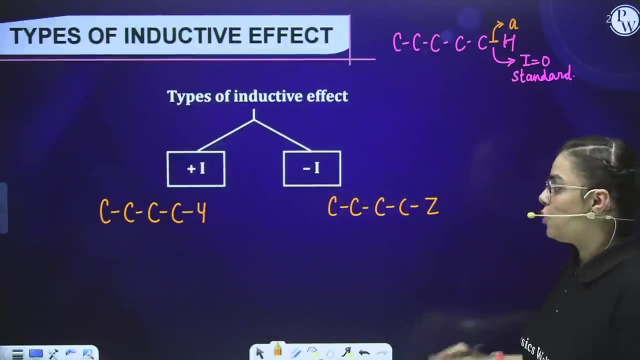 a bond. the other two now. first of all, we are going to see the plus i effect and if i talk about the minus i effect. okay, now what i have used over here. here i used hydrogen, which was kept as a standard. now, for both of these cases to understand, one i have taken is y group, another one i 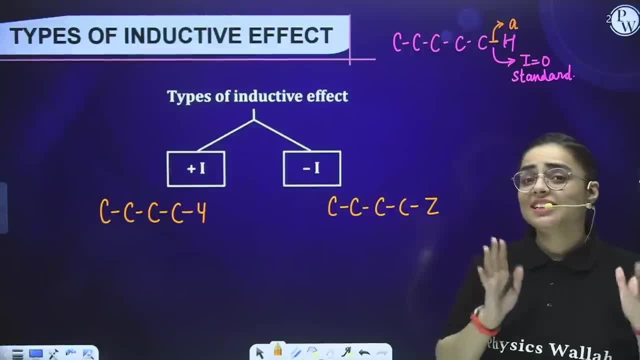 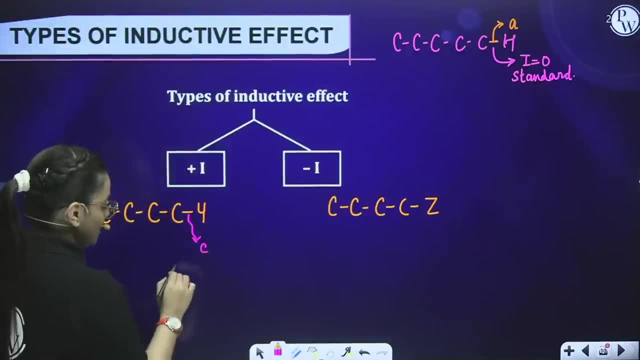 have taken is z group. if i talk that a is basically less than c. now what is c over here? c is this bond, the bond between these two where the electronegativity difference arises. now, as i said, a is less than c, then we observe, plus i effect. now what happens over here there? 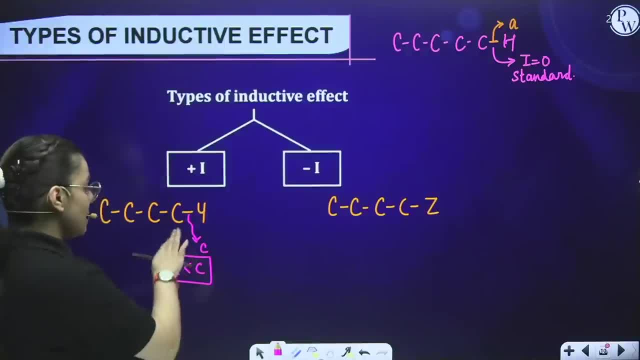 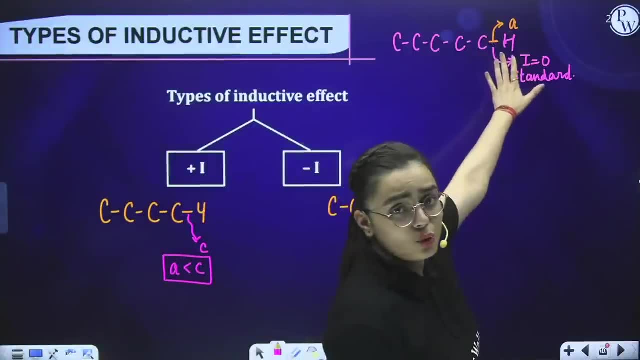 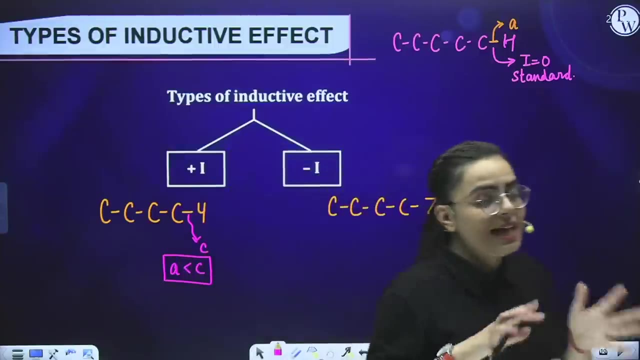 is a electronegativity difference over here. see, this carbon and y has electronegativity difference. this carbon and z has electronegativity difference. we are keeping this as a standard. there is, though, no electronegativity difference here. electronegativity difference arises here. what happens here? when i am saying, a is less. 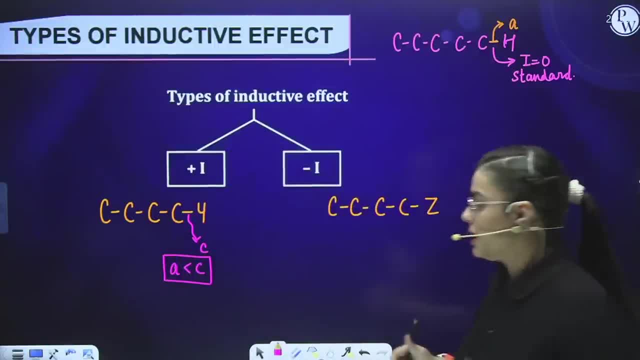 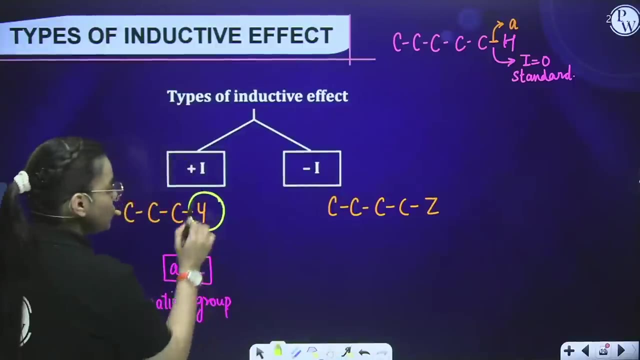 than c. that means it is electron donating group. kindly listen to me very carefully: it is electron donating group. donating group that means this: this y, which you are going to use, will donate electron to your electron cycle of energy. so these are the ones that we are seeing here, fast and easy. thanks, brother. thanks for your time again today. we are interconnected. 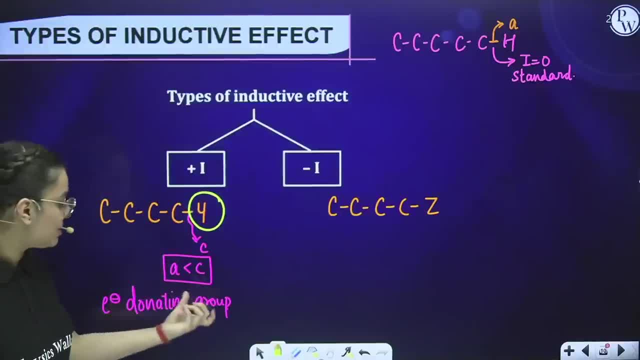 and two. so этоiertlkier a-a-a-sol, draaw métrik through an arc and you will get power. power to these will donate electrons to these. so it is electron donating group. this one is electron donating group. this c is more than this, this a. if it is more than a, that means it has more. 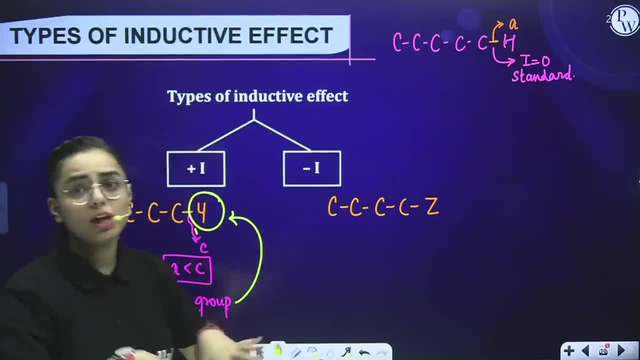 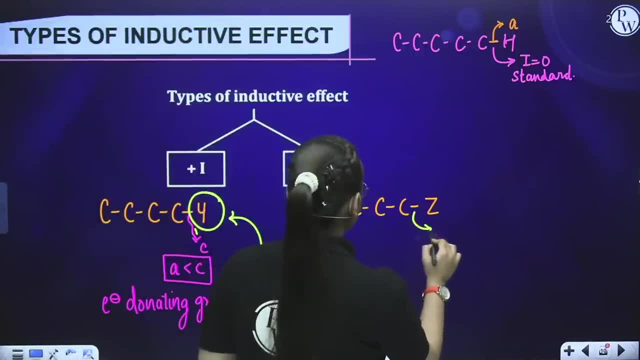 electronegative, it is more electronegative, so it will donate. it will donate, clear. now, if i talk about this case, if i talk about this case, what do you observe over here? let us say there is a bond B here. okay and all. I would say that A is more than B. If A is more than B, what do we? 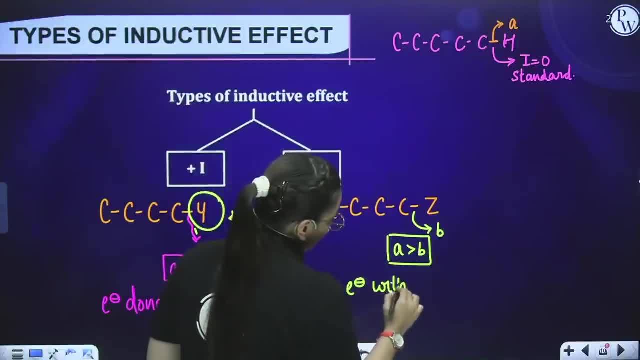 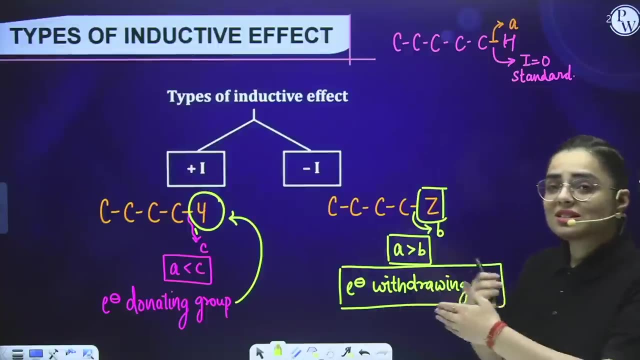 observe over here, It is electron withdrawing group, Electron withdrawing group. Now, what do you mean by electron withdrawing group? Which Withdraws electron, which takes over the electrons? Now this Z will take the electrons from the carbon atoms. Now this Z will take. 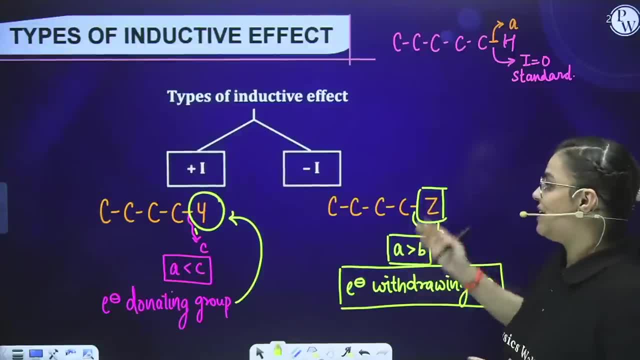 the electrons from the carbon atoms. hence it is electron withdrawing group. hence it is minus i. in other words, if you're not getting this, what is a, what is c? just understand that plus i is the one which is electron donating and minus i is the one which is electron withdrawing. 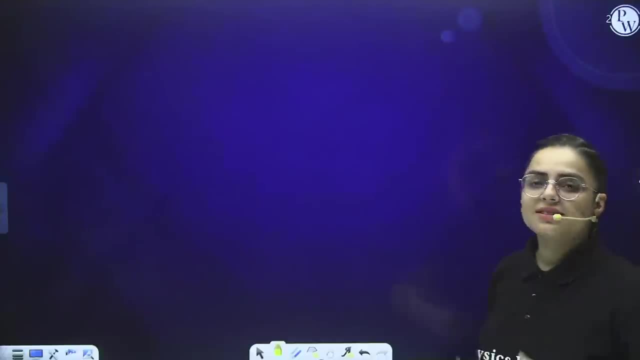 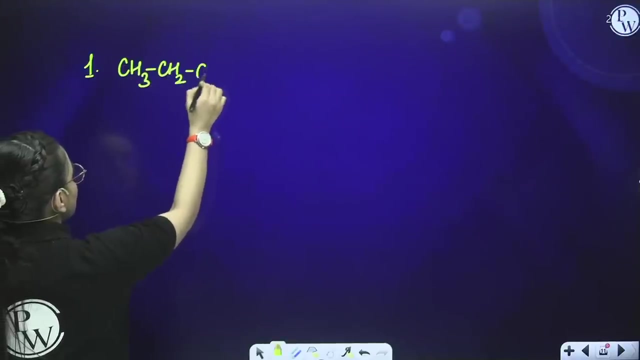 clear. okay, students, now i would take some of the cases and we will understand. basically, where does plus i effect occurs, where does minus i effect occurs? so the very simple case that i would take first over here is ch3, ch2, ch2, ch3. kindly tell me, which kind of effect do you observe over here? 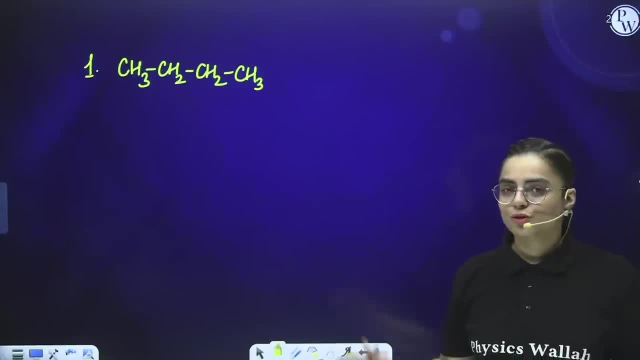 plus i or minus i. so i guess all of you have done this, because here you are seeing only two kind of atoms: one is carbon, another one is hydrogen, and we have seen that we have kept carbon and hydrogen as a standard reference. so if it is kept as a standard reference- it is- it will be what it will. 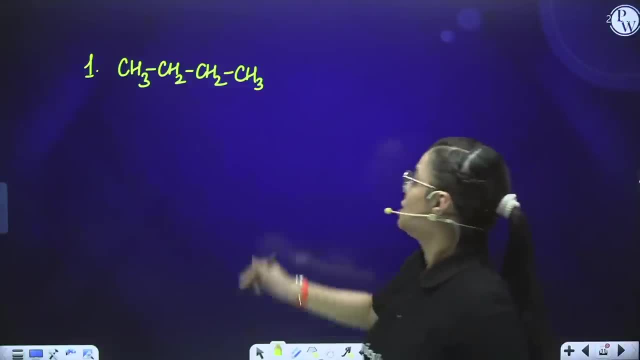 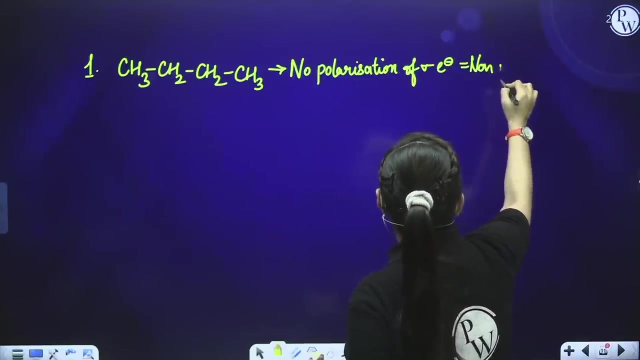 be a non-polar molecule because there is non-polar molecule, because there is no non-polar molecule, because there is no non-polar molecule, no polarization occurring, so there is no polarization of charges, no polarization of sigma electrons. hence, it is what it is non-polar, it is what non-polar, non-polar. 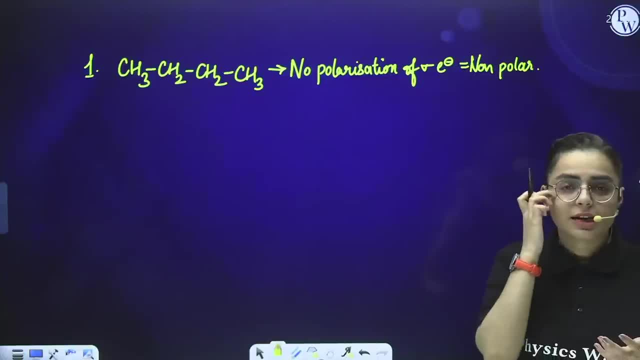 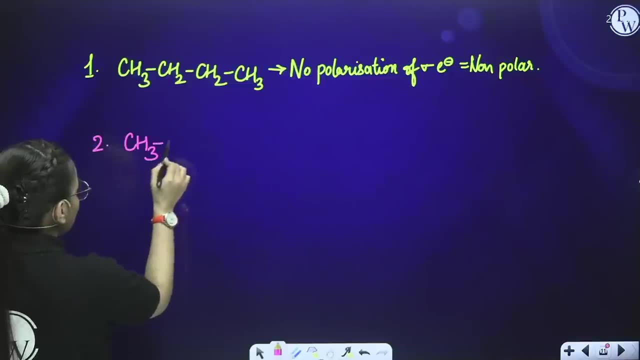 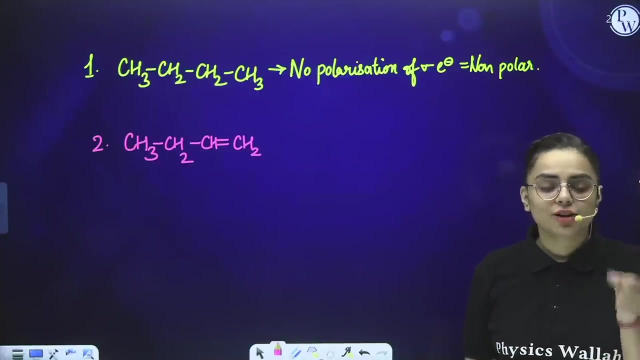 is the one in which there is no poles, no positive, negative poles arises right now. let us take one more case: ch3, ch. okay, now, if i take this case, if i take this case ch3, ch2, ch. double bond, ch2. kindly tell me which kind. 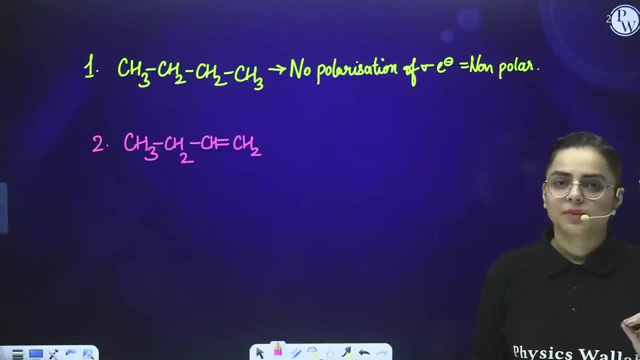 of effect. do you observe minus i or plus i? first of all, what we need to check. what we need to check. we need to check ma'am electronegativity over here. how to check electronegativity? see, see this carbon. kindly tell me the hybridization for this carbon. now, how to check hybridization? to need to check. 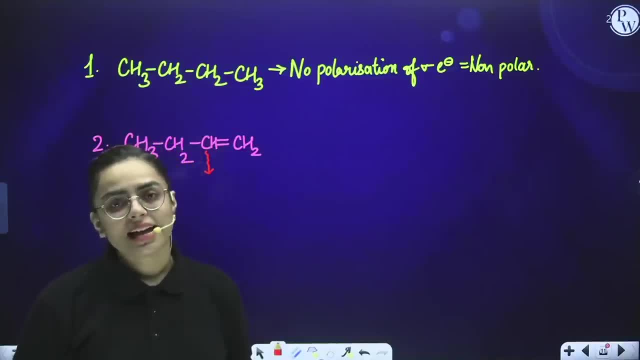 hybridization. to need to check hybridization, to need to check hybridization, we should see the number of hybridization. we should see the number of sigma bonds and the lone pairs. pi bonds are not counted. sigma bonds and the lone pairs, pi bonds, are not counted in hybridization. so there is one sigma. 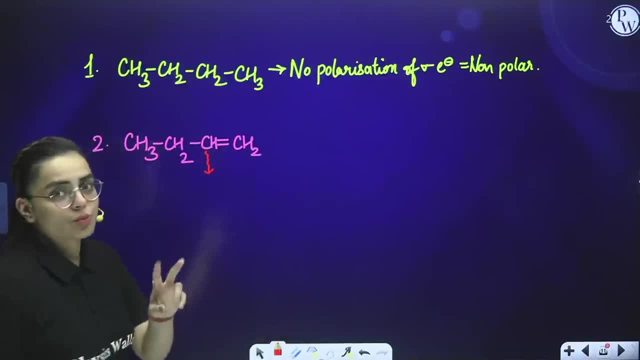 in hybridization. so there is one sigma bond over here, one over here and one with hydrogen bond over here, one over here and one with hydrogen pi bond is not counted how many sigma bonds three pi bond is not counted how many sigma bonds three and for three. let me tell you if you are the sum. 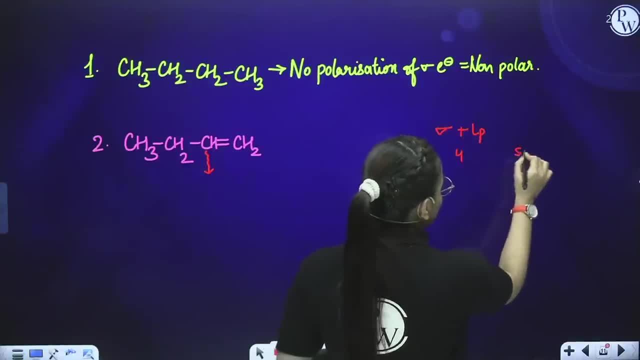 and for three. let me tell you: if you are, the sum of sigma and lone pair comes out to be four of sigma and lone pair comes out to be four, hybridization is sp3. if the sum comes out to be, hybridization is sp3. if the sum comes out to be three, hybridization is sp2. if the sum comes out to. 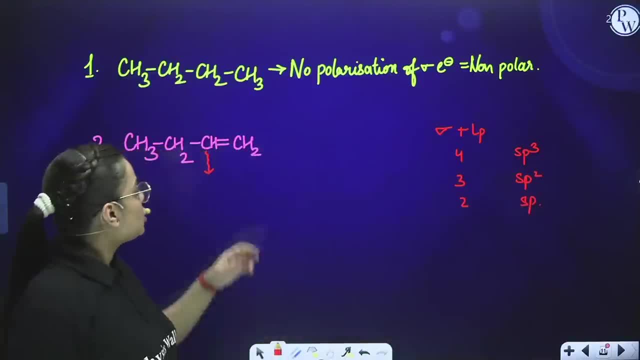 be three. hybridization is sp. this is the basic concept, right. so here, if i talk about this carbon, this is the basic concept, right. so here, if i talk about this carbon, it is making three bonds, three. it is making three bonds, three sigma bonds. there is no lone pair. there is one pi bond, but pi bond. 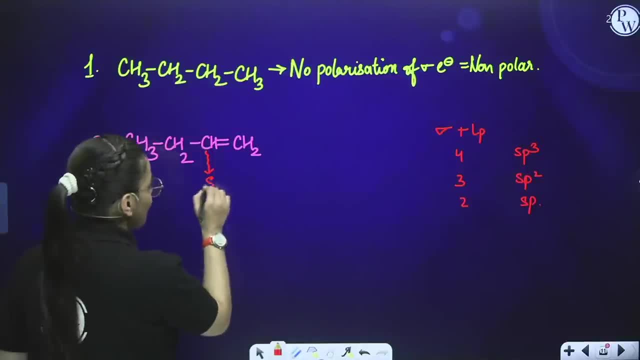 sigma bonds. there is no lone pair. there is one pi bond, but pi bond is not counted in hybridization, is not counted in hybridization. so it is making three bonds. hence hybridization is sp2. now, if i so, it is making three bonds. hence, hybridization is sp2. now, if i talk about this carbon through, 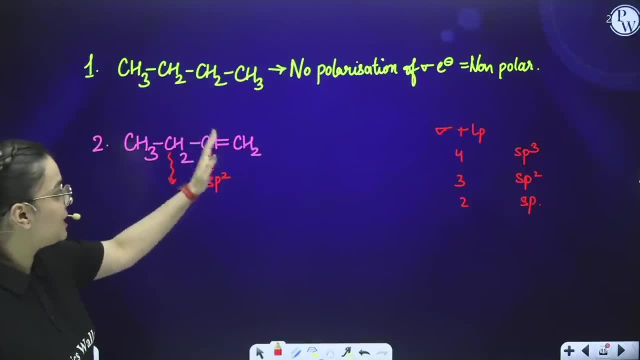 talk about this carbon, through which it is bonded. it is bonded with this carbon. it is bonded with which it is bonded. it is bonded with this carbon. if i talk about this carbon, it is also sp2 hybridized. this carbon, it is bonded with this carbon. if i talk about this carbon, it is also sp2 hybridized, so 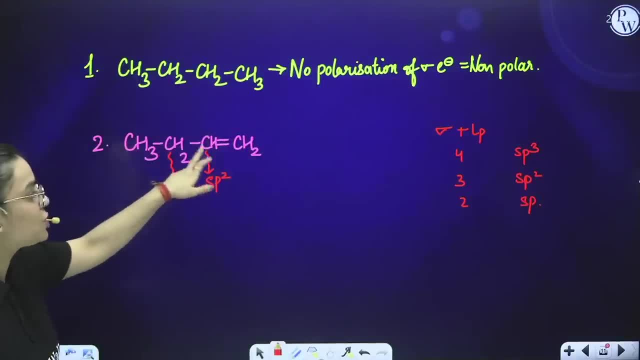 these are same thing. but what is different over here? this carbon which is bonded directly with these are same thing, but what is different over here? this carbon which is bonded directly with sp2. this carbon is what it is making: two bonds over here in two with hydrogen. that means total. 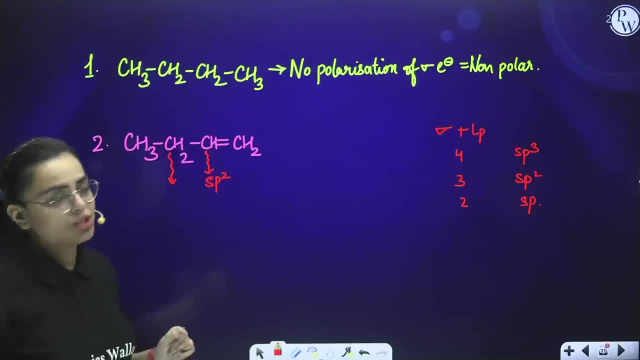 sp2. this carbon is what it is making: two bonds over here in two with hydrogen. that means total four. four sigma bonds are being made now, when four sigma bonds are being made students, what would sigma bonds are being made now, when four sigma bonds are being made students, what would be the? 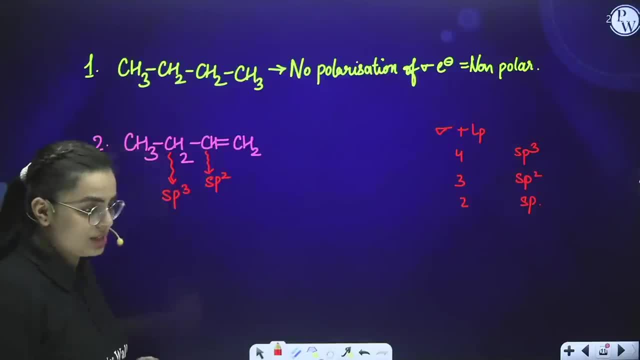 sigma bonds are being made. students. what would be the hybridization? it would be sp3 ma'am now see. hybridization. it would be sp3 ma'am now see. i've already told you percentage s corrector is. i've already told you percentage s corrector is directly proportional to in electro negativity. 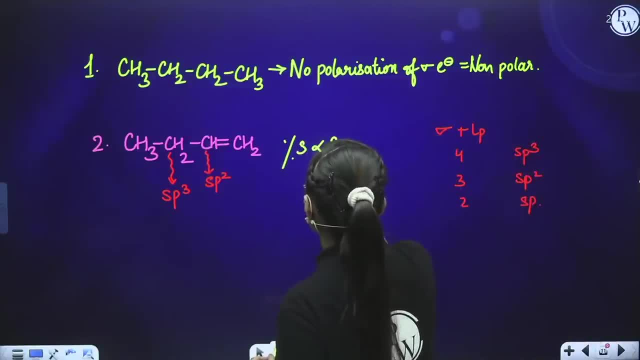 directly proportional to, in electro negativity what i've told you. percentage s corrector is directly proportional to electro negativity. sp will have more electro negativity than sp2, and then comes sp3. i hope so you remember this in the general knowledge concept. so now, which will have? 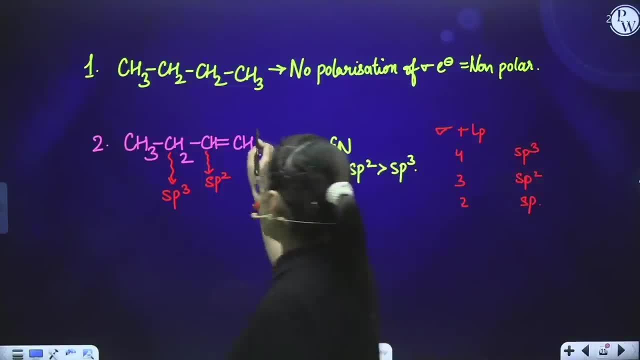 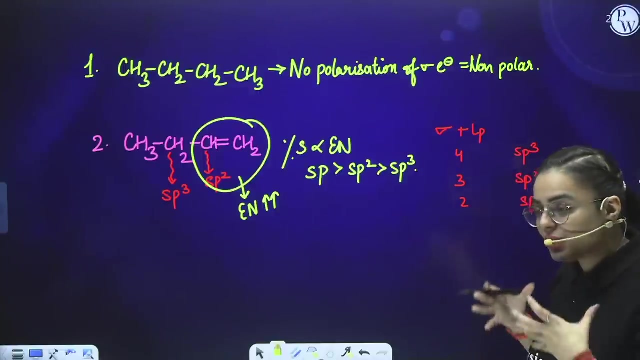 more electro negativity ma'am sp2 will have. that means this: two carbons will have more electro negativity. this will have what this will have: more electro negativity. so which kind of effect it is if it has more electro negativity? electro negativity means that tendency to attract a shared pair of electron. that means it wants some electrons, so it is a. 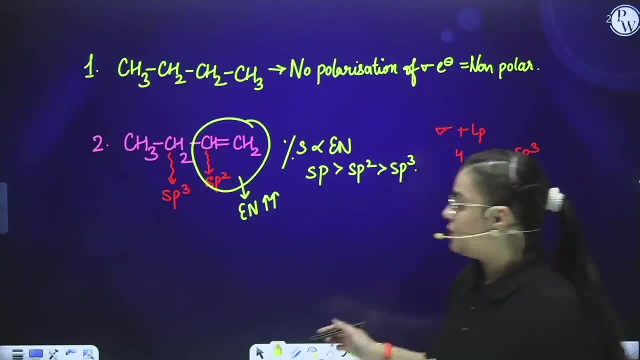 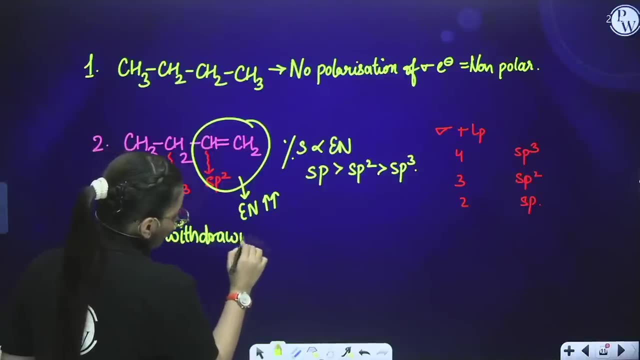 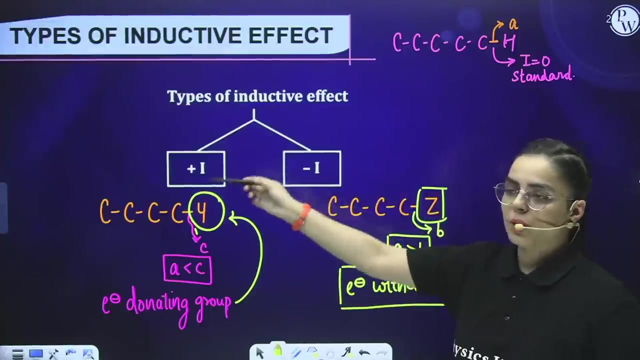 kind of what. it is a kind of electron withdrawing group. now, if it is a kind of electron withdrawing group, so it is. it shows which effect. it shows minus i effect. it shows which effect minus i effect. we have seen in the previous case, see electron withdrawing group. is this one which is minus i? electron donating is the one which is. 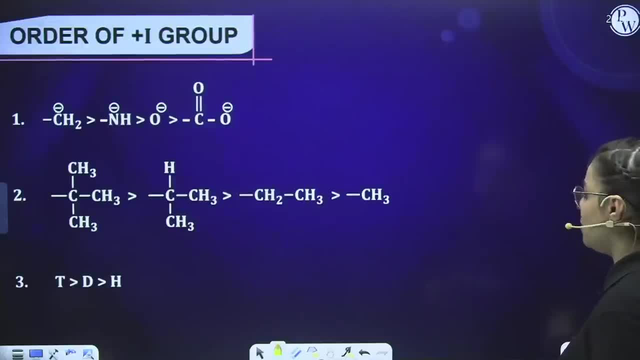 one plus electron withdrawing group. is this one which is minus i? electron donating is the one which is one plus electron withdrawing group. is this one which is minus i? electron donating is the one which is one plus i right now over here. oh on, on this case, only let us see one more case. one more case is still left. 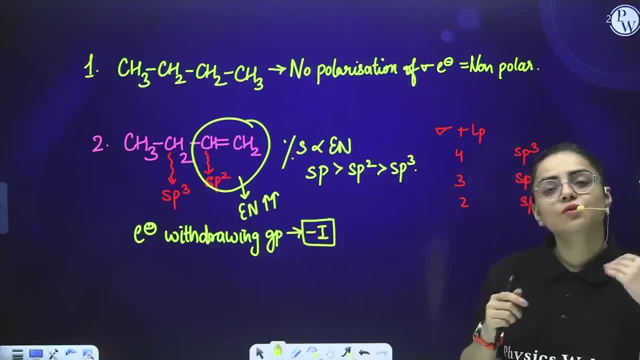 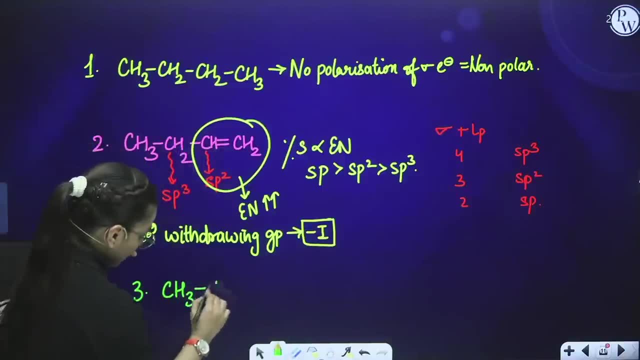 over here. so we will see the other case that is left as of triple bond. let us see of triple bond. if i talk about triple bond ch3 c, triple bond ch, now again, i want you all to apply this case over here. find out the hybridization. if you find out. 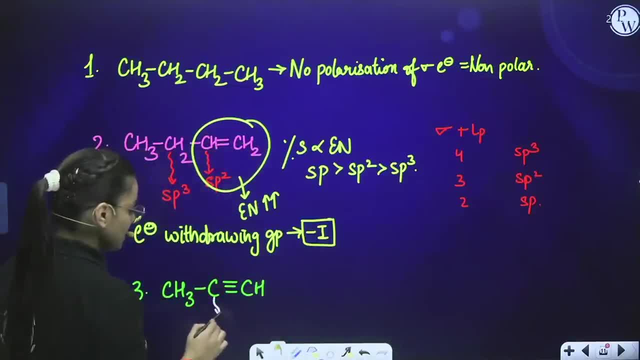 the hybridization of the carbon atoms over here you would say that this carbon is basically making sigma bonds, other two other pi bonds. so if they are making two sigma bonds, the hybridization is going to be sp, and if i talk about this carbon atom again, it is going to be sp, because it is 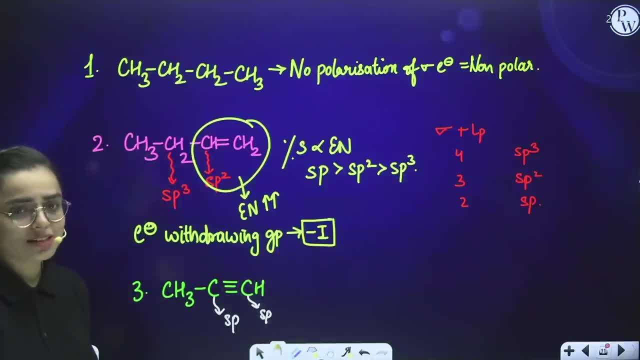 making one sigma bond over here and another will will be there with hydrogen. if i talk about this carbon atom, it is making four bonds. that means it is sp3 hybridized. so this two are sp, while this one is sp3, which will have more electron negativity again. sp will have more electro negativity now if 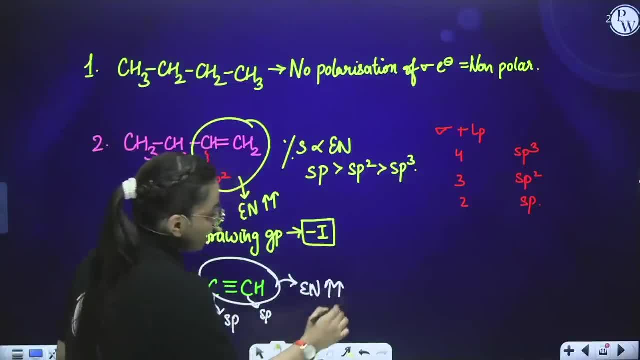 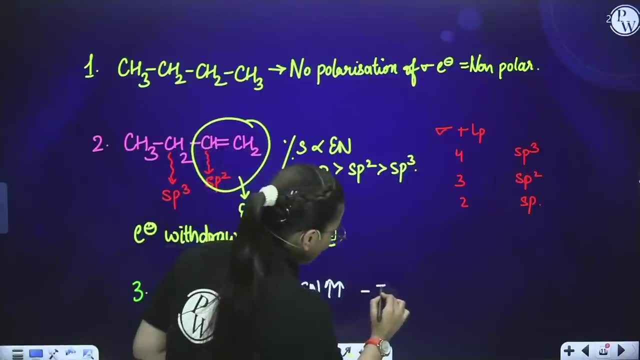 this has more electronegativity. that means if you add another charge and then add more carbon bond, means they require electron. they want electron to be shifted towards them. now that means they are electron withdrawing group. that means it shows minus i effect. it shows which effect it will show. 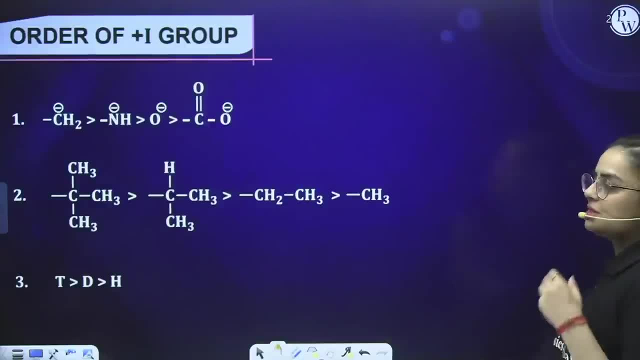 minus i effect. hope so it is clear to you people. now, students, coming to the important concept that is the order of plus i group. now we have seen inductive effect. what is inducting effect? let us revise it. it is distance dependent effect which basically is seen up to three or four. 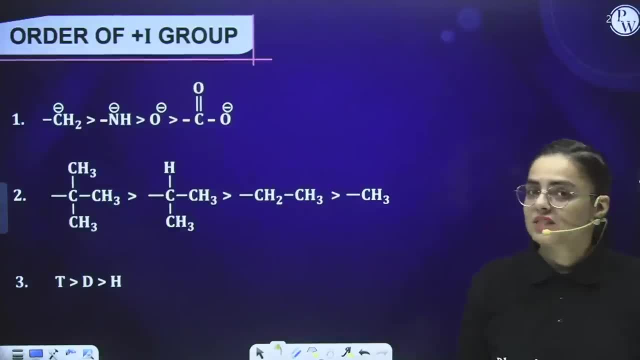 carbon atoms. it is permanent effect. it is delocalization of sigma electrons. right, this was inductive effect. now the second thing that we understood was about the types of effect in between. we got a lot of general knowledge about the organic chemistry. right now, here comes the. 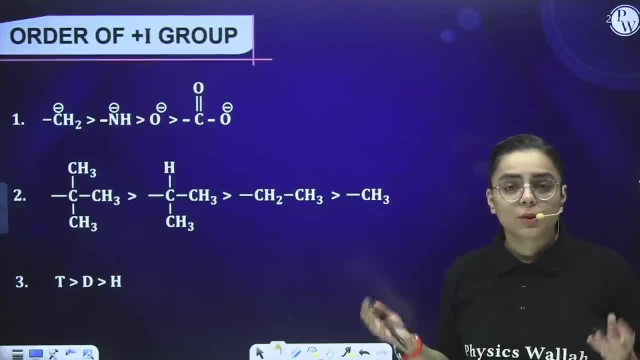 order of i groups: plus i group or minus i group. whenever you are being given some question, they will ask you which is more stable. so how you are going to tell which is more stable? if you remember this order, it will help you to do questions even very fastly, right? so? 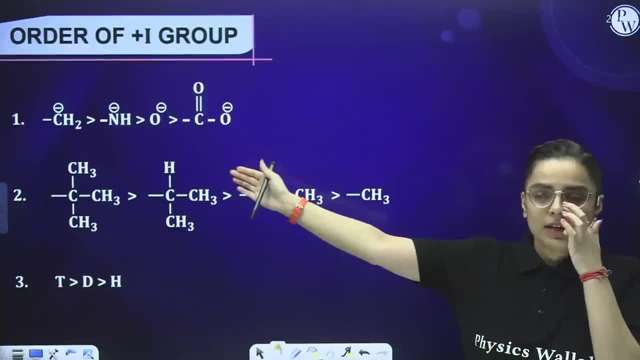 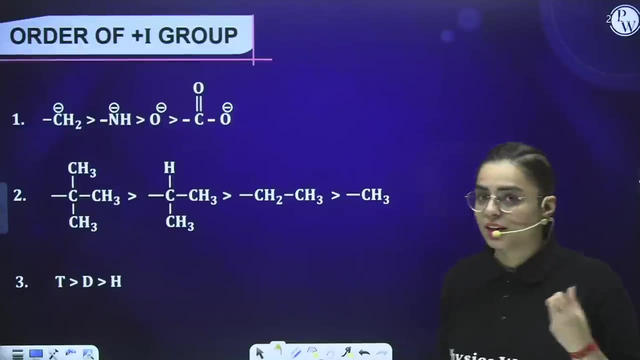 students, if you see the very first case over here, you see whenever you are going to see ch2 negative group. now what does happen over here. ch negative here is, you know, here it will. it will have more donation. now, if it will have more donation, as i know, electron donating group is what it will show. 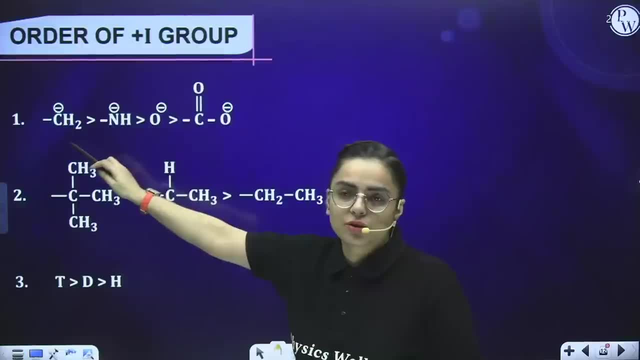 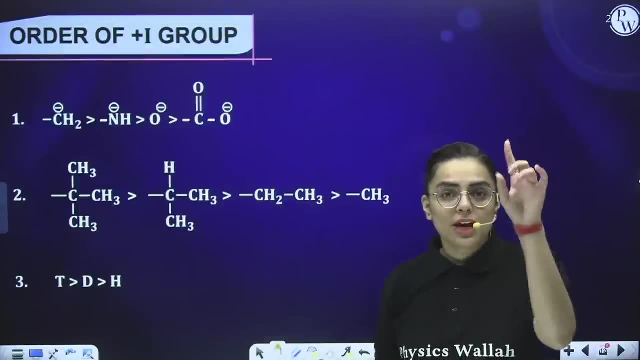 plus i. so this will show plus i more because it is more electron donating. then comes this nh negative, then comes o negative, as you have seen the case of o negative previously when i was given oh and o negative in the case when i told you to do this. then it will show plus i group. so this will show. 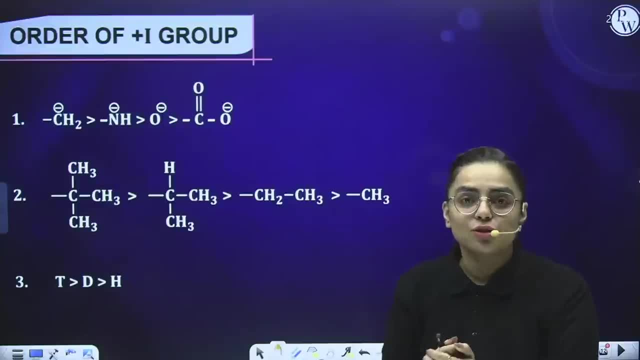 plus. but you know, if you do all thoseBreak-out, you will see that when you show something here, the stops as you are doing the o negative, then you will see the link that you should have the now Emily you saved. so every time you tons of. if you know, let us say you are going to. 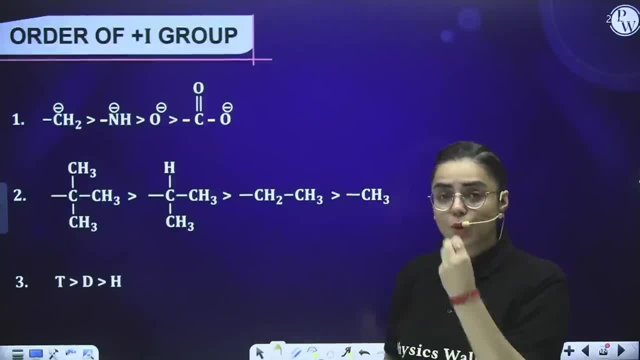 see whatever you want to see: magnetic field, as you can see, rods are here. so this time, on the left of this varian, 굉장히 stable statistic, then you do not expect go homeボ, you don't expect to see much electric field on the right side of it, because it is honestly 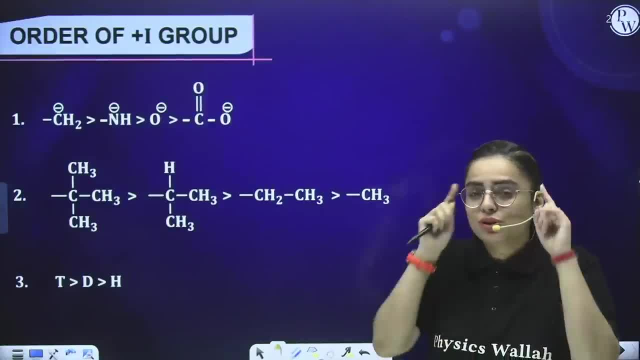 fun, even if it is graphically создatd in the wrong way. so what you do have to find them on the left side of this column, right? so check the link there. oh see, the 0 negative by 0 or 0 Janeiro, it would equal right, since, as one from Radam k��, it was something Peak method, but please. 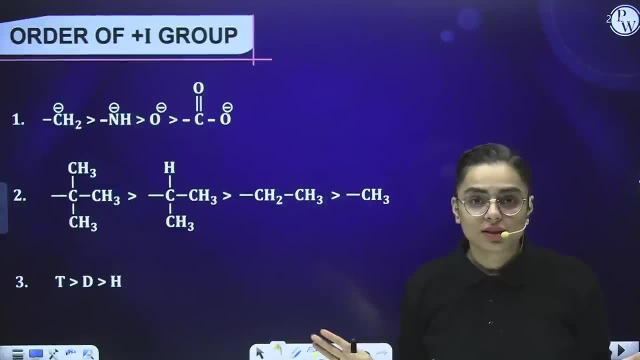 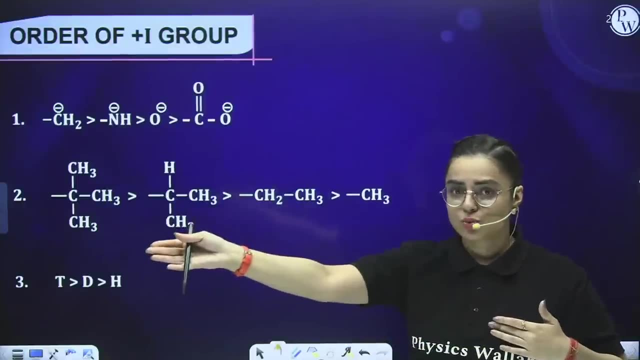 conclude quadrant 1, then calculate by road that which John the negative is playing it just- and electron density. both are different concept. electron density is the one in which we have seen that whosoever he has electron density more will give its electrons to the another one. but whosoever 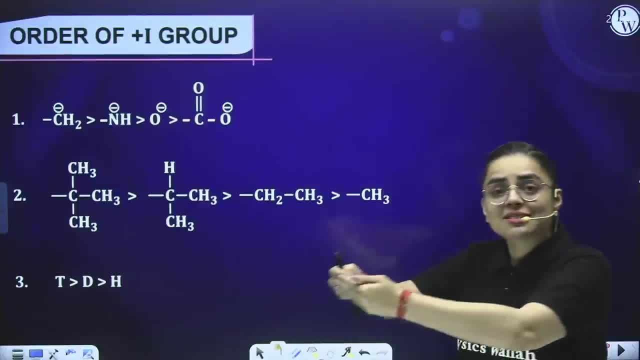 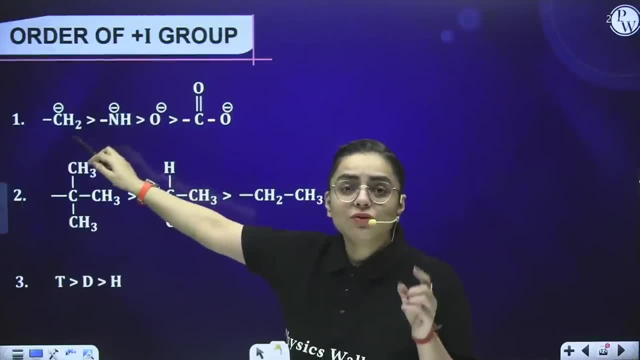 has more electronegativity, they will have the tendency to attract electron towards itself, clear. so here, as i told you, this will donate electron. this, if this will donate electron, that means it is less electronegative. that means it is less electronegative. now, don't compare this. 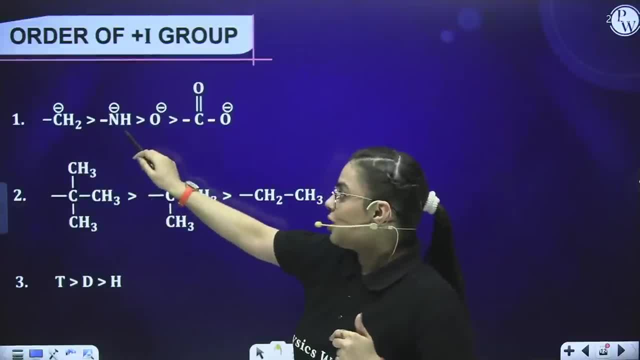 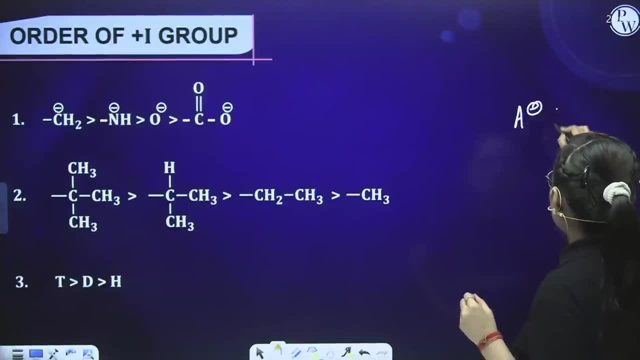 with electron density concept. okay now, if i talk about this, nh negative this o negative o negative? we have already seen that. uh, you know a negative, a and a positive. what i told you. i told you: this will have more electron density than this, than this. that means, if i am talking about plus i group, 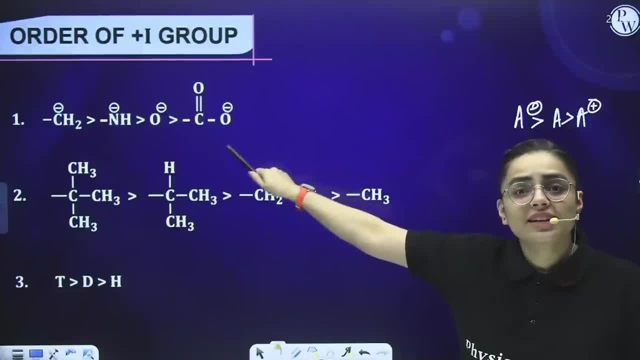 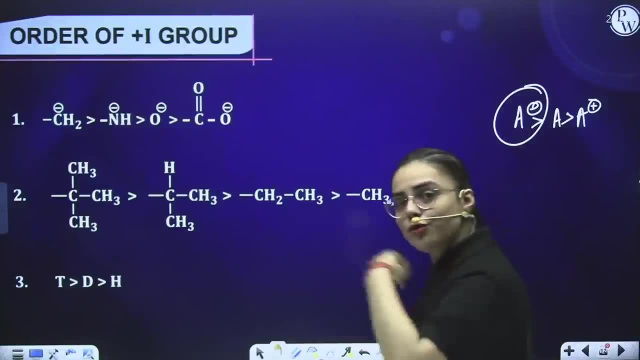 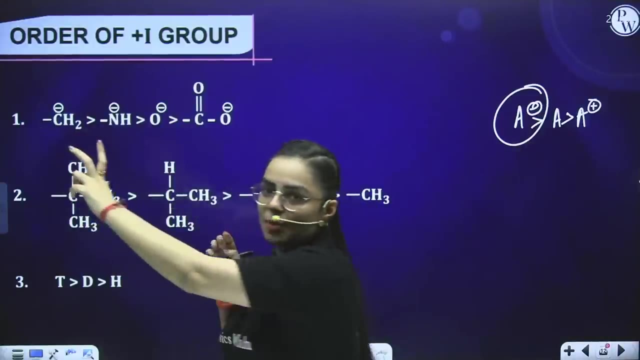 all i want is: first, the negative charge is one. why the negative charge is one? because the negative charge is one: have more electron density now. if these have more electron density, it will donate now, if they will donate, they will have plus i group. so you will see what. you will see a order where first minus- you know- negative charges comes in plus i. 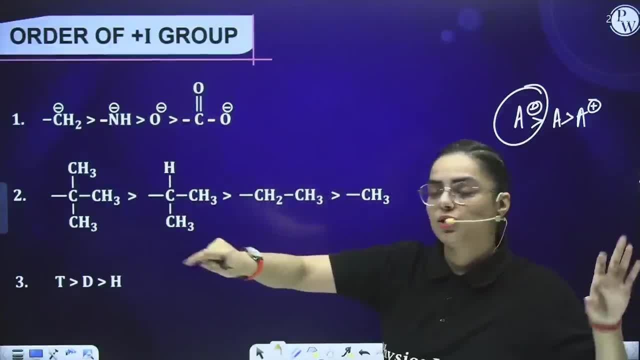 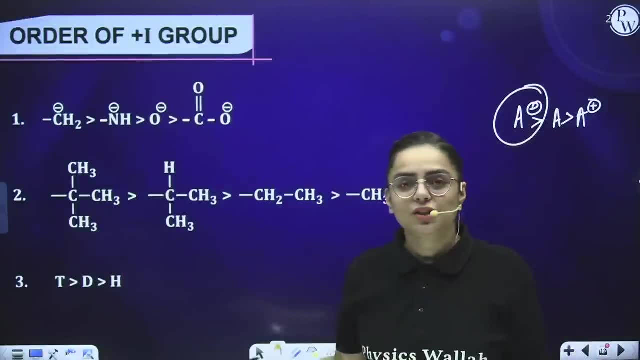 order. always remember first of all, the first order that you are going to observe is of negative. why? because they have more electron density, and more electron density means they will what they will donate, and if they will donate then they will have plus i group. then after the students, what? 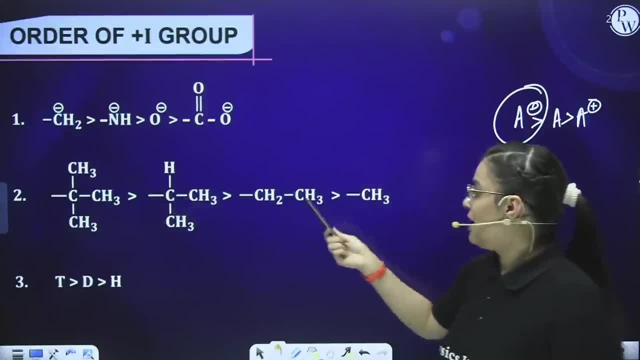 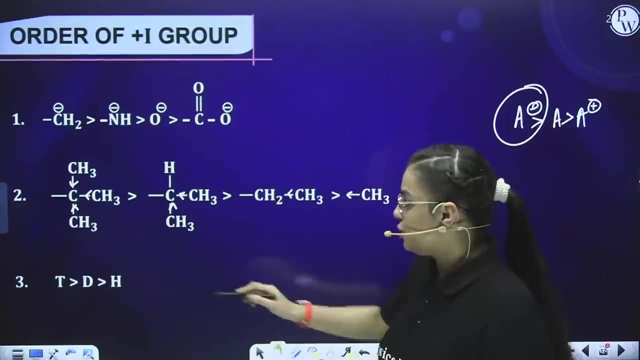 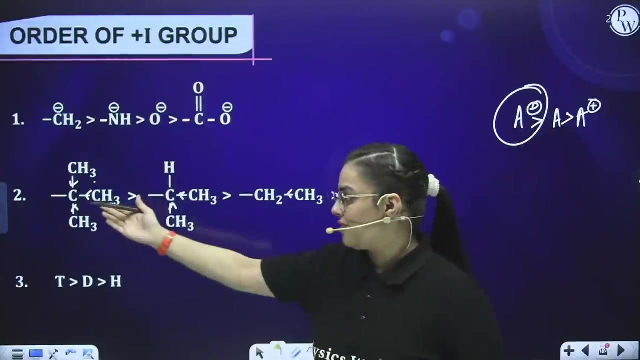 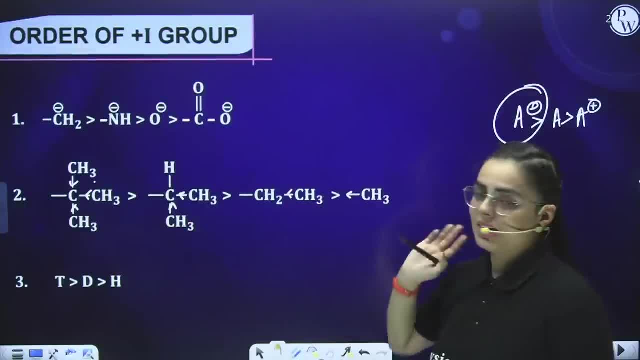 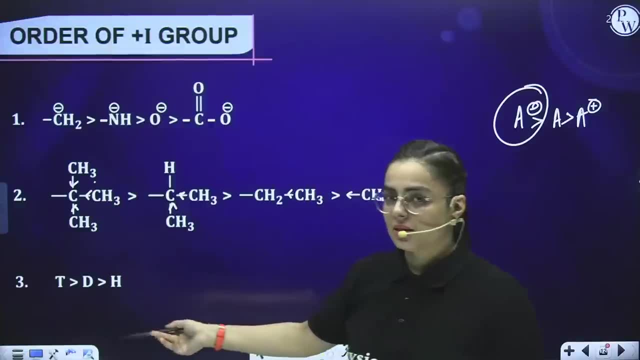 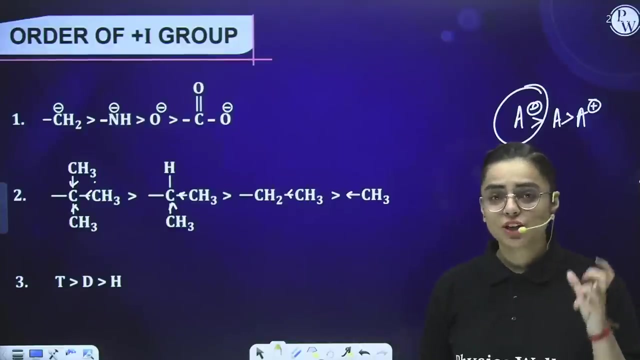 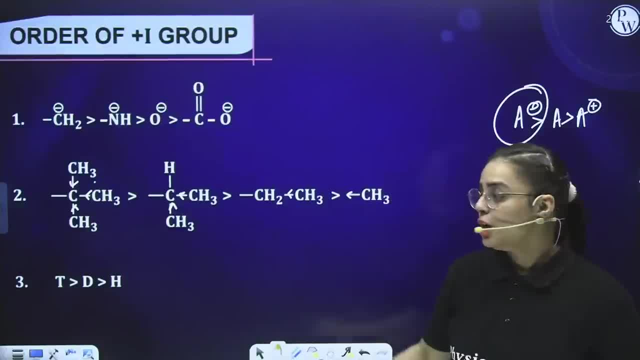 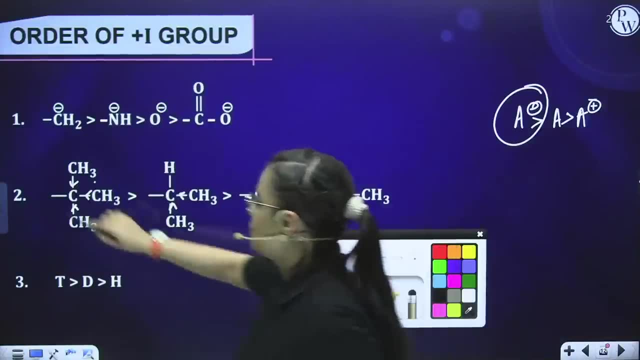 the difference over here. so whosoever is having higher atomic mass will donate more. now, if they will donate more, they will show plus i group. so these you have to learn. first order, i guess you have to learn, it is quite simple. but this you don't have to learn, because three degrees more. 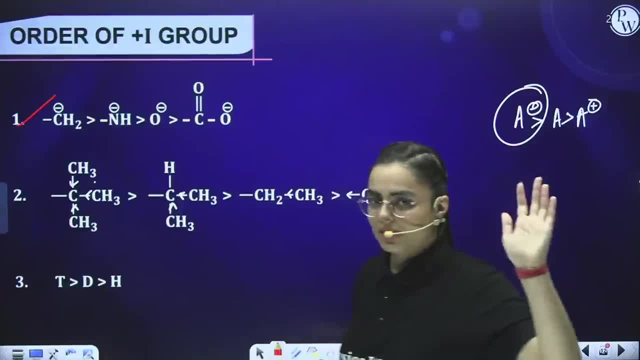 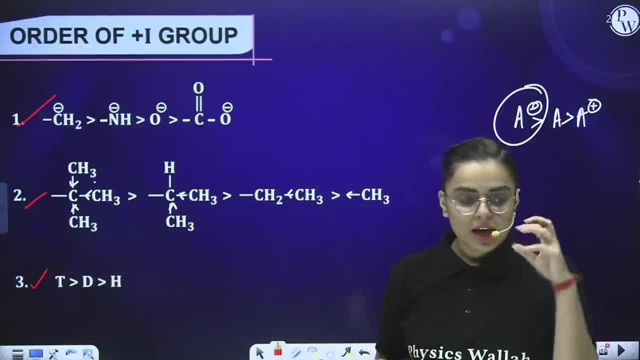 stable than two degree, than one degree. it is quite easily. we get in our minds right other than this. this is also very easy. why this is easy? because if they are isotopes, then you need to keep the atomic mass in your mind. more the atomic mass, more will be the donation, more will be the donation. 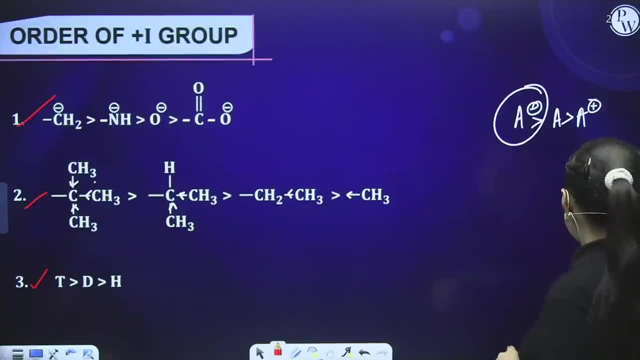 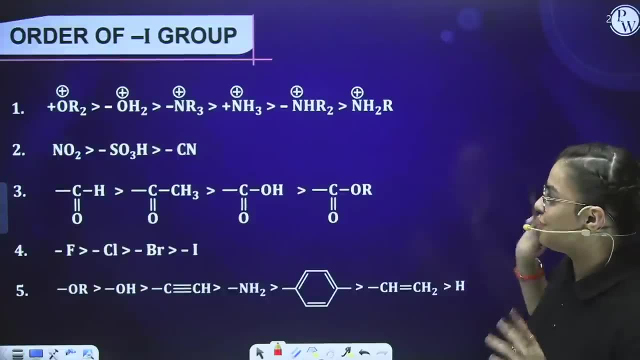 more will be the plus i group. clear, okay now. similarly, we see the order of minus i group. now, if i talk about the minus i group, this is order now. first of all, see the difference in the previous case. we also the first groups, contain the negative charges here. all these group contain 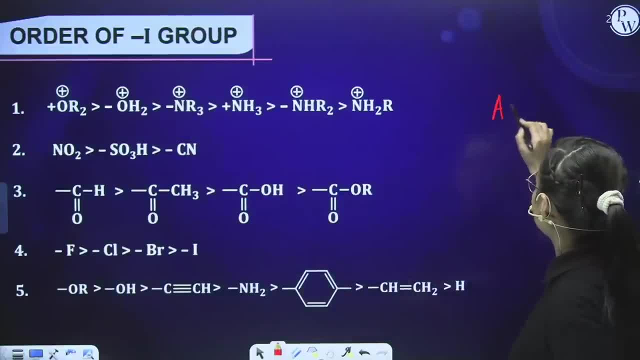 the positive charges. again, i am repeating the same concept. if you are given a negative, if you are given a positive, or if you are given a which will have more electron density, a negative which will have less electron density, this, the one which is having less electron density, will have less. 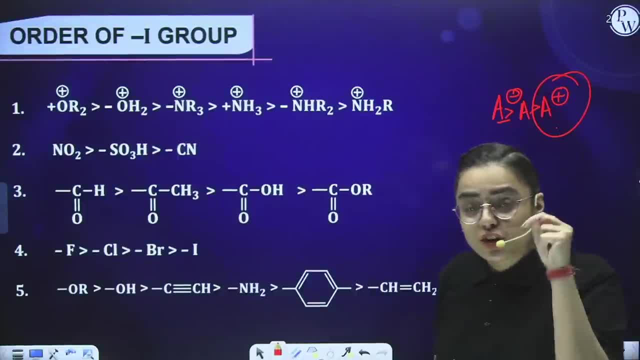 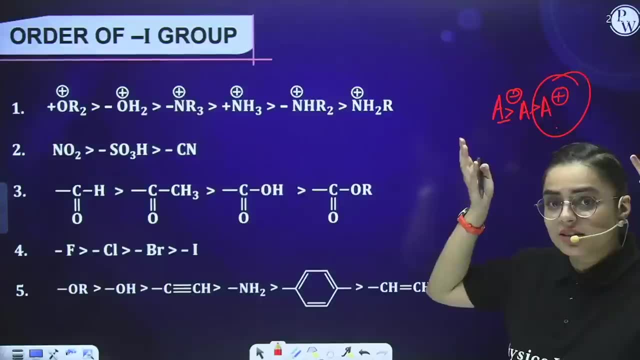 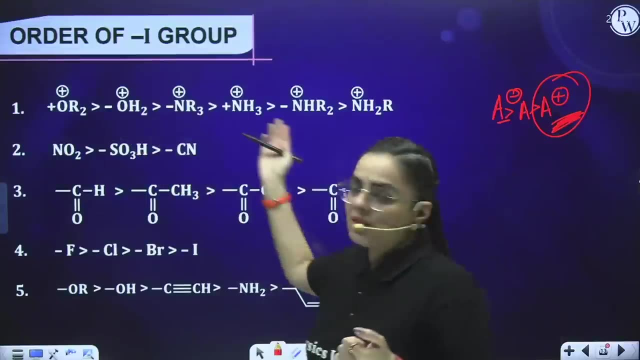 electron density, not negativity. electron density less will what will withdraw its electron when it is withdrawing electrons to make it electron density more. it is known as minus high group. so the positive one will withdraw the electrons. hence the positive ones are written first, right. so now there is an order of: or two positive, oh two positive. now this is the exception over here. 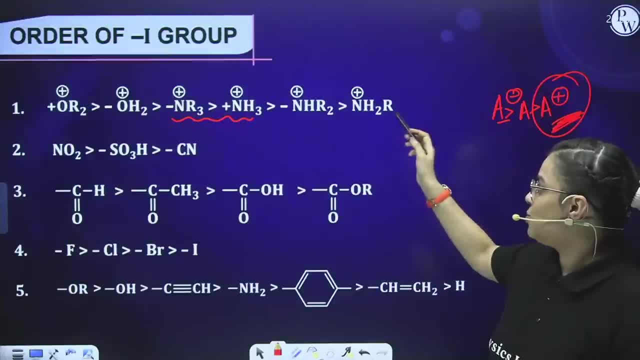 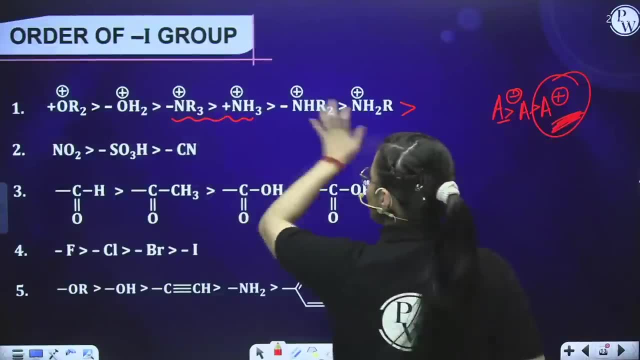 just you need to keep in your mind right, then comes nhr2 and then comes nh2. are positive, now comes the second, the order. this order lies in this way: firstly you will write, then secondly, then thirdly, then fourthly. this basically you can write in one single horizontal line, also clear. 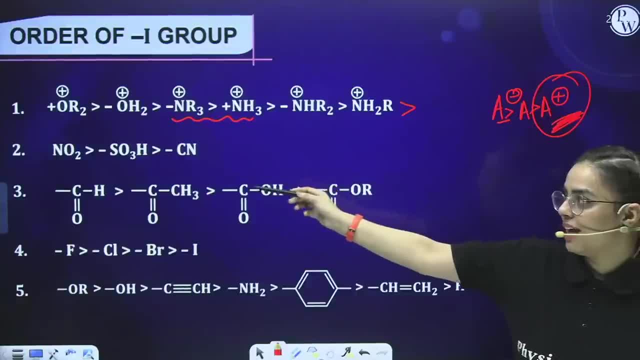 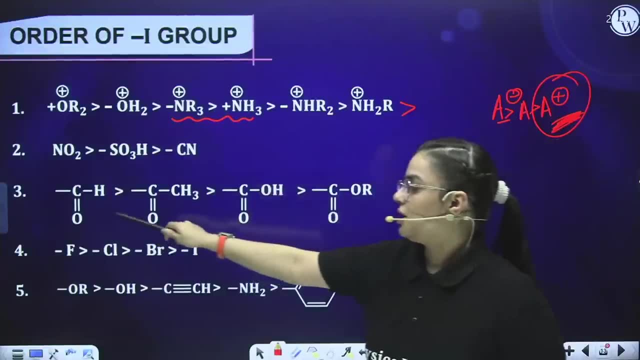 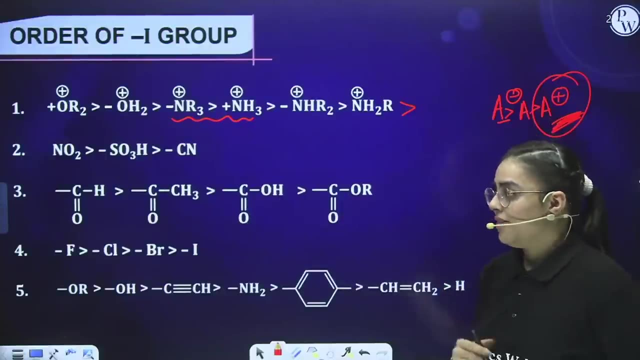 now, if i talk about the second one, we have no2, then we have so3h, then we have c and cyanide. if i come across the next one, then we have this group: coh, c double bond, oh, then we have c double bond. ch3, then we have c double bond, oh, carboxylic group, then we have c double bond, or then comes. 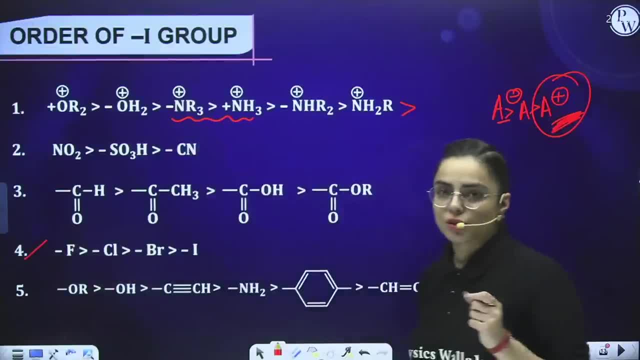 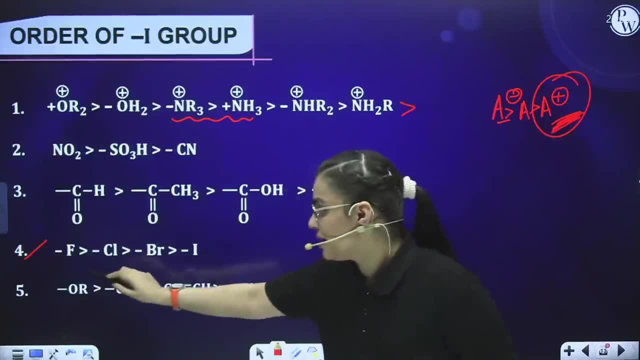 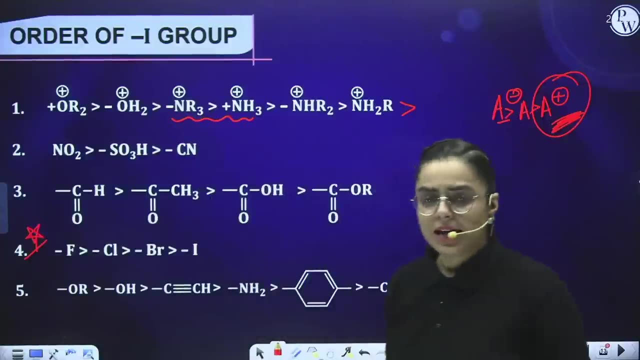 this one. it is quite different and it is quite important. also, this you have to keep in your mind: for minus i effect fluorine has more minus i, then chlorine, then bromine, then iodine. kindly put a star over here. this you are going to observe in many of the cases, in many of the cases. so put a star over here now. 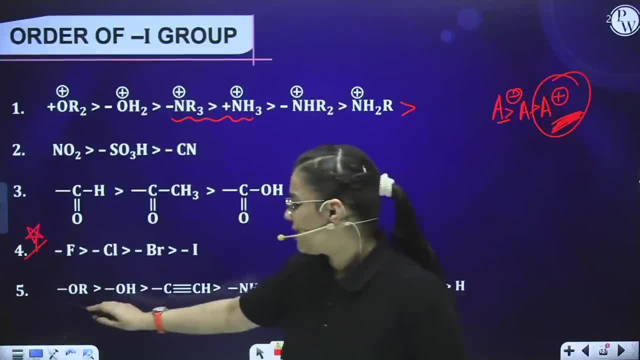 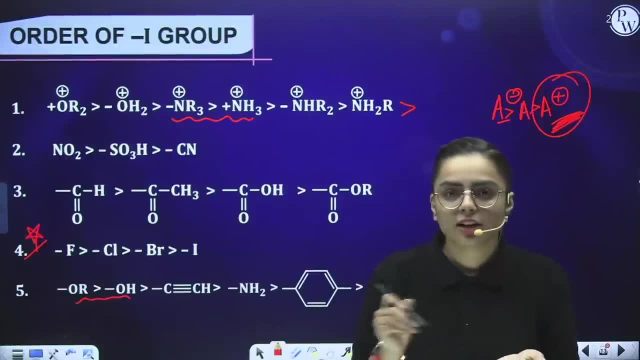 if i talk about the last one, this is the last one. this is also, again, the exception over here. okay, now, this order you need to keep in your mind, don't you know? don't keep on writing and learning the numbers. no, no, no, just read it once, twice and thrice. that's it, when you're going to apply this. 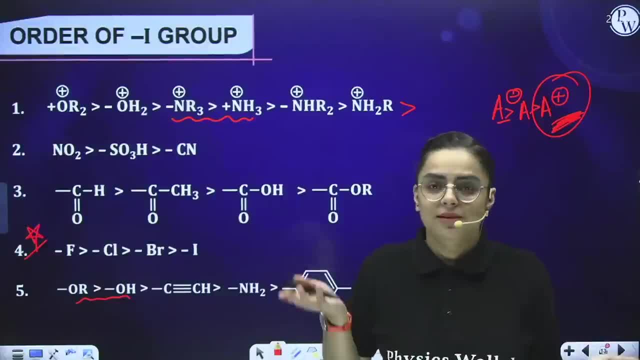 in questions. you will automatically get to know, you'll compare and learn. you know you'll compare- this is plus i group, this is minus i group- and how you are going to compare. you're going to compare with the concept of electron donating and electron withdrawing, and that will only be learned when you 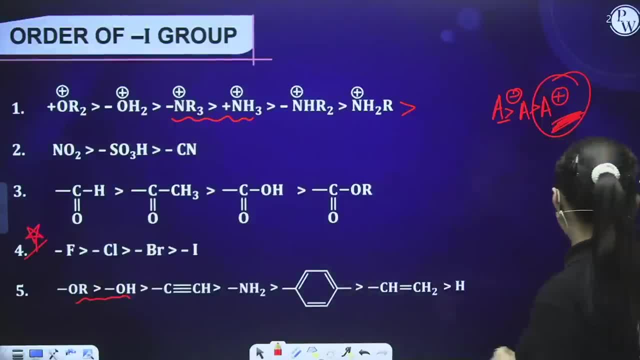 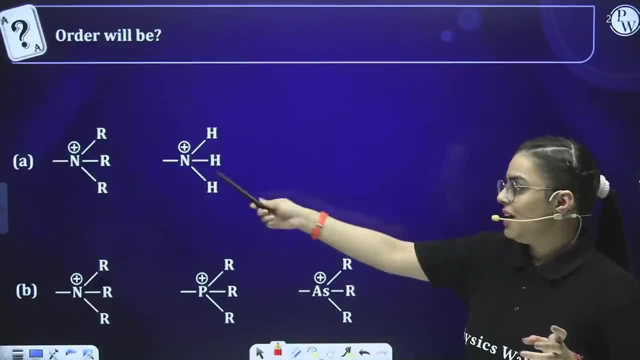 are going to practice more and more questions clear. so, students, this was all about the order of plus sign minus i. now there are some questions of order. first of all, if i talk about this order now, what do you observe over here? we observe that, ma'am, the central atom over here is nitrogen over. 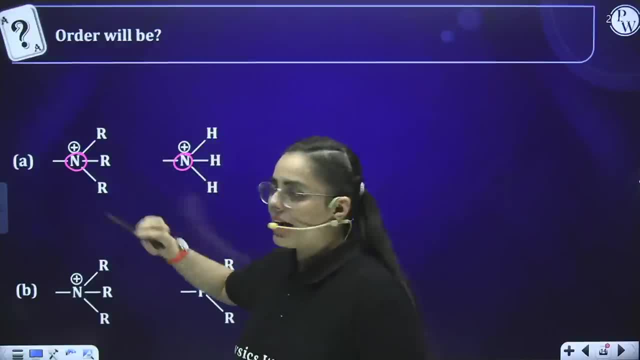 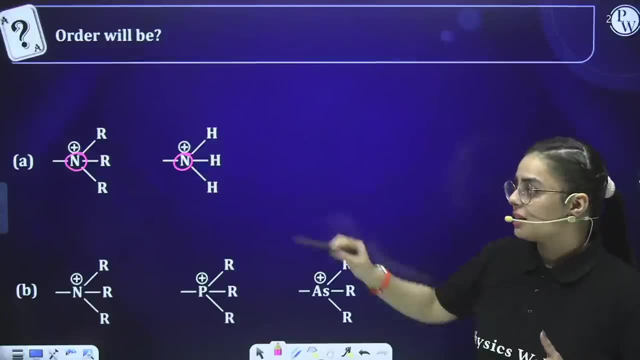 here is also nitrogen. this contains what it contains- r group, alkyl group- while this contains hydrogen, this contains hydrogen. ma'am, we know that. what we know over here is that we have to tell the order which order it follows. does it order it? does it follow minus i or plus i? first, 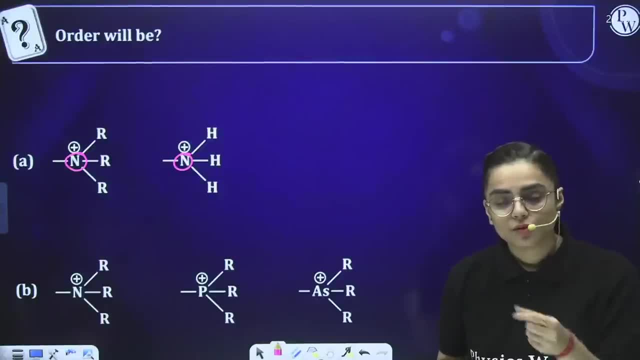 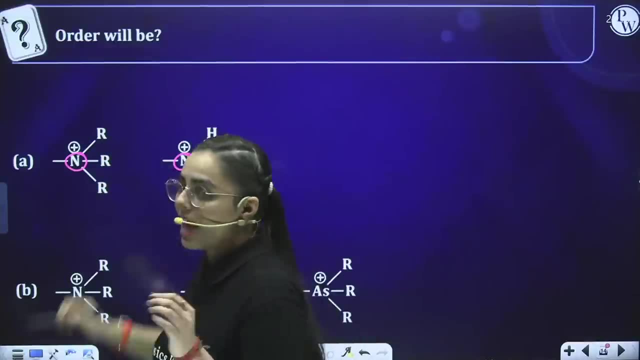 we need to identify this. you know, plus i is the one which is electron donating, minus i is the one which is electron withdrawing. now what happens over here? we know that r group r group refers to ch3 or ch2. ch3- we have seen the order of 3 degree, 2 degree, 1 degree. they all were what they all will. 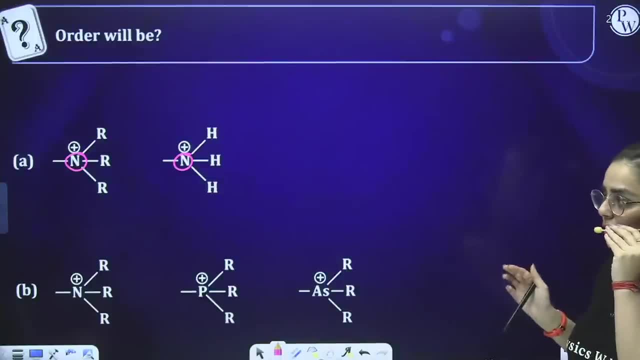 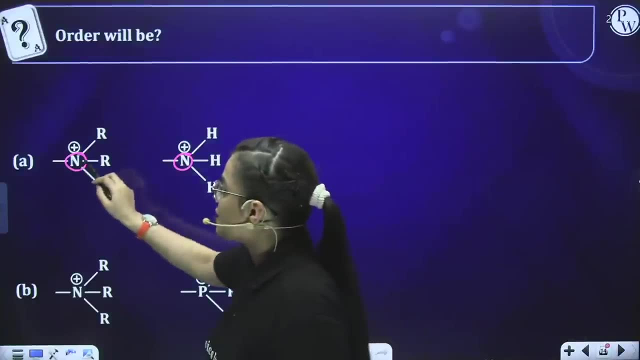 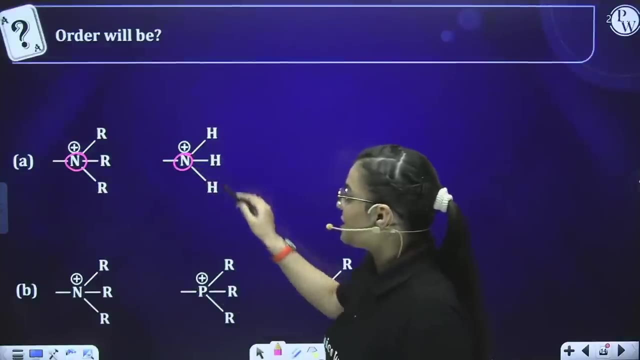 you know what they were doing basically. basically what they were doing. they were seen in the plus i effect, right. but here what we are seeing, these r groups are attached with nitrogen. these are attached with nitrogen and it has positive charge over here. now this n positive is attached with. 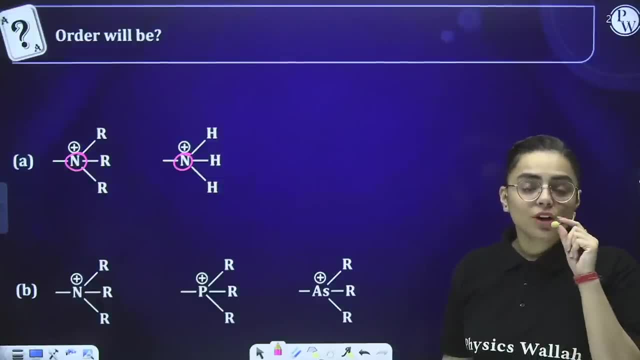 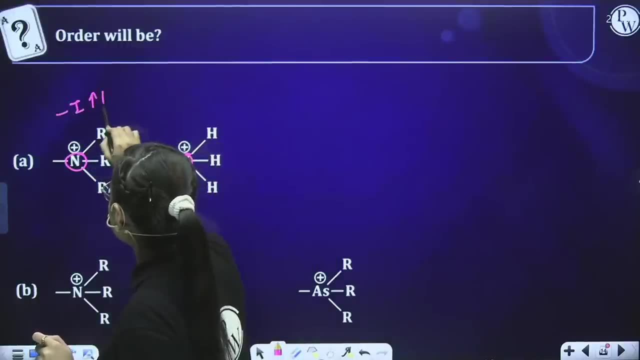 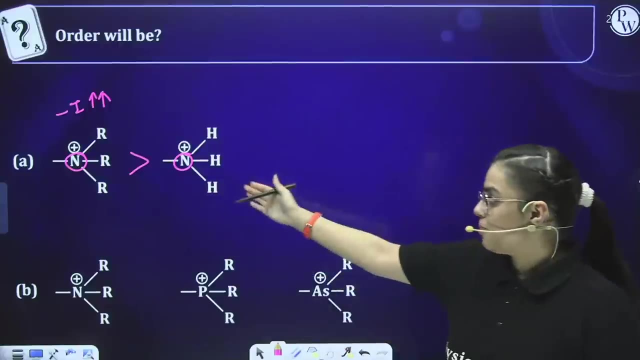 hydrogens over here. this is attached with hydrogen. now, what we see that they will have, this will have minus i more than this. this will have minus i concept more than this. minus i. that means electron withdrawing more than this, because they will withdraw electrons more as comparative to this, because hydrogen is. 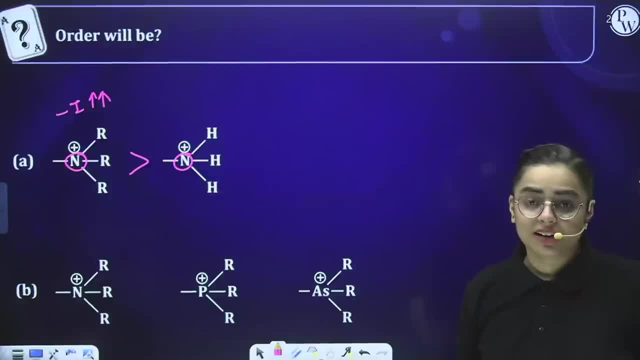 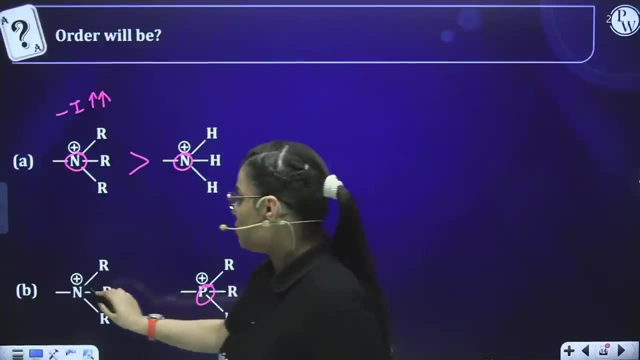 least electron negative, because hydrogen is least electron negative than nitrogen. that's why, if i talk about this case, in which we see that central most atoms are different, here central most atom is different: here is itions broadкт, here is a Citrogen, here is phosphorus, here is arsenic. so what do we observe? 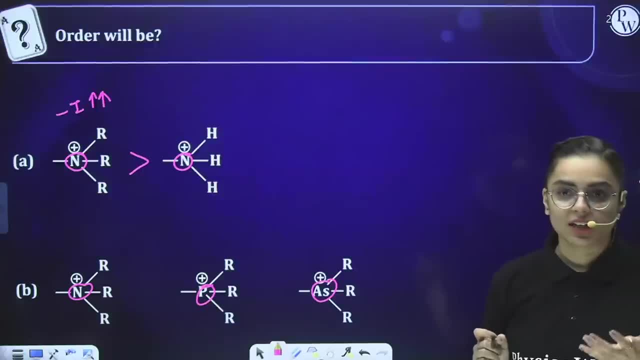 here over here we know that percentage as character is directly proportional to electronegativity. so the deciding factor over here is the central atom, because other than the central atom all acquires the r group. when all acquire the r group we know that percentage as character is directly. 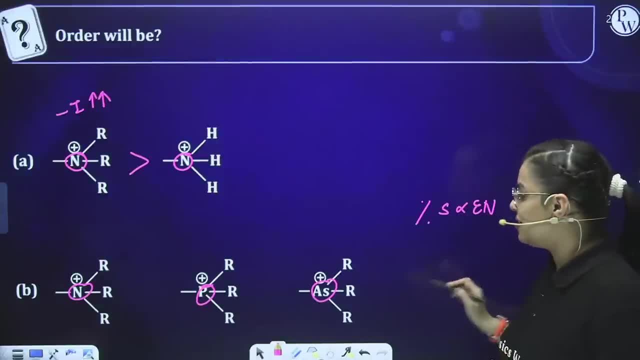 proportional to electronegativity. right and other than this. we know that deciding factor is what? deciding factor is our central atom. now here, though, whosoever will have more electrone negativity- listen to this- whosoever will have more electronegativity will have minus i effect. 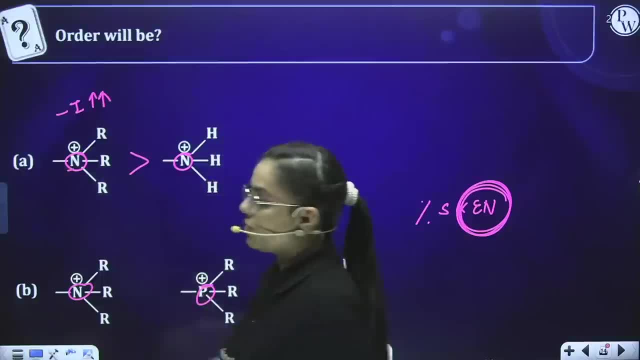 we have seen in this case, nitrogen is having what more electronegativity than carbon. so it if it has more electronegativity. more electronegativity refers to as tendency to attract. tendency to attract refers to as electron withdrawing. electron withdrawing refers to as 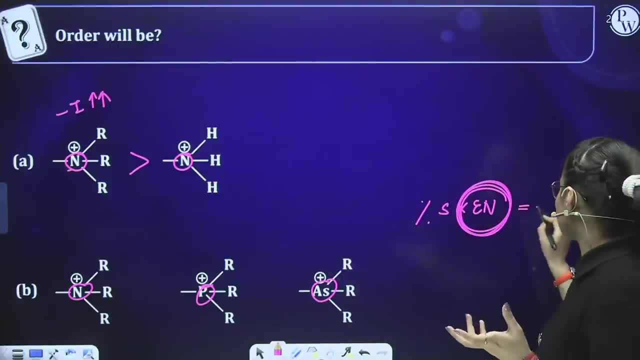 minus i effect electron withdrawing refers to as minus i. that means the person that is going to have more electronegativity is minus i, because it will attract it will withdraw. now who will withdraw? which will have more electronegativity now, in this case? who have more electronegativity? 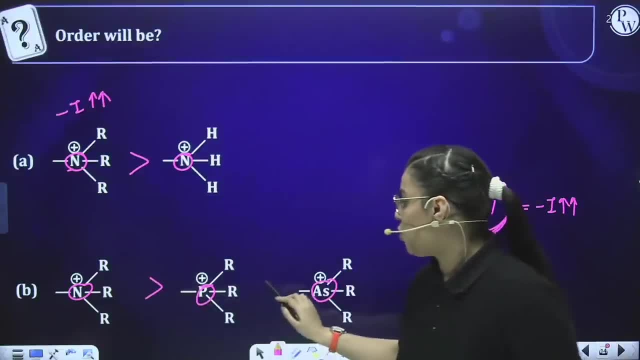 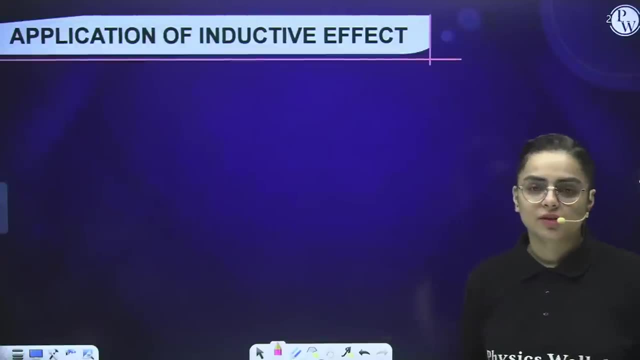 students. nitrogen now, if it has more electronegativity, the order is going to be this. the order is going to be this hope. so it is clear to you. now, students, comes the application of inductive effect. now, if i talk about the application portion, all i would say, in the application we are: 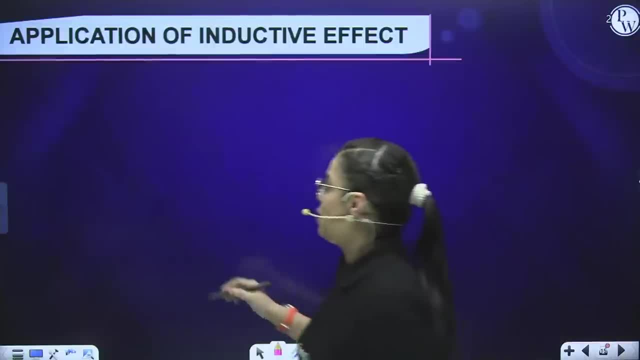 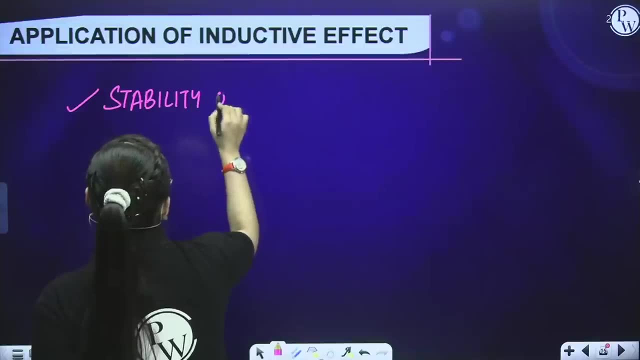 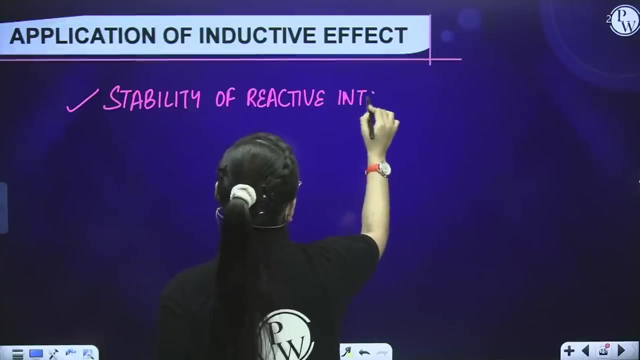 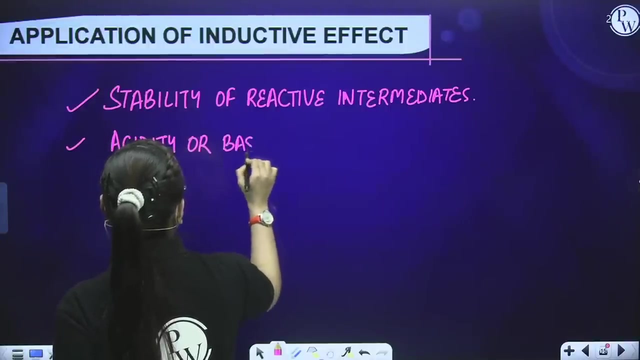 going to see the stability of the reactive intermediates. what we are going to observe over here is the stability of reactive intermediates. other than this, students, we study about acidity basicity. this is all in the application portion. other than this, you understand that we are going to study about acidity basicity. 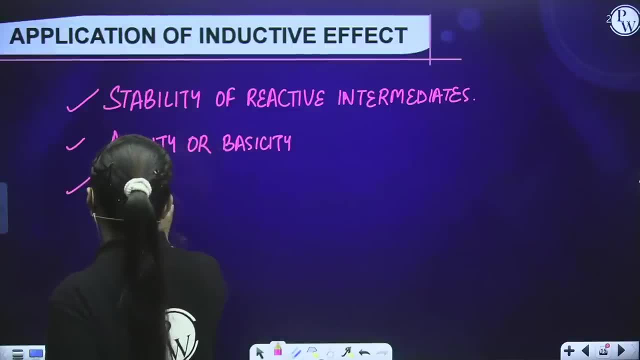 you understand about dipole movement, melting point, boiling point. dipole movement, melting point, boiling point. okay, other than this, students, what do you see here? you see the stability or you can see the reactivity of alcohol carboxylic acid. you see the stability, or you can see the reactivity of alcohol, carboxylic acid. 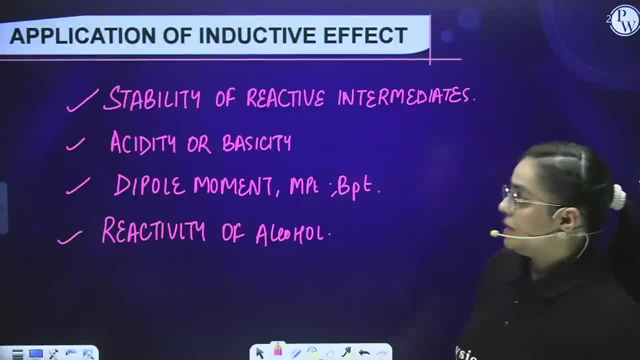 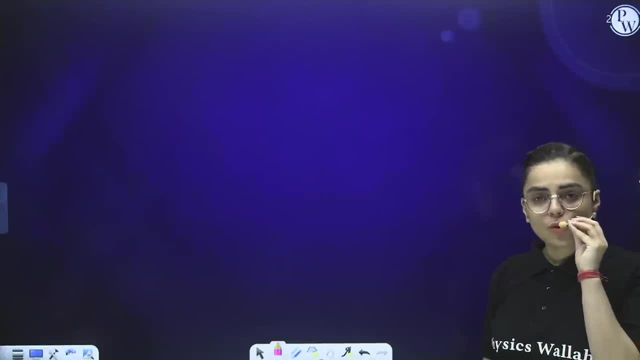 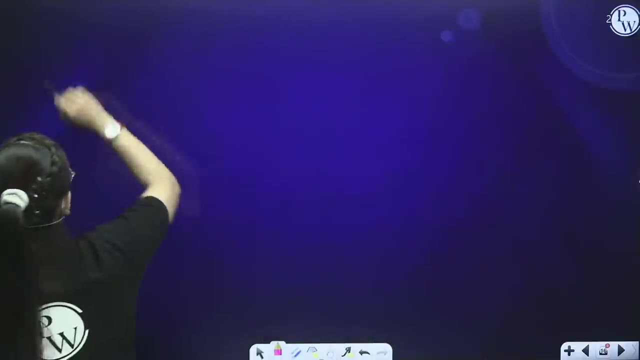 okay, now students are. these were the applications of inductive effect, one by one. i'm going to explain you in detail if i talk about the first application, before that, i want you- want to want you all- to understand one more concept of general knowledge. now, what is the concept that we are going to understand over here? that is about? 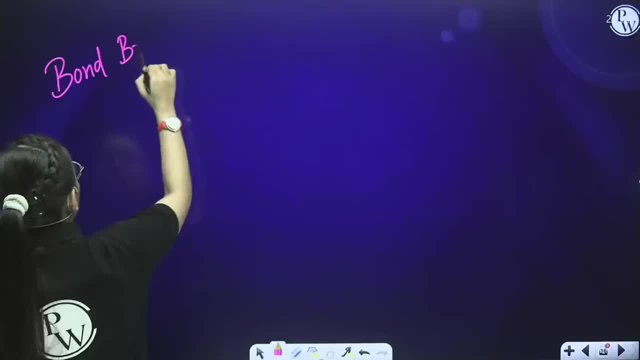 bond breaking. that is about bond breaking concept. now, what do you mean by bond breaking, ma'am? okay, see, bond breaking students can be of two types. it can be of two types. now what are the two types we define bond breaking into? if i talk when there are same atoms given to you, when there are same atoms, 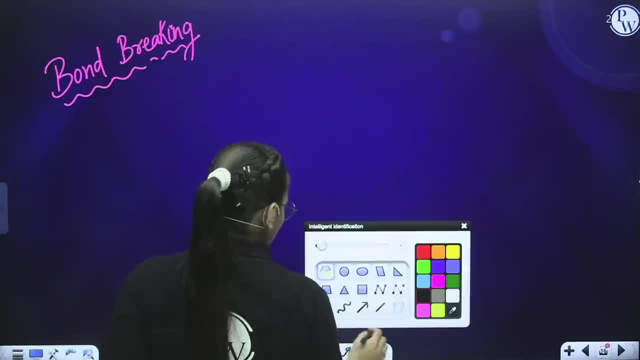 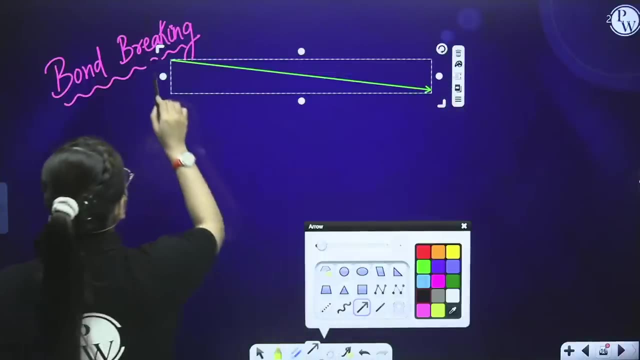 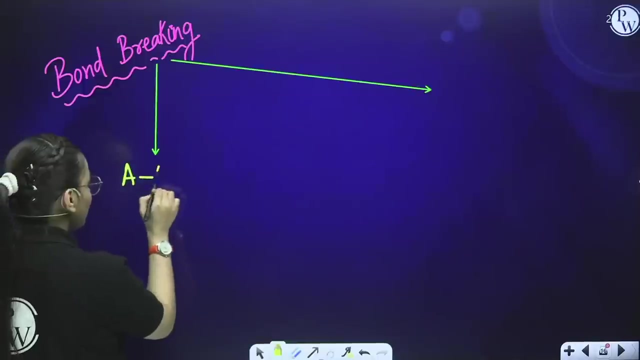 given to you. okay, see, when, students, you are given a bonded with a. this is the first case and the second case is going to be when a is bonded with b. now you are given two cases: when the atoms are same and when the atoms are not same. when the atoms are same, does electronegative 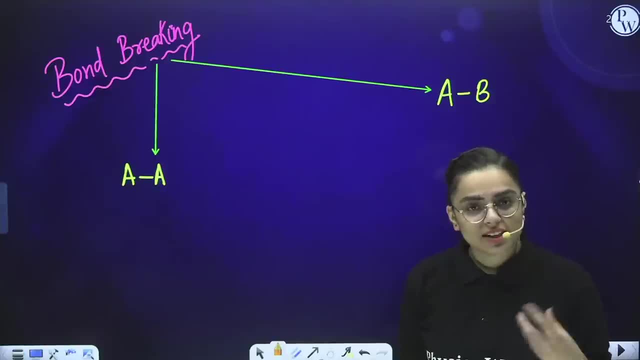 difference arises over here? no, why? because there are same atoms. so there is no difference in electronegativity, no difference in electronegativity. when there is no difference, electronegativity that means delta e- n is going to be zero. now, when there is delta e n is going. 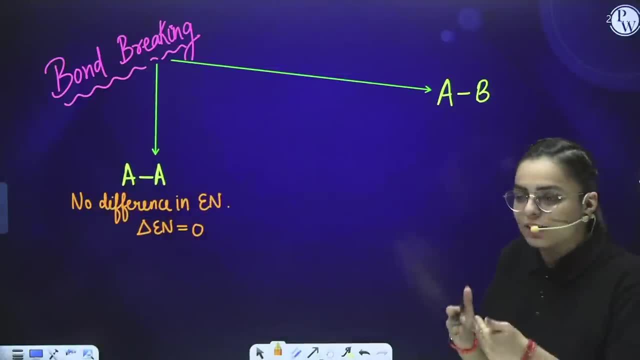 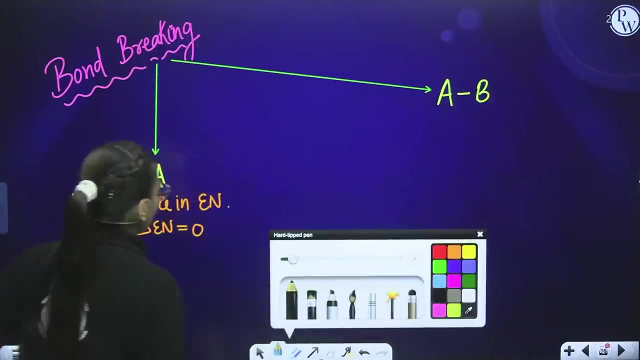 to be zero. that means there is no electronegativity difference. that means electrons are present in between. they are not shifted towards this more or that more. no, they are present in between. now, which kind of breaking arises over here? i say electrons are present in the center. most position like this. now, one thing you need to keep in your mind when they 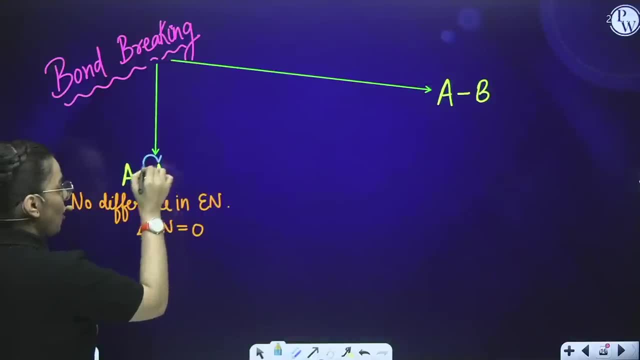 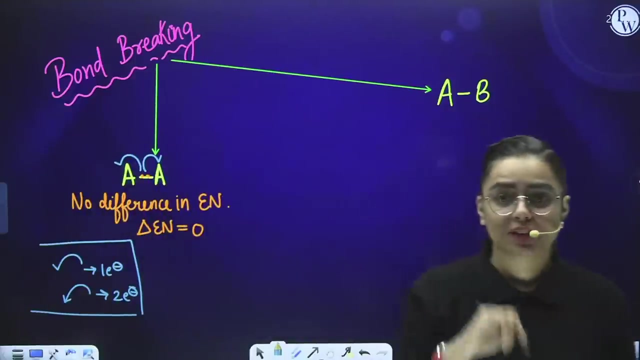 are equal electrons, then bond cleavage occurs over here in such a way. now what is this arrow? see, when i am representing this arrow, it is refers to as one electron. when i representing this full arrow, it is referred to as two electrons. now you should learn the movement of arrows also. we have seen the arrows of electronegativity. these are a kind 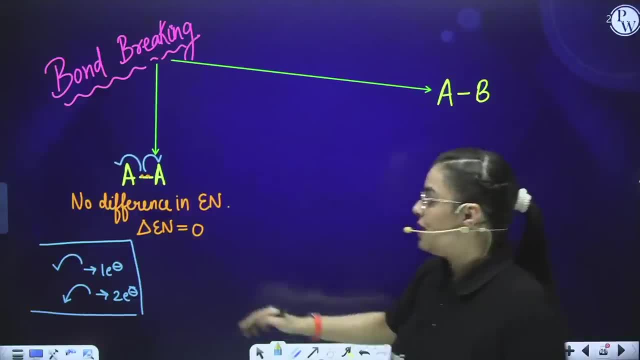 of different arrows. now, students, if i am talking about this arrow, it refers to as the movement of one electron towards this a and one electron towards this a. we know that a single bond contain two electrons. when we are doing a breakage of bond, that means we are dividing this bond into 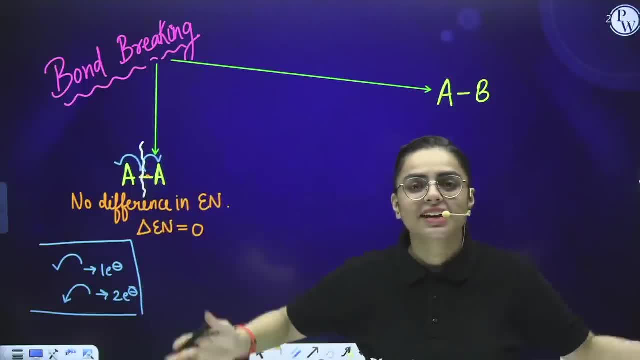 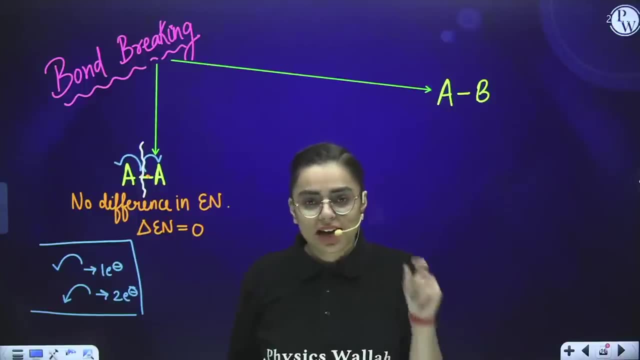 into such a way that a- a gets separate. now, if a, a are getting separate, both of the atoms are same. that means electronegativity difference is not there. so both of them will acquire one one electron. and when they acquire one one electron, we show this one electron by this arrow. now what will rise over? 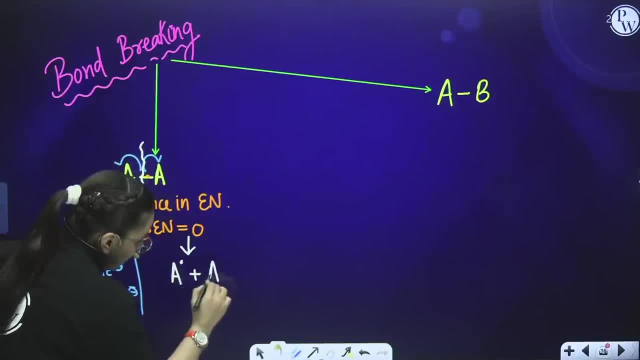 here a radical plus a radical. now this radical, this dot, is referred to as one electron. so this kind of cleavage, when we see same kind of atoms are present, it is known as homolytic cleavage or homolytic bond breakage. this is the very first kind which is homolytic cleavage, which is the very first kind which is homolytic cleavage. 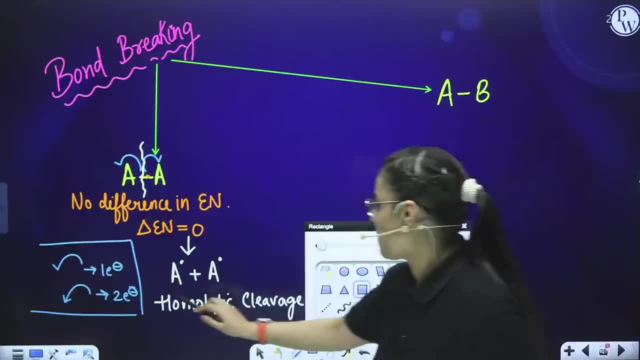 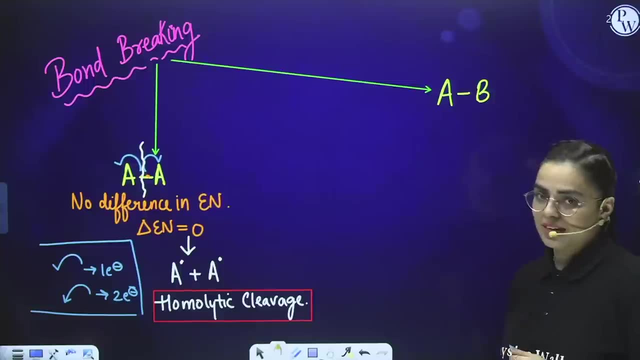 of a bond before a bond breaking. students, kindly put this in a box now. this was also a general concept that you need to keep in your mind. now comes the next case. if i talk about this case, i want this bond to be broken. now here, what do we observe? here we observe: 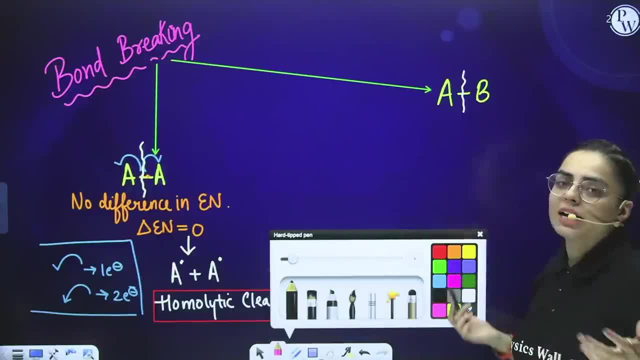 basically the electronegativity difference because there are different atoms. so yes, it is, but always there is an electronegativity difference. now, if i say there is an electronegativity difference, why? because atoms are different. collected gases are illegal. every atom is 주고. 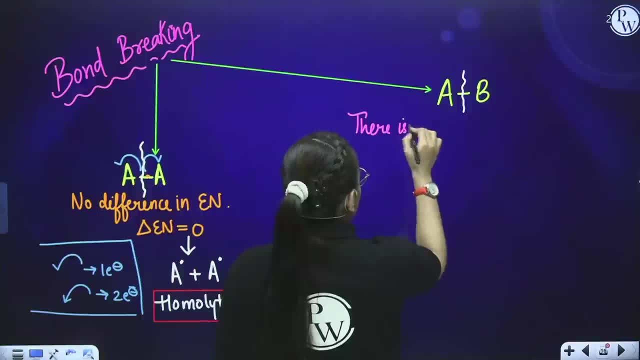 collaborated products which also have electronegativity, since if there is a đến, there are less electronegativity. difer comic policy if i say there is an electronegativity difference. why? because atoms are different objects, but also some같은. What makes you feel like you get a hundred electron. confident, that means you can dense all your atoms where you are finding them. 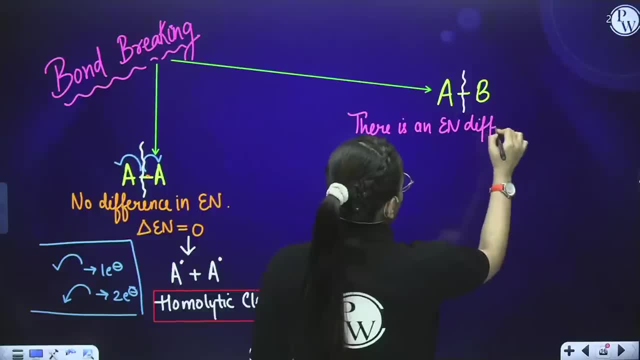 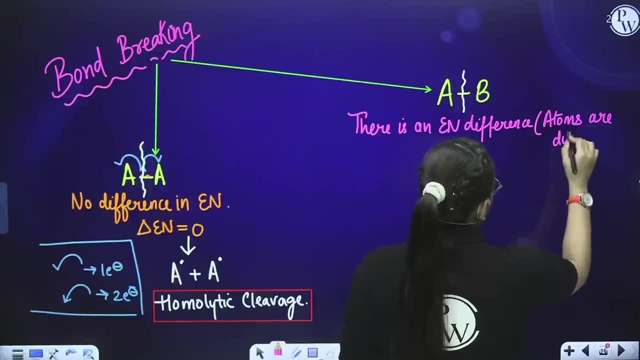 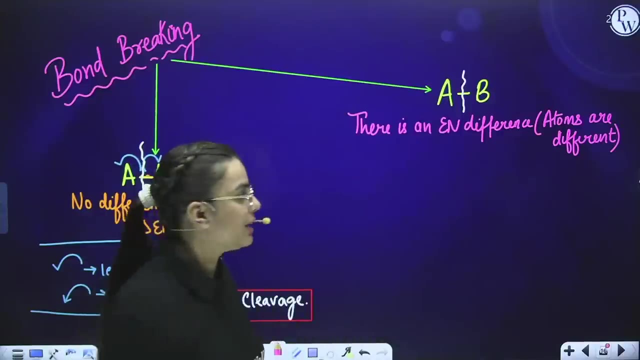 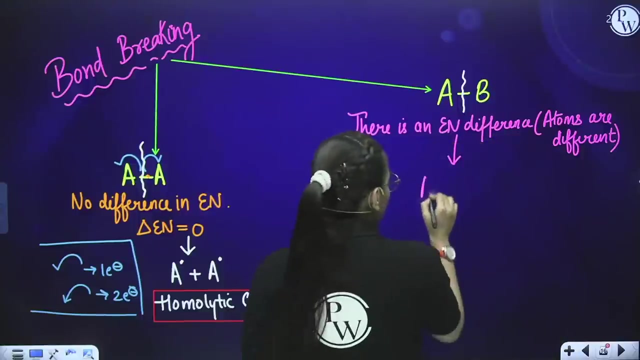 difference. why? because atoms are different. atoms are different. now if students atoms are different and if I say: let us assume B is more electronegative than A, what happens over here? if B is more electronegative than A, so here A will acquire positive charge and 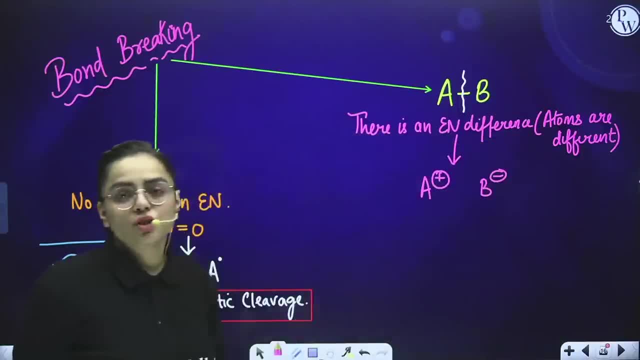 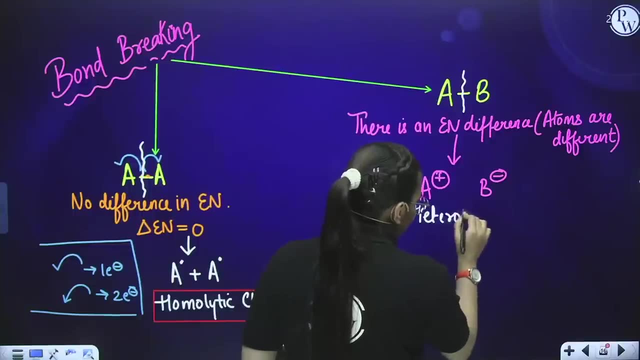 B will acquire negative charge. now, this kind of cleavage is known as heterolytic cleavage. this kind of cleavage is known as heterolytic cleavage. now, what is heterolytic cleavage? when two different atoms are present and the bond breaking process occur when same atoms. 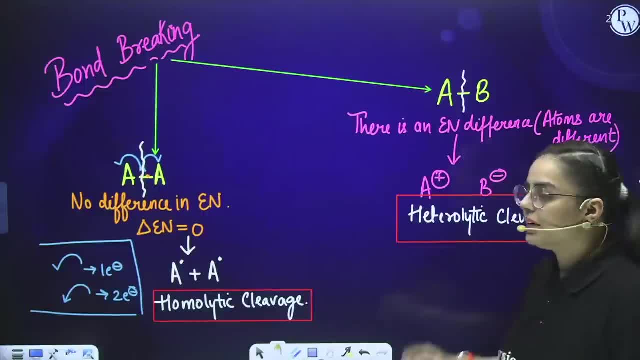 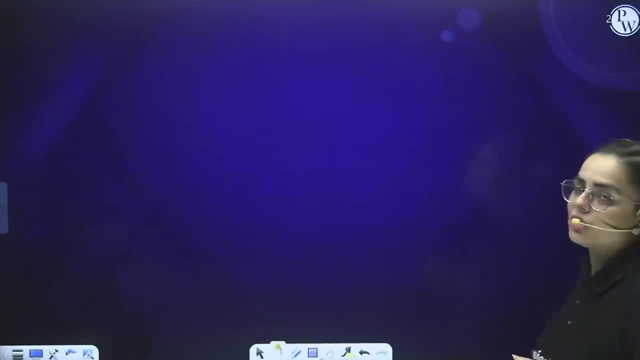 are present and the bond breaking occurs, that is homolytic. when two different atoms are present and, due to the electronegativity, bond breakage arise, that is heterolytic cleavage. now, students, comes our first application. that is stability of a reaction intermediate. 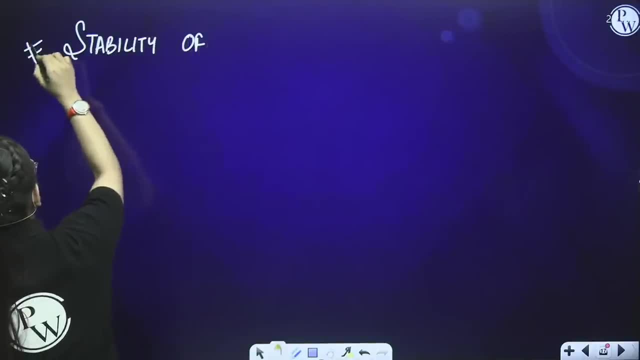 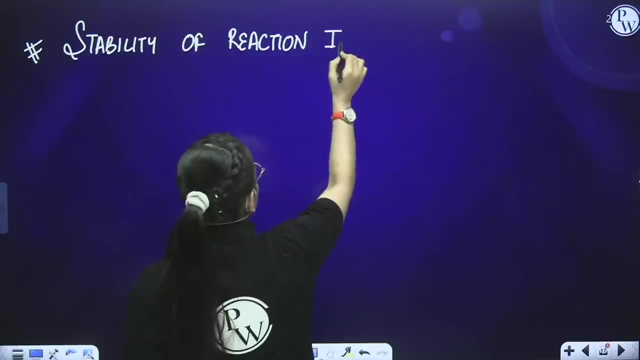 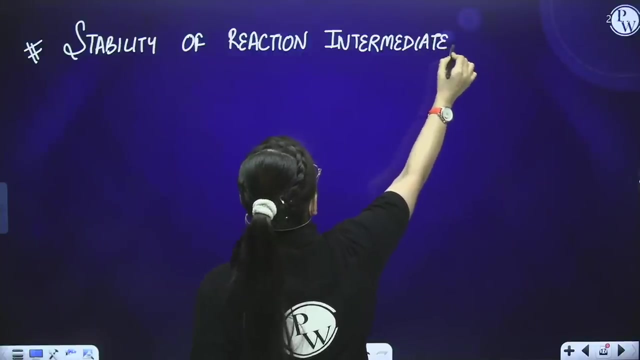 stability of this is, you know, the application portion of reaction intermediate. now, as I told you in the very first slides that, what were reaction intermediates? they were carbocations, they were carboanions, they were carbon free radical. we have understood this now here. 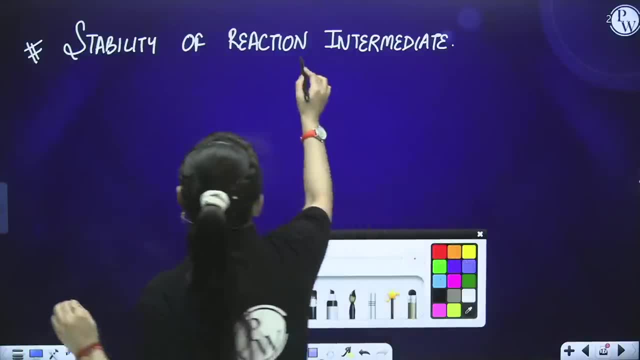 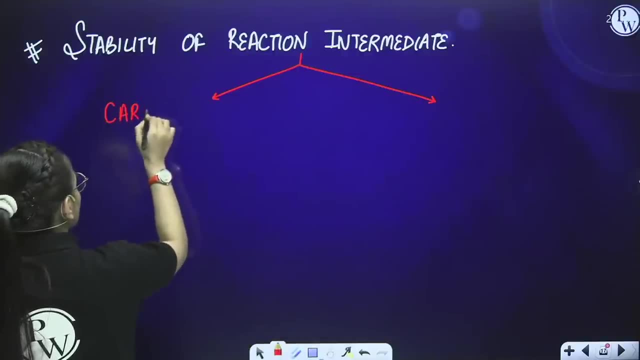 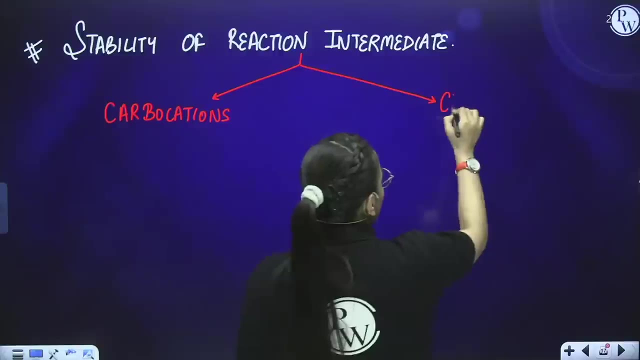 if I talk about the stability, we observe the stability in the case of carbocations as well as the carboanions. so what kind of stability do we observe if I talk about carbocations? the second one is carboanions. First of all, we need to understand what are carbocations. students. carbocations, if I split. 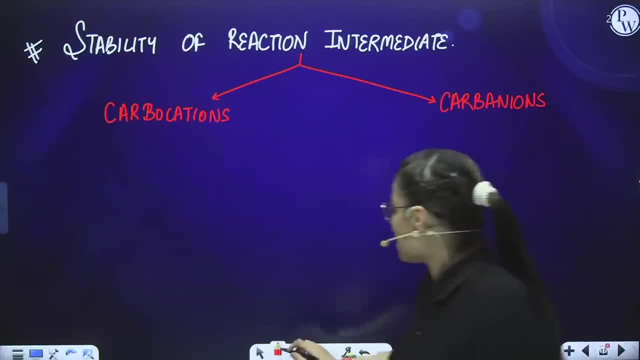 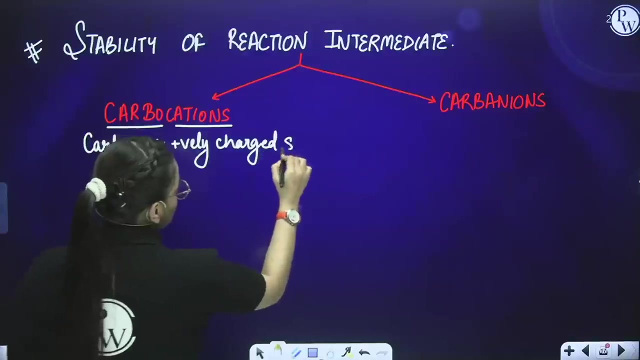 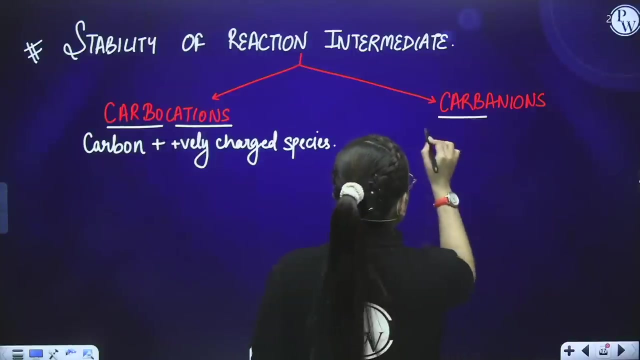 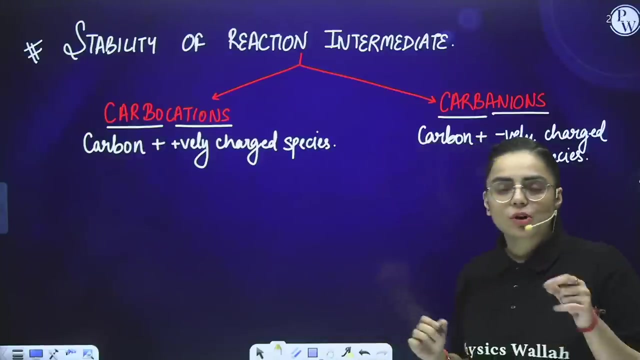 it into two types. it is carbon plus positively charged species. it is what It is: carbon plus cations refers to positively charged species, positively charged species. now, if I talk about carboanions, it is again what Carbocations: Carbon plus negatively charged species, negatively charged species. now, see, if I talk about carbocation. 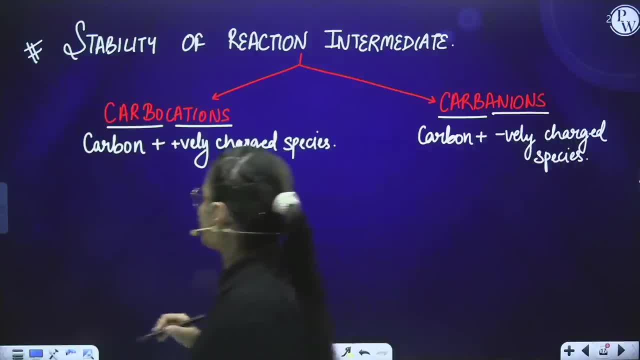 in detail. they are also known as carbonium ion. they are also called carbonium ion, also called carbonium ion- clear, Clear Now, students, if I talk about carbocation in detail, let us take an example. how does carbocations are formed? if I take a general example, I would say, for example, if I have CH3F now 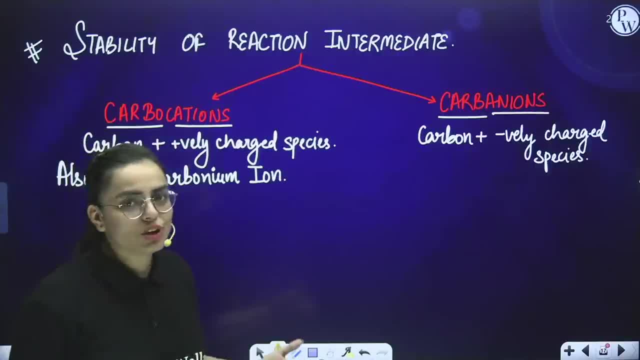 we know that carbon is bonded with fluorine and we know that fluorine is more electronegative than carbon. now, what does occur over here? heterolytic cleavage. we get CH3 positive and F negative. why? because there is a difference of electronegative over here, difference of 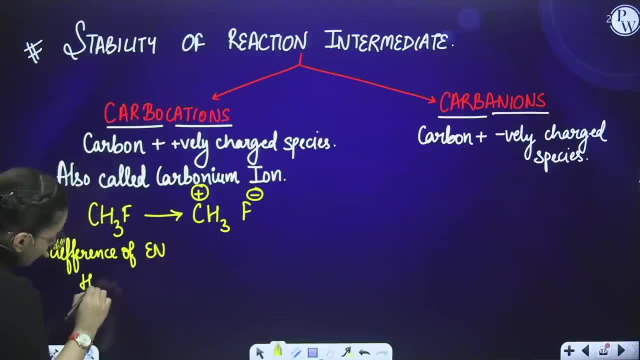 electronegativity occurs here. heterolytic cleavage occurs, as fluorine is more electronegative than carbon. so fluorine acquires partial negative charge, and carbon acquires partial positive charge. so again carbon plus positively charged species. that means here CH3. is what 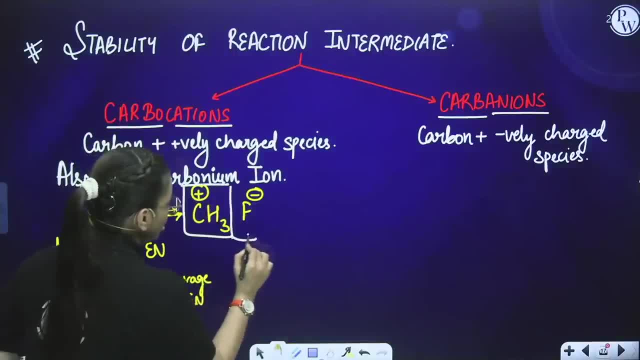 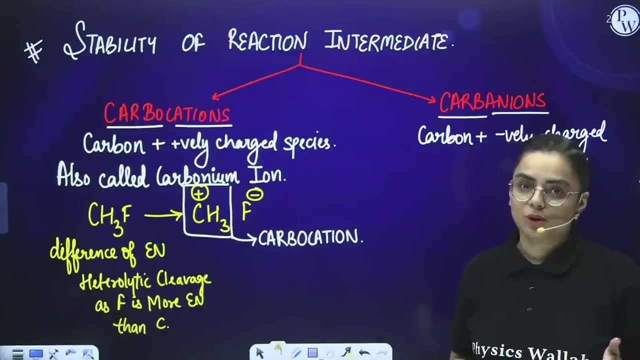 Here this CH3 is what CH3.. Here this CH3 is carbocation. here this is carbocation. students. now what carbocation is basically? what? here we are seeing heterolytic cleavage, and how is the structure of carbocation? Basically, it is electron deficient species. how, I would say it is electron deficient if. 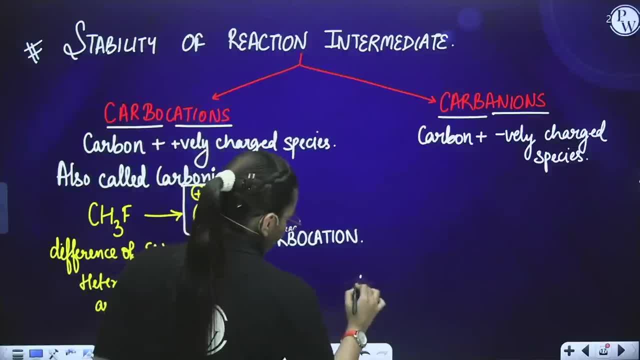 I talk about its structure over here. let us see, this is carbon. okay, now this is hydrogen. I have. this is hydrogen, this is hydrogen, This is hydrogen and this we have the positive charge over here. now this is the structure for carbocation. this is the structure for carbocation. it is electron deficient species. 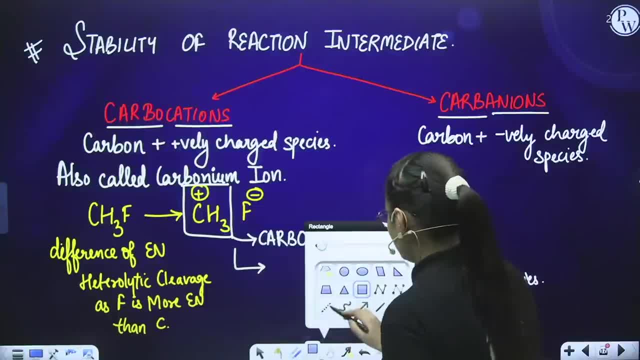 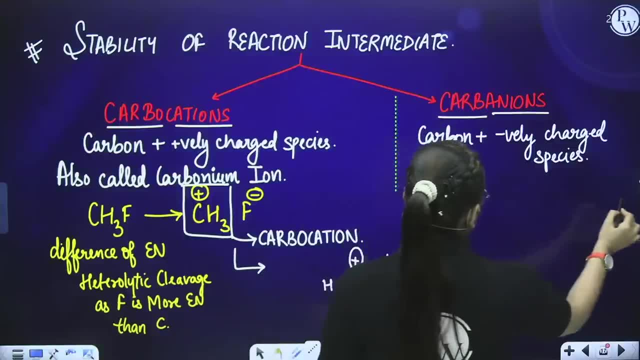 it is electron deficient species. kindly put a line over here so that we do not get confused between carbocation and carboanine. we do not get mixed both of these, right, okay? Okay, students, so now you can see. carboanine we will discuss in the next slide in this. 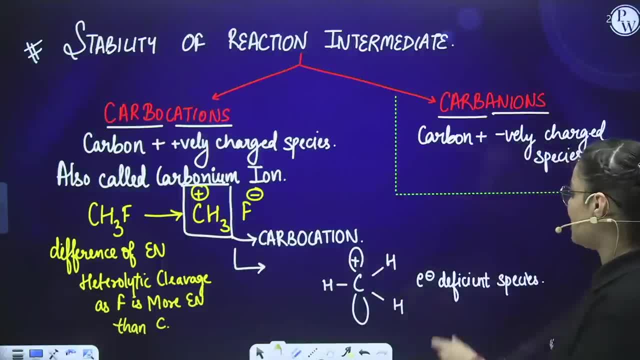 slide is all I am telling about carbocation. this is the structure for carbocation. it is electron deficient species. how many electrons are present over here? You can see that here basically there are 6 electrons present. it is sp2 hybridized. 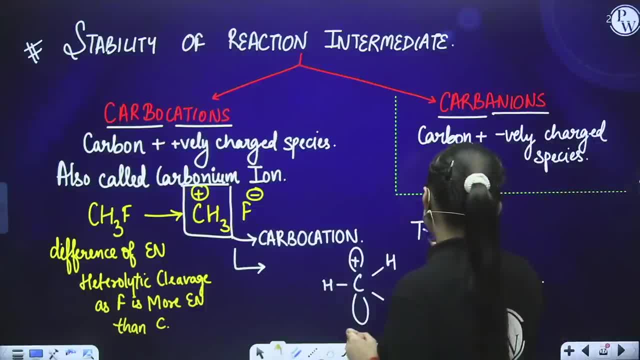 students. and it is trigonal planar. it is trigonal planar sp2 hybridized with sp2 hybridized. okay, Okay, Okay, So this is 6 electrons, because it is electron deficient, hence it is 6 electron species. 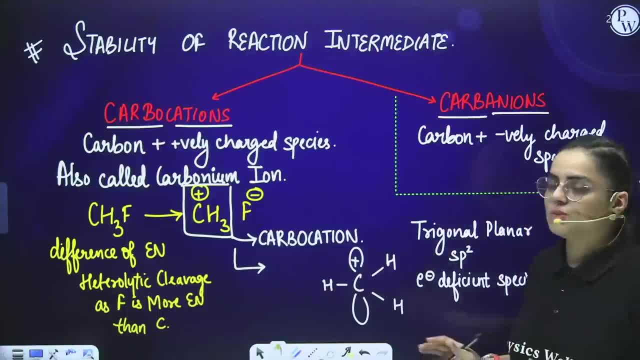 Now, who will attack over this? as it is electron deficient species, nucleophile will attack over this, because nucleophile will have more electron density. Now coming towards what carboanine? this was all about carbocation, which is the one which is having positively charged species, also known as carbonium ion. 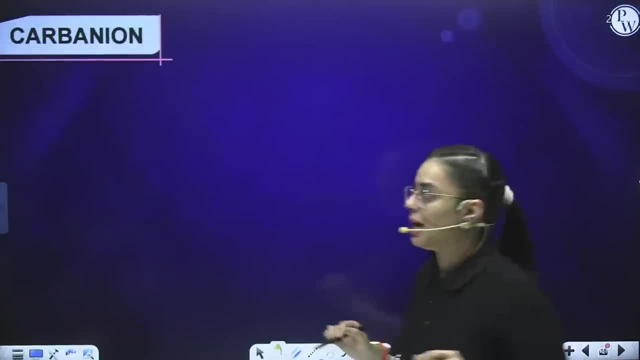 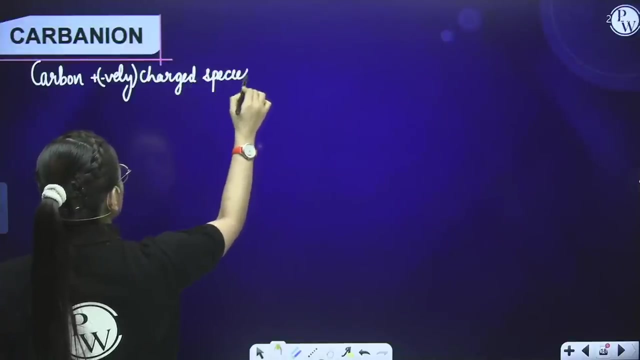 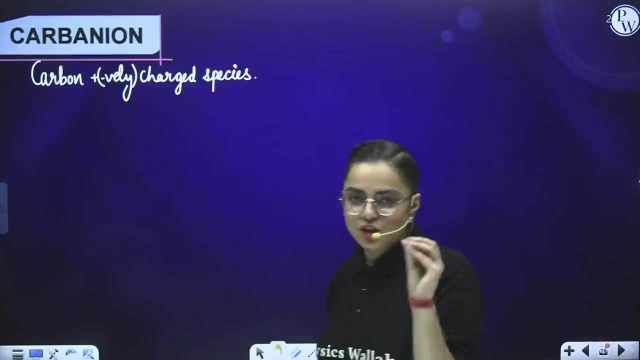 Now, if I talk about what? if I talk about carboanine, this is again carbon plus. carbon plus, This is a negatively charged species. negatively charged species, this is what is carboanine. Now, if I talk about carboanine, let us take one case, like I took CH3F here. let us say: 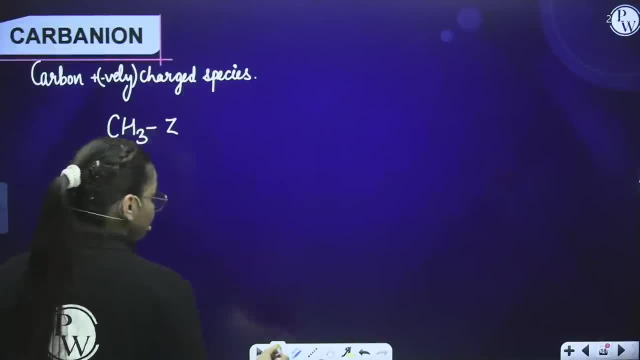 CH3Z. now I would say that this Z, it has less electronegativity than carbon. now, if it has less electronegativity than carbon, what do we acquire over here? again, heterolytic cleavage, because there is a difference in the electronegativity carbon has, now more. 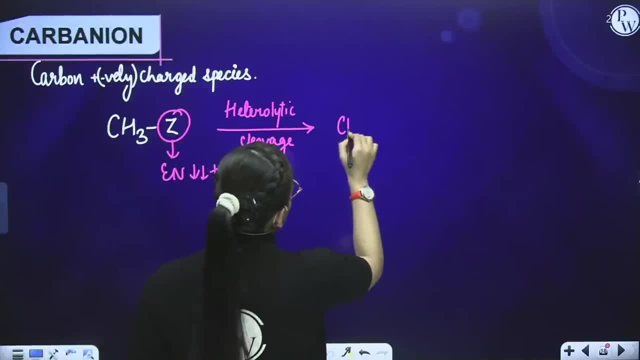 electronegativity than the Z group. So if it has more electronegativity, then will we have CH3 negative plus we will have Z positive with us, Dear students. now what is CH3 negative over here? this CH3 negative is carboanine. this 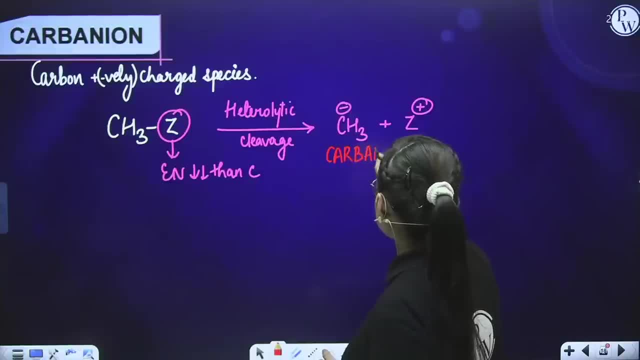 is. this is carboanine. Okay, Okay. So what is carboanine? now let us talk about its structure. so how does it looks? it looks like this: This is the structure for carboanine, which is basically what, which is basically tetrahedral. 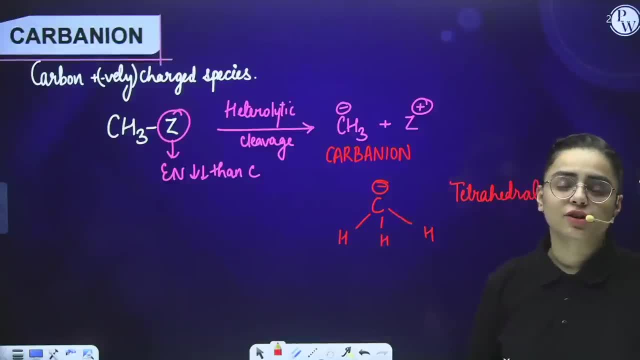 Now, if you kind the electrons 1,, 2,, 3,, 4,, 5,, 6 and you have 7, 8 electrons, it is electron rich species. it has electrons, 8 electrons. it is electron rich species. 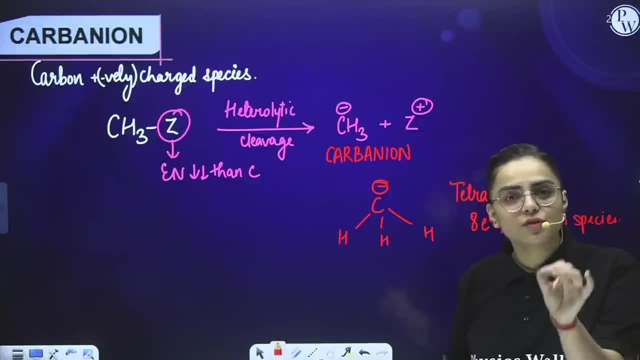 So who will attack over here? electrophile will attack over here. do not get confused about nucleophile. electrophile we will cover in the upcoming topic. So just I want you to understand the difference between carbocutine and carboanine. 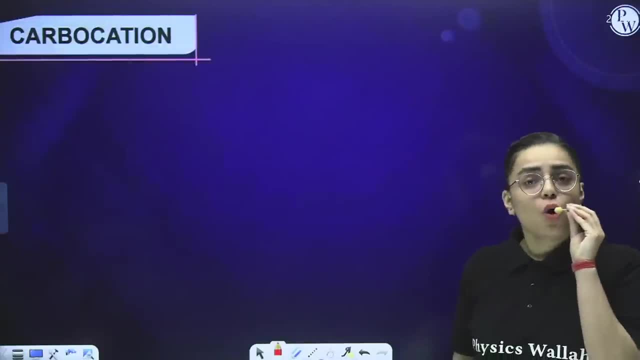 Okay, Now, if I talk about the carbocutine, the order of carbocutine, the stability, because we have seen the plus I effect, basically defines us about the carbocutines we have seen. we have seen this case. 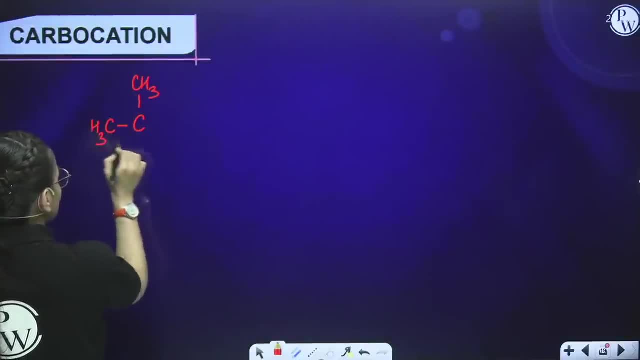 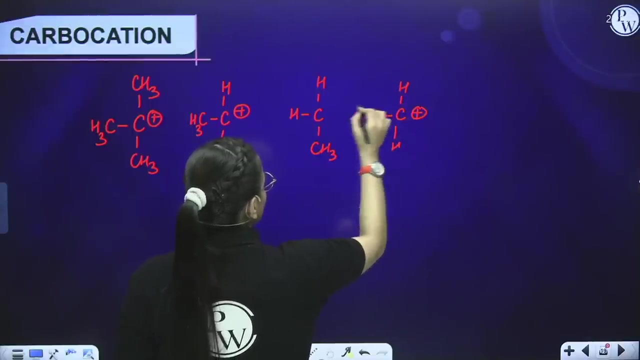 See CH3, CH3, CH3.. Okay, Okay, Okay, CH3 positive. Then we saw this case: CH again is CH3, again is CH3 positive. Then we have CH H, CH3, and the last one is CH H H positive, positive. 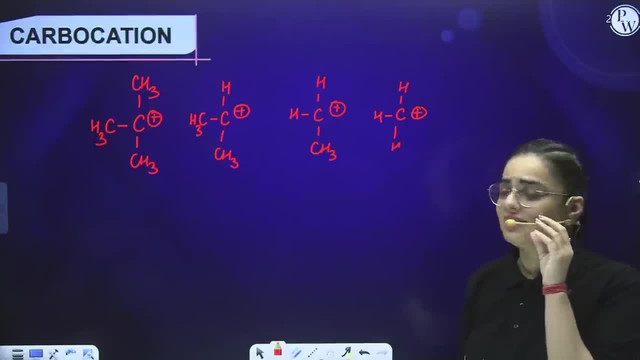 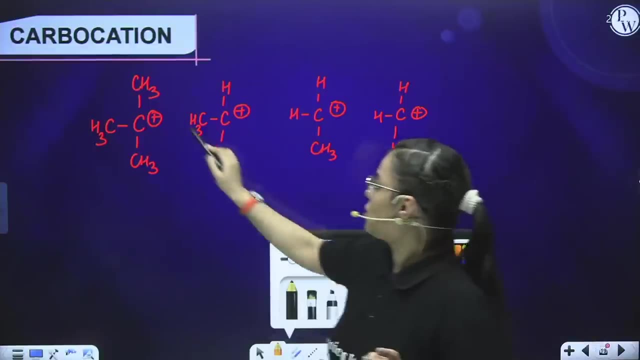 Now for these carbocutines, which will be more stable. we have already seen this case, students. we have already understood this case. How we have understood this case. Okay, here i would say, the order is going to be this: you remember, plus i effect in plus i. 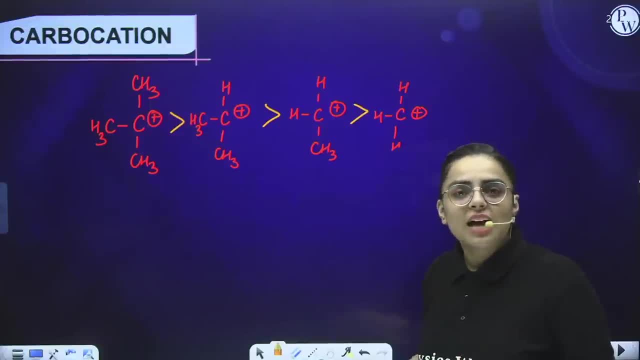 effect what i told you. i told you this order to remember. so these were carbocutines. this is three degree carbocutine, then two degree, then one degree. you need to remember in your minds that three degree carbocutine is more stable than two degree, then one degree. this. 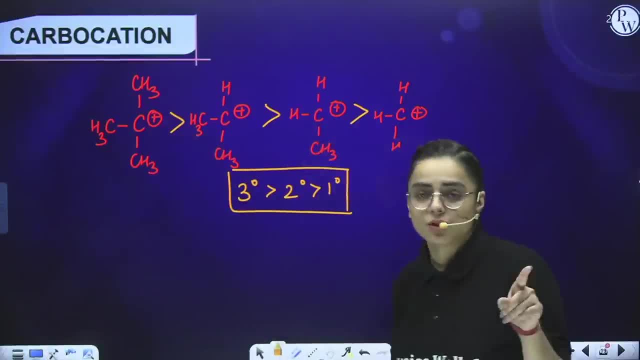 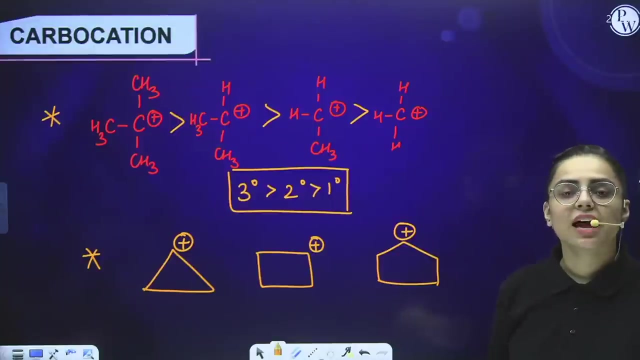 i am talking about carbocutines, not carbon ions. don't get confused. now if i talk about a ring like structure, this was the first case that you need to remember. okay now students. for example, if you have this kind of structure, which will have more, you know stability for this carbocutine, so i would say the small ring will have more. 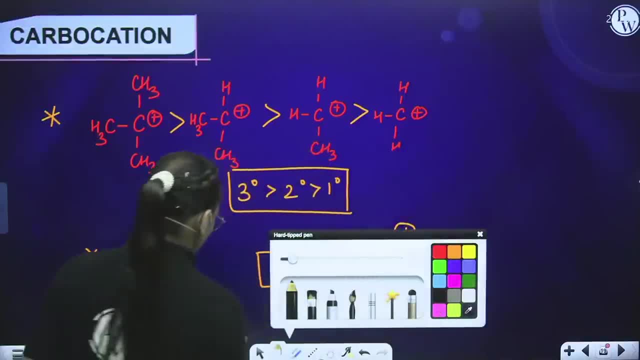 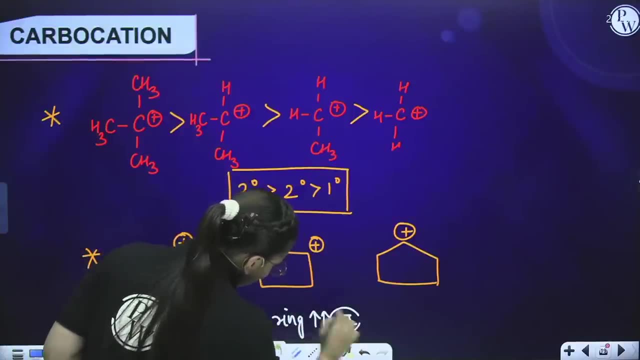 minus i, the small ring will have more minus i. now, if it has more minus i, that means the large ring will have property of minus i, with the small ring which is greater than minus i, and if it has this quantity, which i this accurateGA, we can write it, you know. 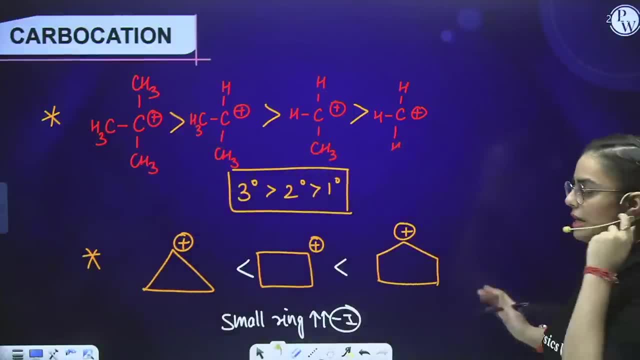 ring will have the plus i effect. so this is going to be the order. this is going to be the order. other than this, whenever you are giving any of the compound, kindly find out if it is 3 degree, if it is 2 degree or 1 degree. if it is 3 degree, it will be stable. then 2, then 1. this is a general. 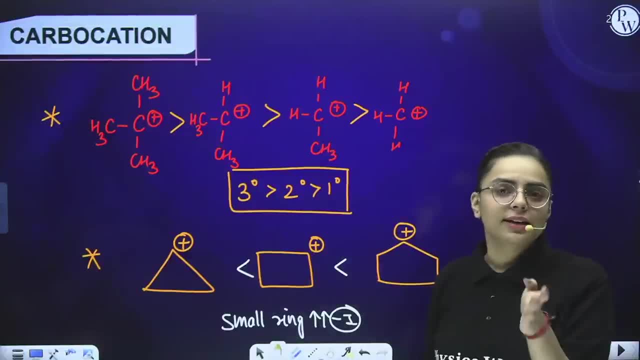 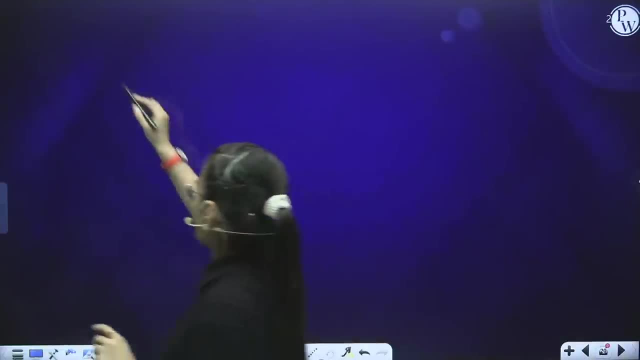 case other than this. you can get many cases, but you need to find 3 degree, 2 degree, 1 degree. that will be your answer right now, students. if i talk about the next, for the carbo anions, if i talk about carbo anions, the order is: 1 degree is more stable than 2 degree, and then 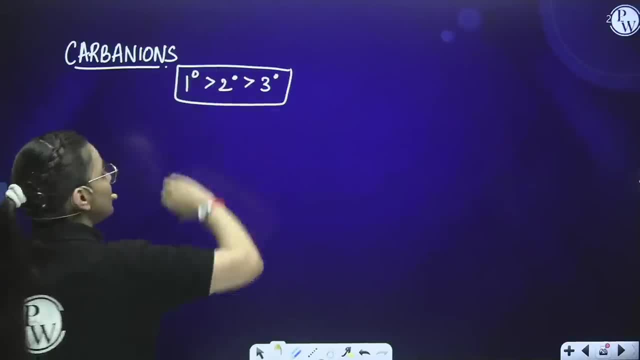 3 degree for carbo cuttings. what do we observe? we observe that 3 degree was more stable than 2 degree, than 1 degree. here, 1 degree is more stable than 2 degree, than 3 degree. now let us make the structure for these also. this is our 3 degree. it acquires negative charge. then is our. 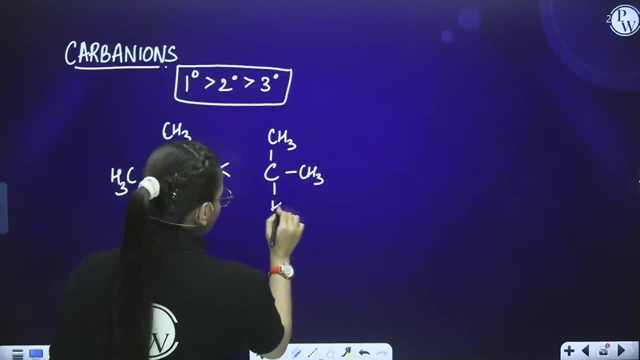 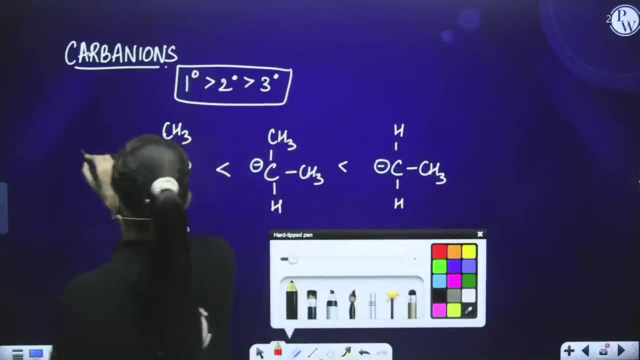 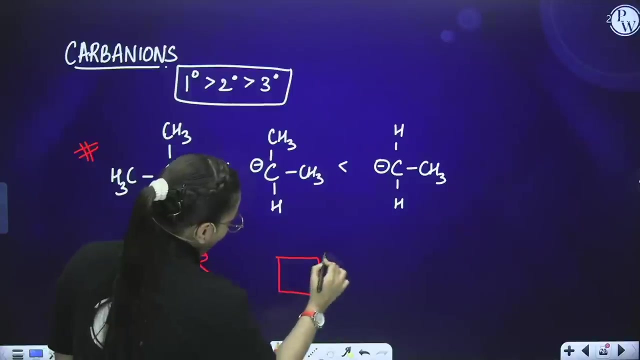 2 degree degree and then is 1 degree. So 1 degree is going to be more stable than 2. then you know the 3 degree. If I talk about the ring like structures over here in this, this was the first case. 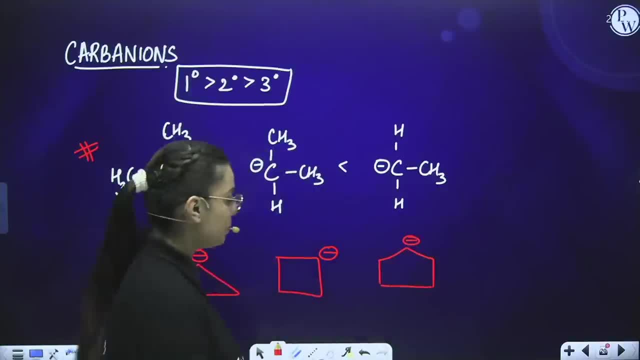 So, as I have already told you, for Carbo 9- the small rings, one will be more stable. So this is going to be the structure. This is going to be the order. Now for Carbocatines, the larger rings were stable, not the smaller ones. 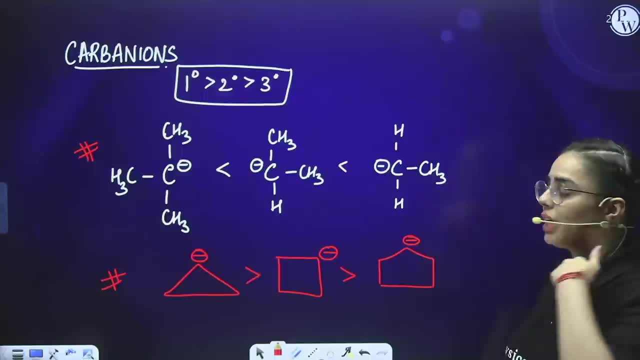 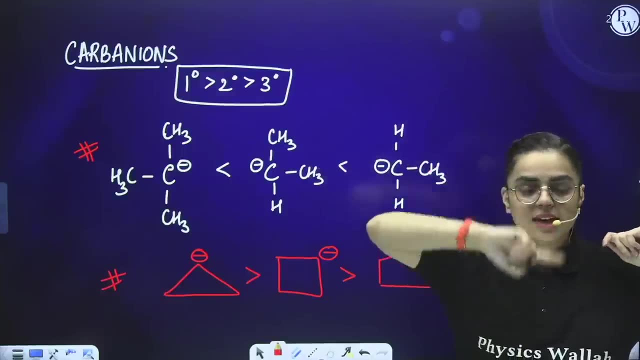 For this, smaller ones will be stable and then the larger one. Other than this, if you acquire any question, kindly find out: 1 degree, 2 degree, 3 degree, then apply this concept: 1 degree will be more stable for the case of Carbo 9, then 2 degree. 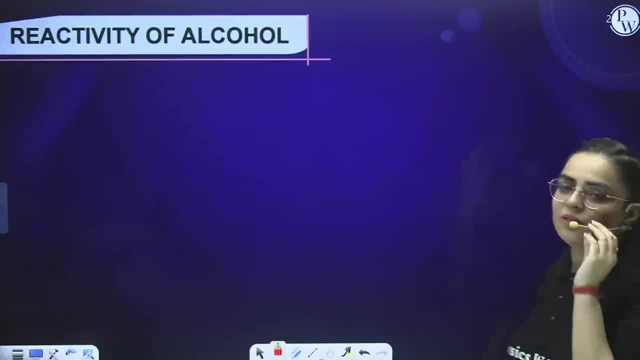 then 3 degree, Now come students. our next topic, that is the reactivity of alcohol. This is also one kind of application in inductive effect For the reactivity of alcohol. What kind of questions arise over here is acidic strength. What arises over here is acidic strength. 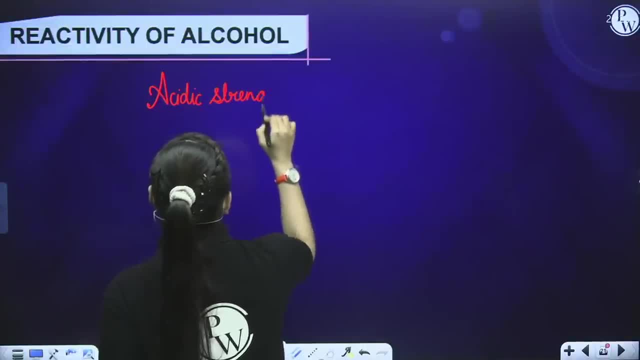 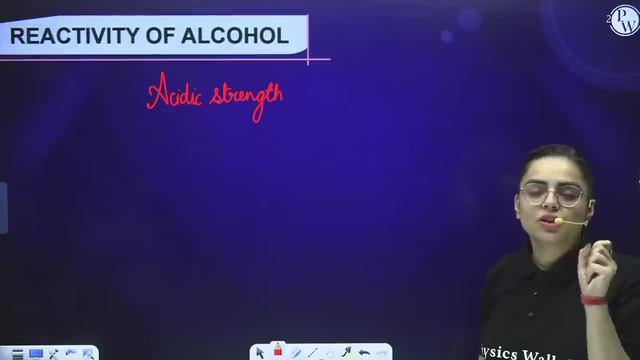 They ask you about acidic strength. So when they ask you about acidic strength, see, you know 2 kinds of effect. 1 is minus i, 1 is plus i. Whenever you need to find acidic strength of any of the alcohol, acidic strength is directly proportion to minus i groups. 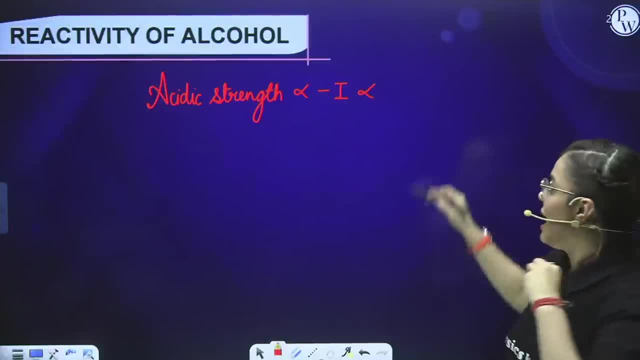 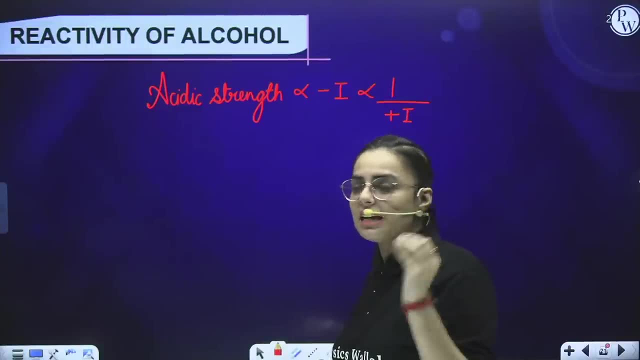 The one- those who are having minus i groups will have more acidic strength, and the one which will have the plus i group, they will have less, Because Acidic strength is inversely proportional to plus i, but directly proportional to minus i. So this is the order that you need to keep in your mind. 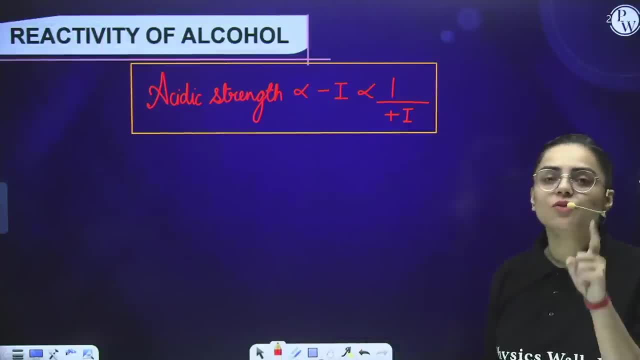 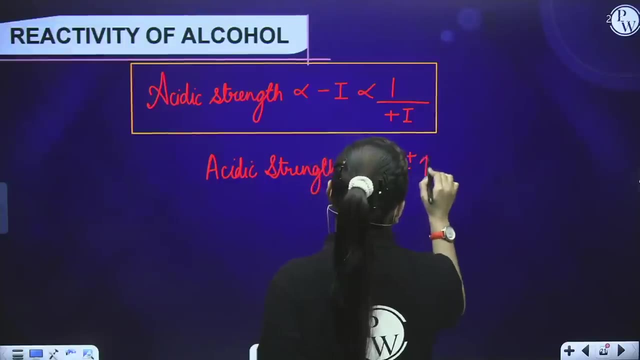 Okay, this is the first order that you need to keep in your mind, and when, whenever you have calculated acidic strength, do remember acidic strength. if acidic strength is more, then more H positives are produced, More H positives are produced, And if more H positives are produced, 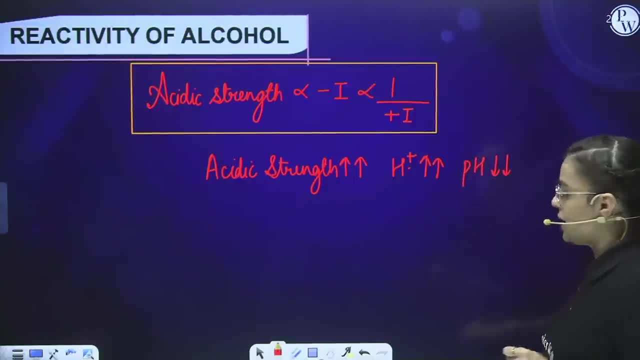 Then pH is going to decrease. less will be the pH, more will be the H positive, less will be the pH, more will be the Ka. more will be the Ka, less will be the pKa, less will be the pKa. So this is all what you need to remember in the reactivity of alcohol students. 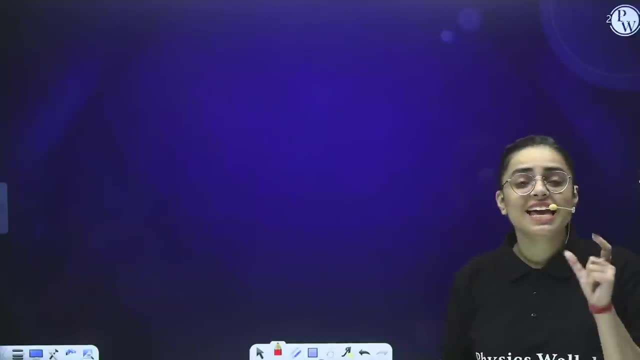 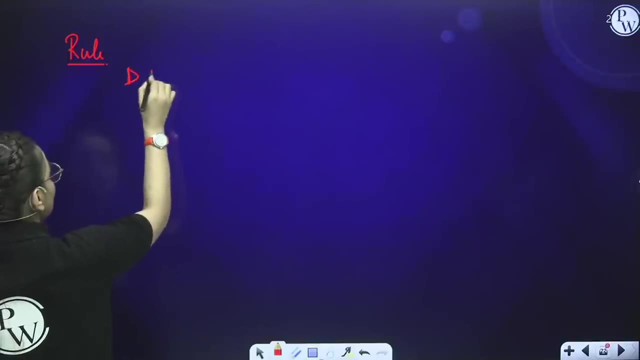 Now coming to the next rule that you need to keep in your mind is DNP rule. Next is rule that you are- you will see in the questions- that is DNP rule. This is DNP rule. other than this, Other than this, reactivities. 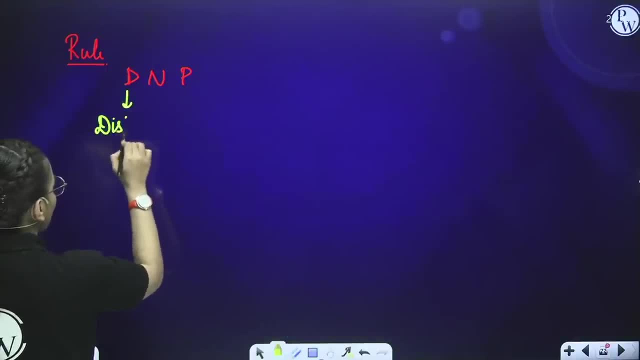 Now, what do you mean by D? D is distance, N is number and P is power. P is power. So the order comes in this direction only. First of all you will see distance, then you will see number, then you will see power. 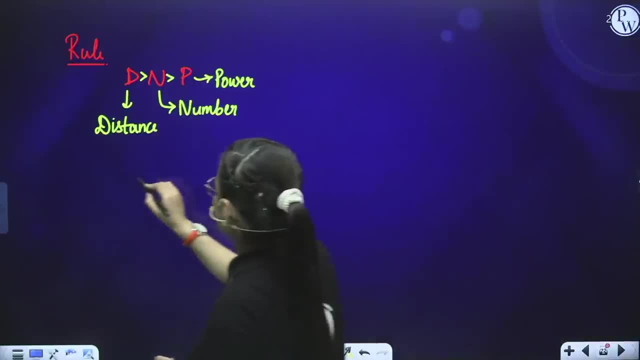 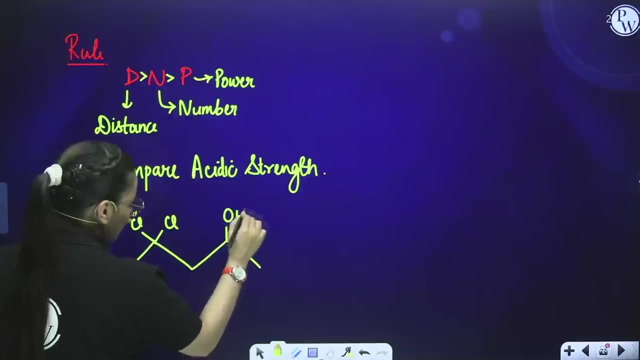 If I talk about comparing one question, if I give you question over here, Compare, Compare acidic strength, compare acidic strength, and if I give you one single case in which, for alcohols only, for example, I'm giving you: okay, now, students, this is the question which I have given you, this is your. 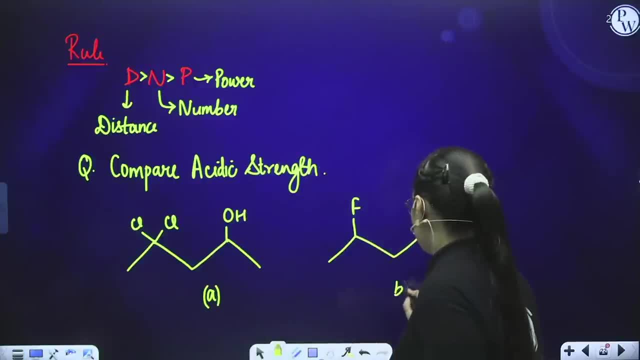 a. this is your b. now kindly tell me which will have more acidic strength. you will say, ma'am. first of all we need to see the distance. distance refers to at what distance of the group is the another group lied. see, oh is present over here. so cl is lied after one carbon. 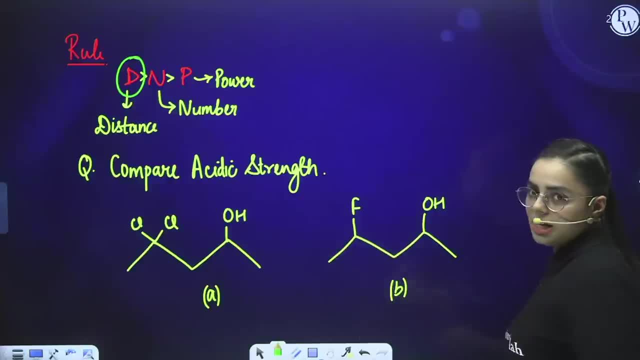 after one carbon to the other carbon. so distance is equal for both of the case. here is which, here is which. then comes one carbon, one carbon, then comes carbon, then comes carbon. it have fluorine, it have two chlorines, right, so distance is same. distance is same. over here now let us talk about what, talk about number. how many fluorine? 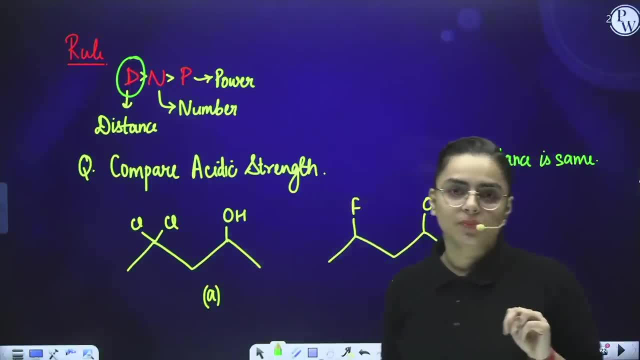 atom? one fluorine atom. how many chlorine atom? two chlorine atom, how many? two? you know, fluorine, chlorine bromine had which group minus i group? so this is minus i group. we know that even chlorine will have minus i minus i, but we are talking about number. how many here is? 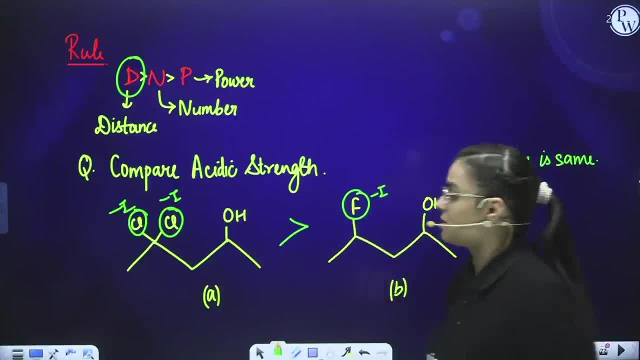 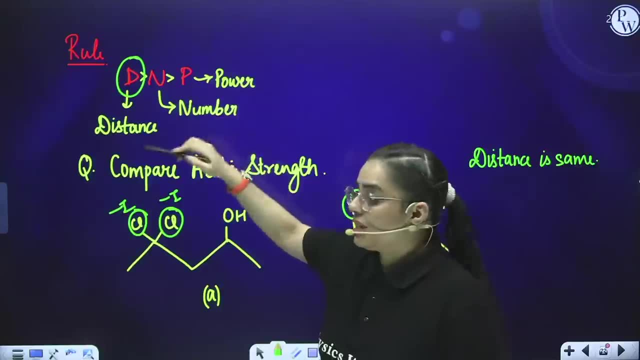 one, here is two which have more. this has more. so the acidic strength is this: it does not, has not depend that you know fluorine will have minus, i more no. first of all check dates, lass, then check number. if number same, then move towards the power power refers to as 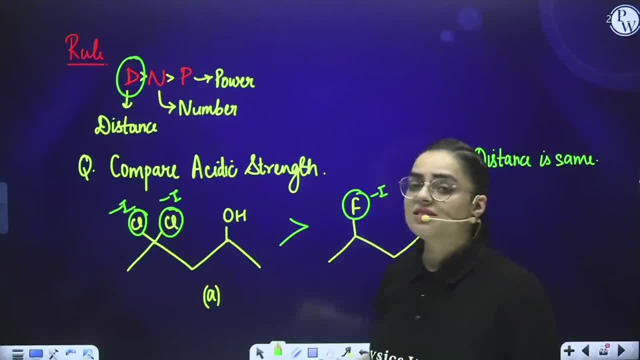 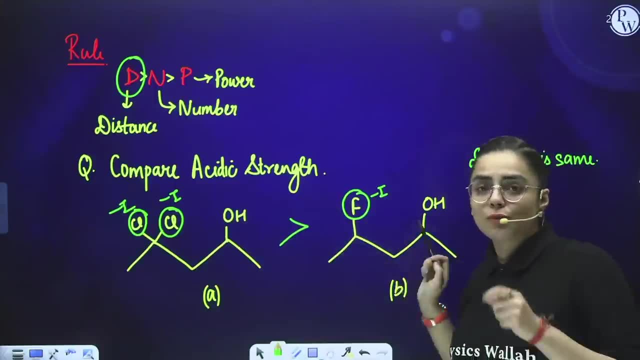 plus I, minus, i jam. first of all check distance them, check number them, check this that this has more i. if they had a same number, no students, if they had one cooker, one floor in, then this would be correct because chlorine is more. chlorine has more minus high light. but first, 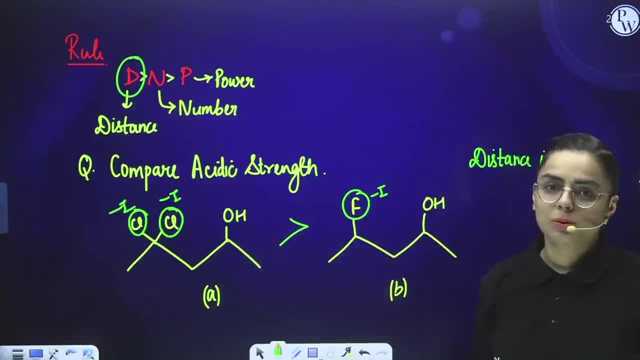 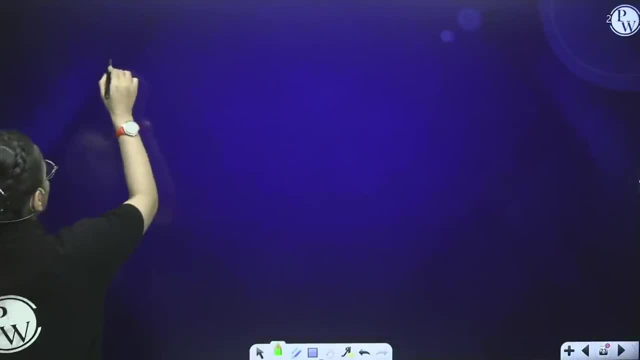 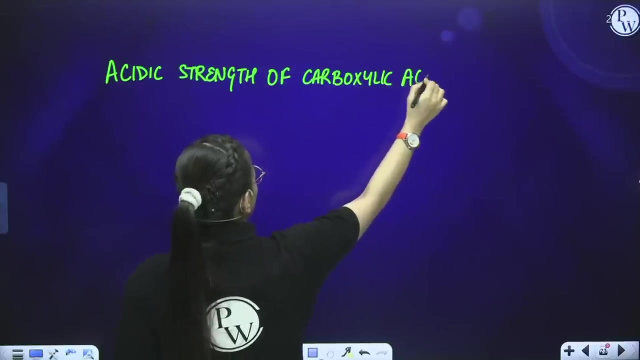 of all distance. then comes number number. here is two chlorine, here is one flowing. so it will be now. if i talk about one more case, let us talk about acidic strength for carboxylic acid. do remember one more thing: in the previous case i have already told you here. 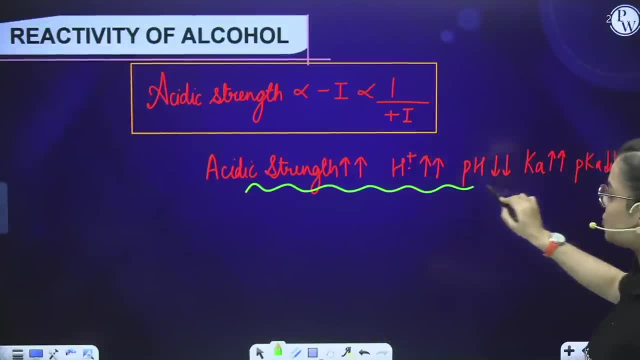 this order. if they'll ask you h positive order, ph order, ka order, pk order. kindly calculate acidic strength. h positive will have same order, ph will have the opposite order. because it decreases, k will have the same order and pk will have the opposite order. clear. now coming back to my this: 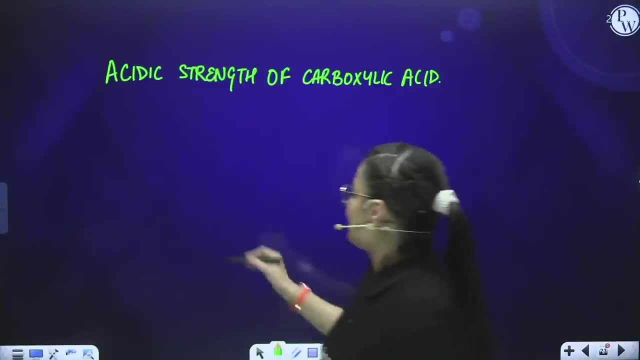 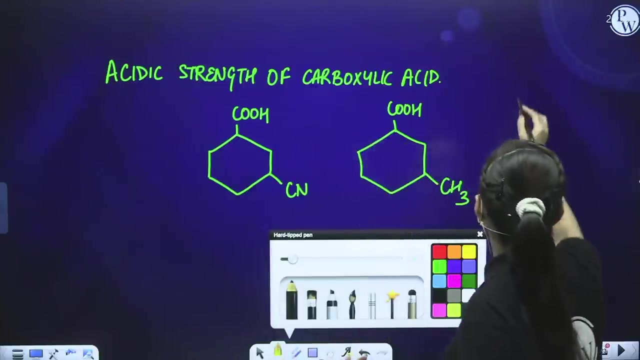 question of the carboxylic acid. i have now two groups with me, for example. i say you, here is cyanide group, here is methyl group, methyl or i would say ch3, methyl is basically ch3. but i'll write directly right now, students, again, what we are going to apply over here. we are going to apply the dnp. 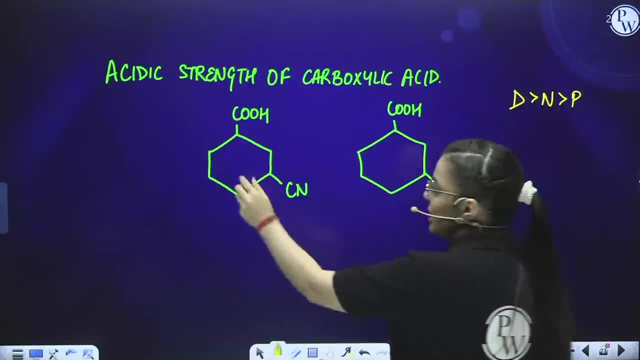 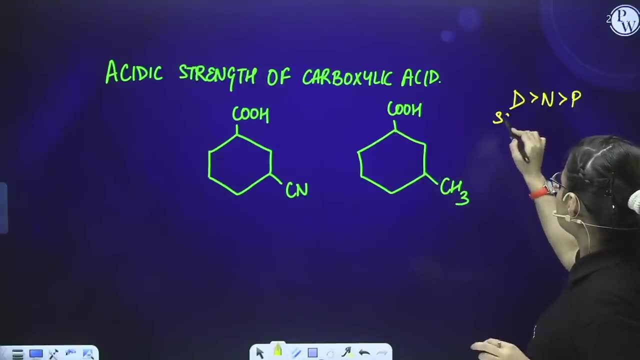 roll. first of all check the distance from the carboxylic acid after one carbon to another carbon. it is c, and after one carbon to the another carbon. it is ch3. distance is same. distance is same. now come towards number 1cn, 1ch3. same again. now here, number is also same. 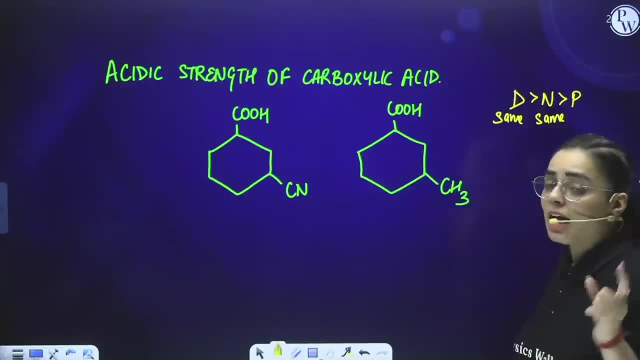 1cn, 1ch3. one is you know, one is CH3, now remember, CH3 has which group, CH3 has which group. It has plus I group and CN has what Minus I group. so here, acidic strength. we know that acidic strength is. 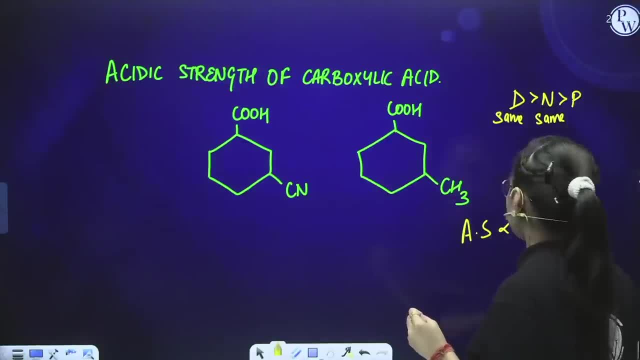 directly proportion to minus I and inversely proportion to plus I. so minus I will have more acidic strength. clear, As you know, CN has minus I and that's why clear students. So in such kind of situations you can do the acidic strength, you can calculate the acidic strength. other than this: 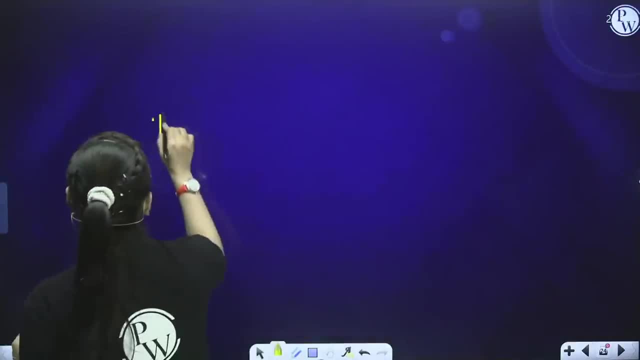 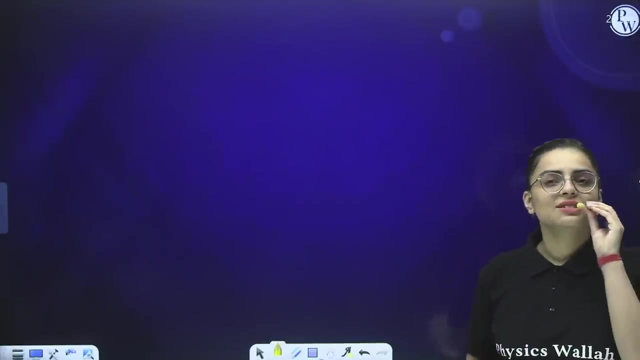 basicity question arises. so basically, basicity for gaseous phase is directly proportion to plus I groups. acidity is inversely proportion to plus I group acidic strength. but basicity is directly proportion to plus I groups. okay, students, Now comes the stability of carbocations. if I talk, 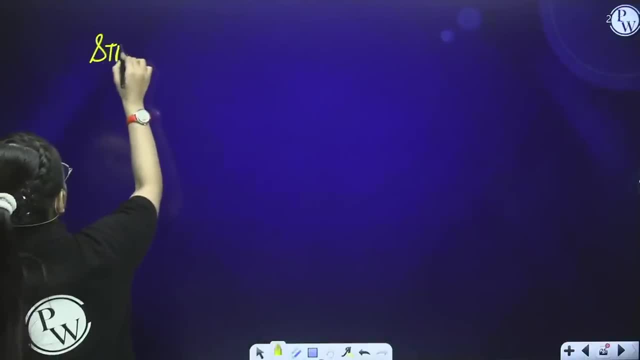 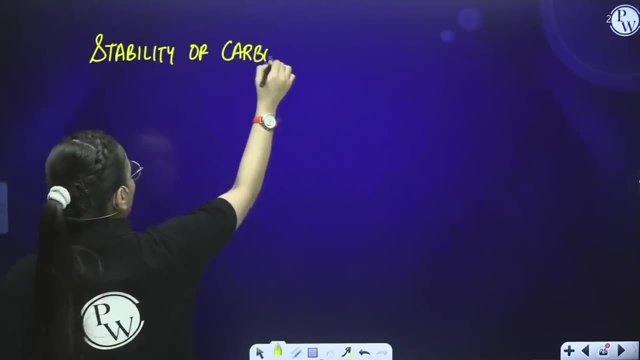 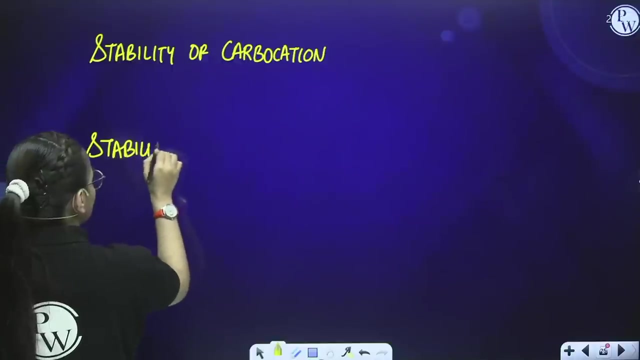 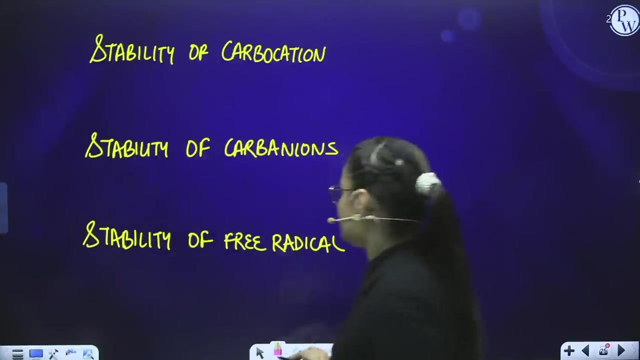 about stability of carbocations. I'll write three of the cases over here. then comes the stability of carboanions and then comes the stability of pre-radical. so if I talk about all of four of these cases, see if I talk about stability of carbocation. 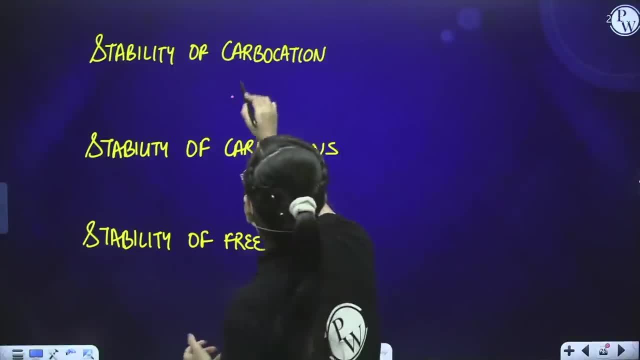 stability is directly proportion to plus I group here for carbocation, stability is directly proportion to plus I and inversely proportion to sorry and inversely proportion to minus I. if I talk about carboanion, it is the opposite order. stability is directly proportional to minus I and inversely proportional to plus I. now, if I talk, 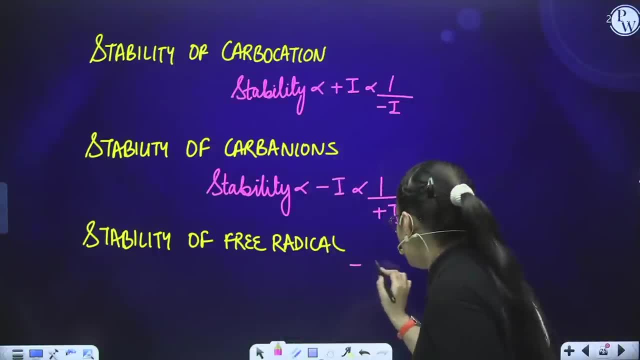 about stability of free radical. now, what is free radical? carbon containing one electron, this is free radical. now, if i talk about this, it is same as that of carbocation. the order is same. this one same as of carbocation, clear students. so here you have seen the application. 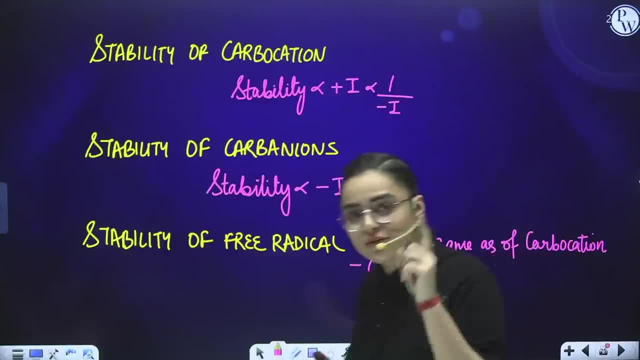 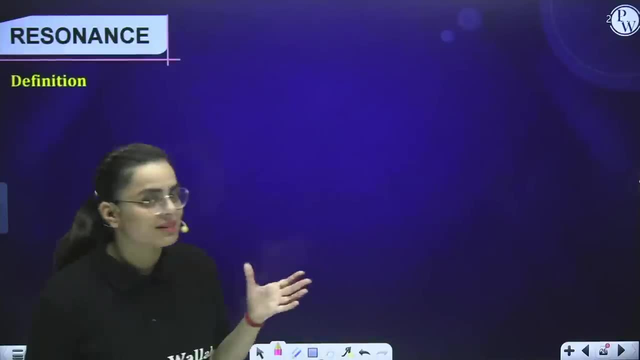 portion of you know, inductive effect. this was the very first effect, permanent effect. under the category of what? electronic displacement. now we will move forward towards our next kind of effect, that is, resonance effect or mesomeric effect. but before understanding resonance effect or mesomeric effect, we need to understand what do you mean by resonance? 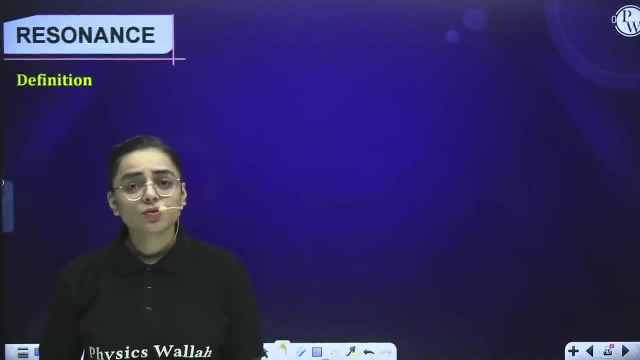 so, students, as we were understanding about resonance first of all, i would love to tell you that if we need to understand mesomeric effect, first we need to understand about resonance. then we will move forward towards the mesomeric effect and we will understand the difference. 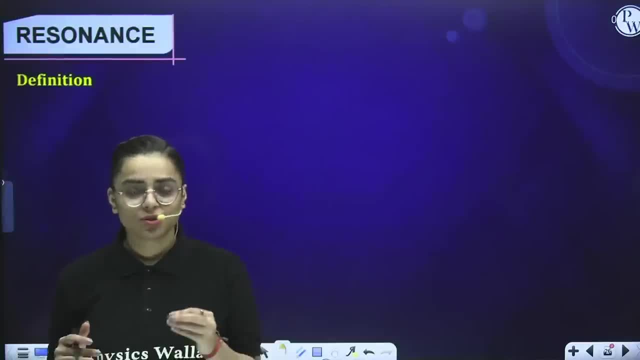 between them. now, what is resonance? to understand resonance, there were two definitions. one were the old definition and one was the new definition. according to the old definition, what do we observe? we observed that, basically, what happened? basically, let us take an example and with the help of that example, i am going to explain you the definitions also. see if 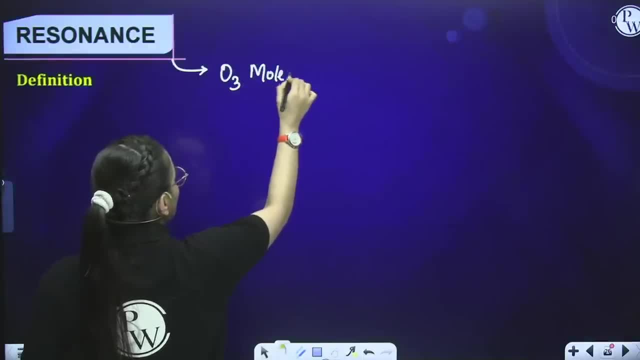 i talk about o3 molecule. if i talk about o3 molecule which looks like this: okay, now, students, in your notebooks you have seen this structure, you have already drawn also this structure, but is it the actual structure of o3 molecule? so the answer is no, a big no. 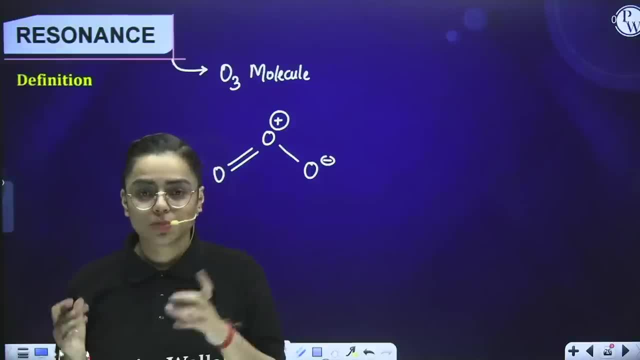 this is not the actual structure. why it is not the actual or the real structure? because if i talk about resonance, also the resonance in resonance, what do we observe? why does resonance arises? when a single structure like this is a single structure, it cannot explain the whole property of the molecule, o3 molecule. then we require a different kind of structure, similar. 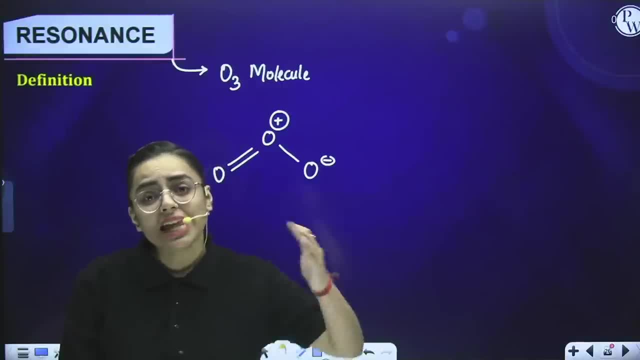 to this. you know now these structures which will explain the property of resonance. you know these structures are referred to as resonating structures. so we will make the resonating structures until when? till we get all the properties of the compound, of the molecule. so this basically single structure is unable to define or, to you know, express the properties. 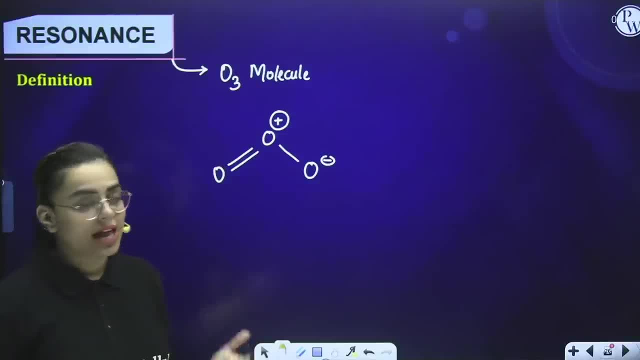 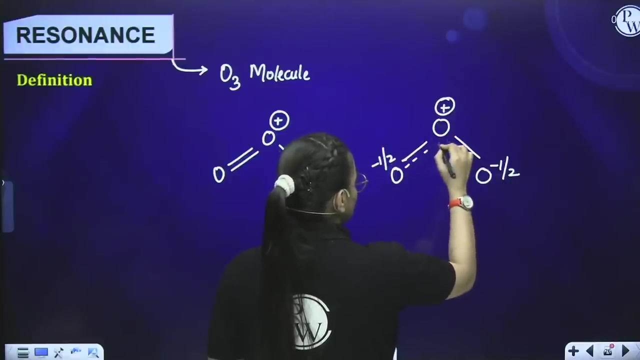 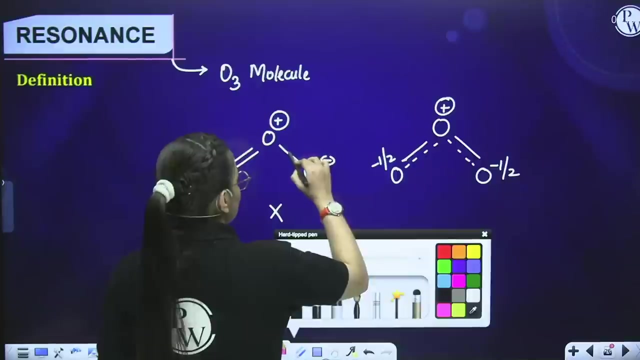 of the molecule o3, so we require more structures, and so this is not the real. however, this is: how does the real structure look like? the real structure basically looks like this. now, what is this? see, if i talk about this structure, practically what a seed. single bond is basically the longer bond and double bond is basically the shorter. 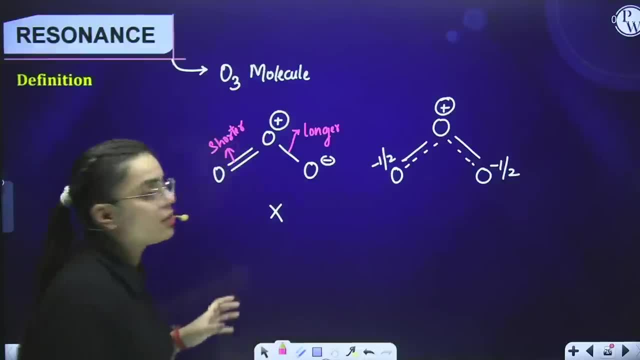 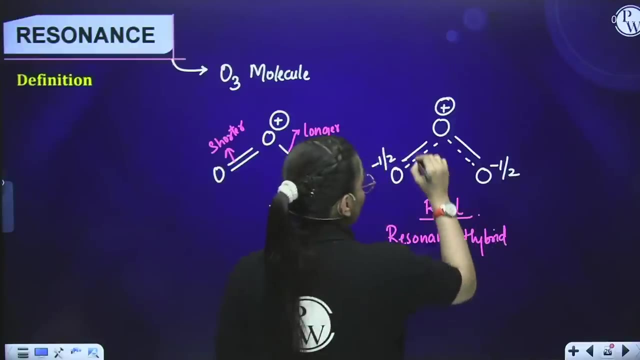 bond but, as i told you, it cannot explain the whole property of the molecule. so this is not the real structure, so this is not the real structure property. the real molecule is this one. this real molecule is resonance hybrid. this real molecule is resonance hybrid, which have all the bonds, all the bonds equal in length, equal. 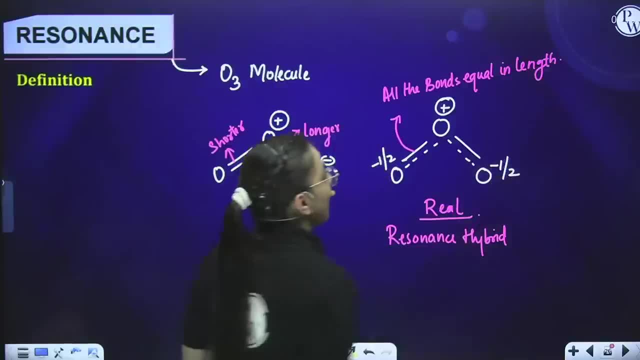 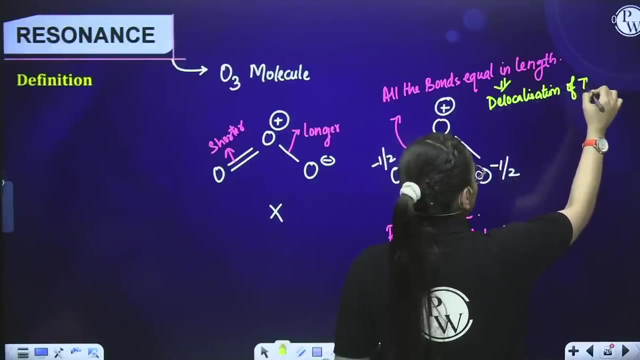 in length, and why does this happen? why does this happen? that all the bonds in this are equal in length due to: due to the delocalization of pi electrons in the conjugated system. in the conjugated system, due to this delocalization process, students, these bond lengths came to. 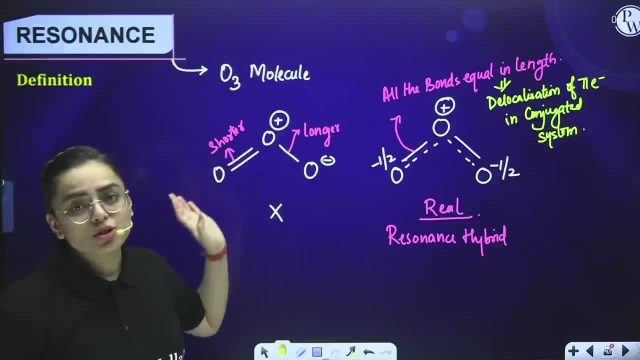 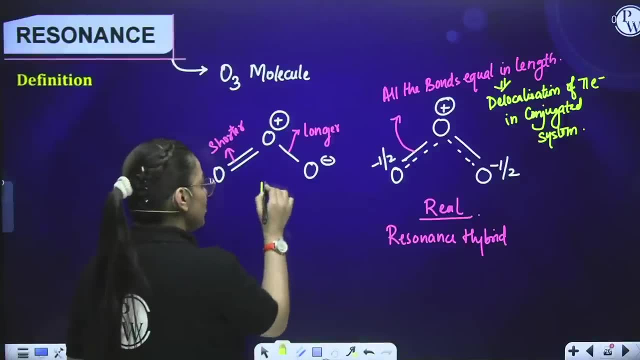 be equal, and so this structure is not the real one, because here, if you observe this, one is longer, another one is shorter, and we see that this is the kind of resonating structure, not the complete structure, not the exact structure. the exact structure basically looks like this: 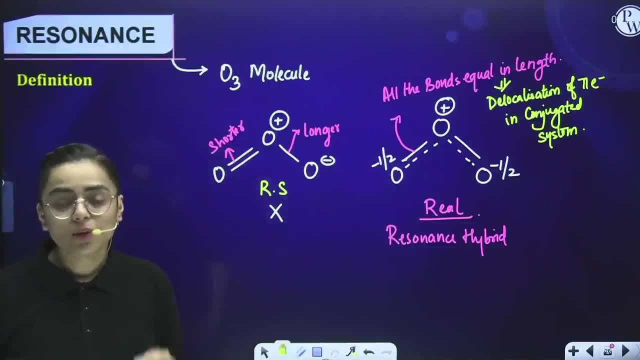 we will understand how to make resonating structure, how to make resonating hybrid in the coming topics. but first of all we need to understand that why there is a requirement of resonance. resonance was required in order to explain or to express all the properties of the molecule clear. 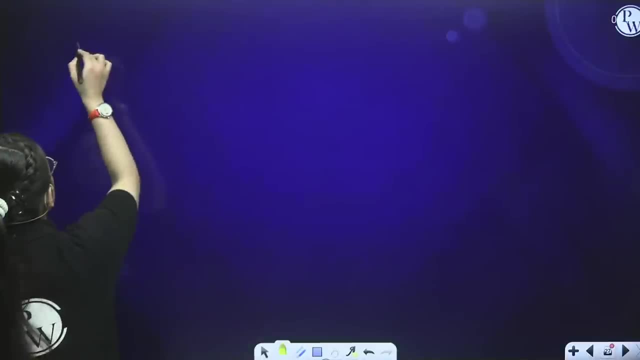 let us take one more example to clarify this concept. one is benzene. if i talk about benzene, benzene basically has two kinds of bond. one is carbon carbon single bond. another one is carbon carbon- double bond. when i talk about these two bonds, i know that carbon carbon. single bond is longer as compared to carbon carbon double bond, which is shorter. so the bond length of carbon carbon single bond comes out to be one point five, four armstrong, and carbon double bond it comes out to be 1.34 Armstrong, which is shorter. so according to: 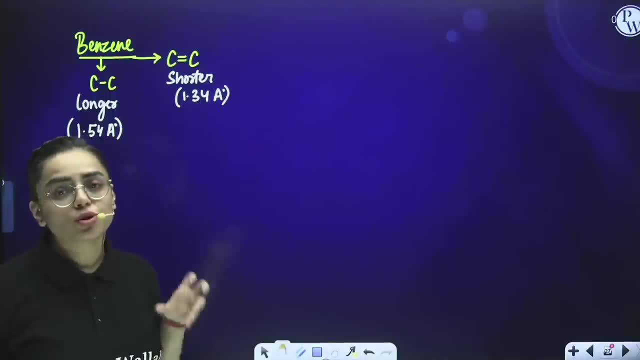 these, you know, the experimental data. if I am going to draw the structure of benzene, how would it look like? this is the you know single bond. okay, then comes double bond which is shorter in length. then comes single bond which is longer in length, then comes double. 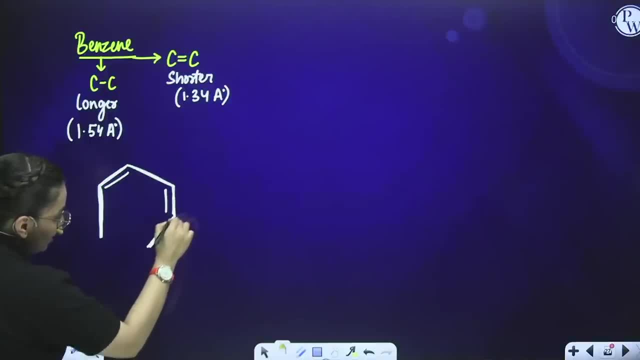 bond which is shorter in length, then comes single bond which is longer in length, then comes what double bond which is shorter in length. so this is the exact structure which should it should look like this, but it does not look like this. how does it looks? it looks. 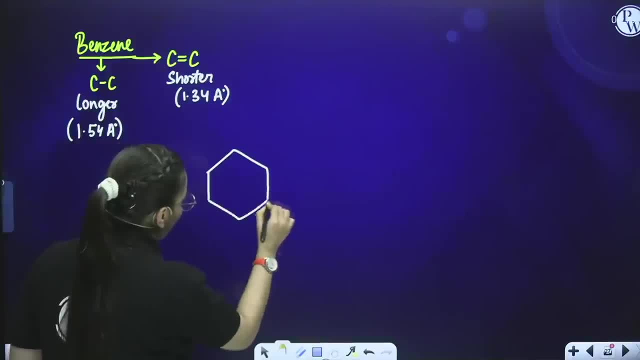 like this. now, ma'am, what you have done. you said that, okay, according to the data, the single bonds should be the longer ones and the double bond should be the shorter ones. these are all carbons According to the bond line notation. you all understand this concept, right? these are longer. 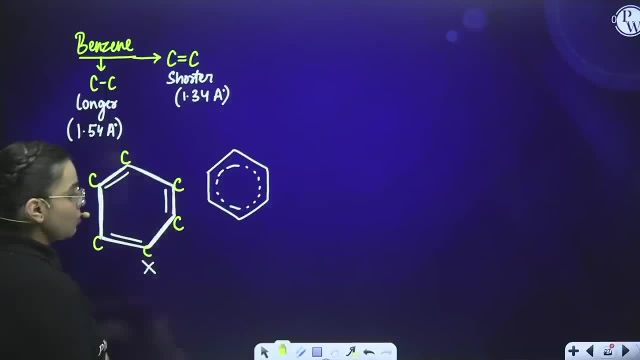 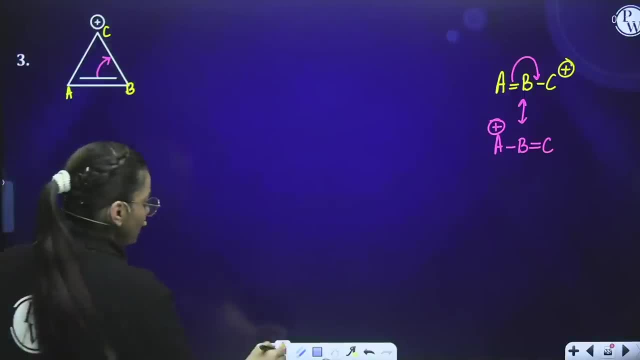 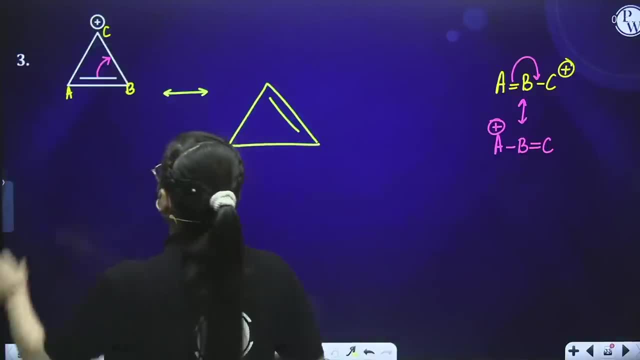 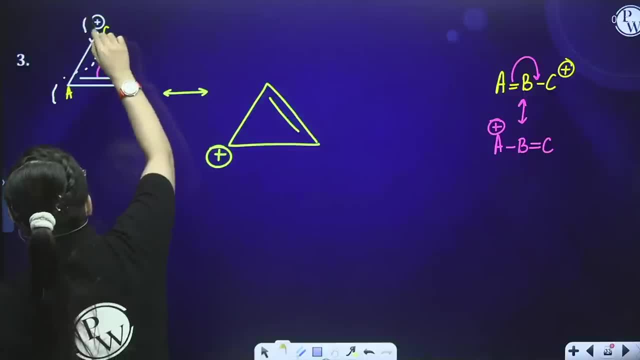 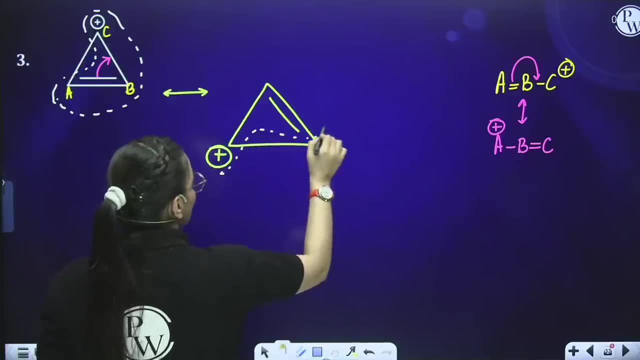 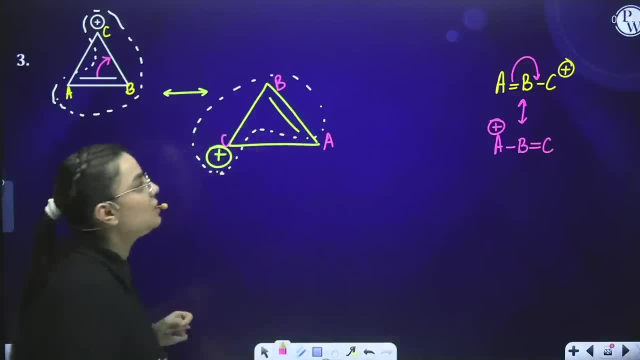 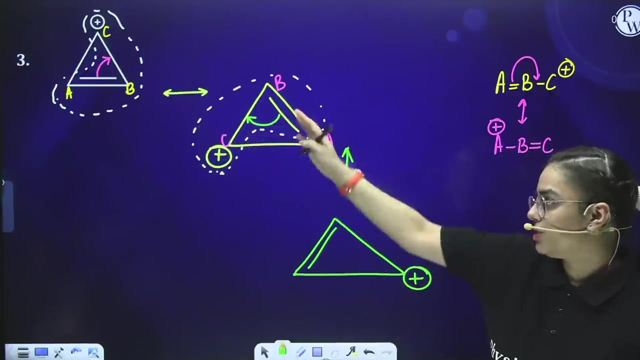 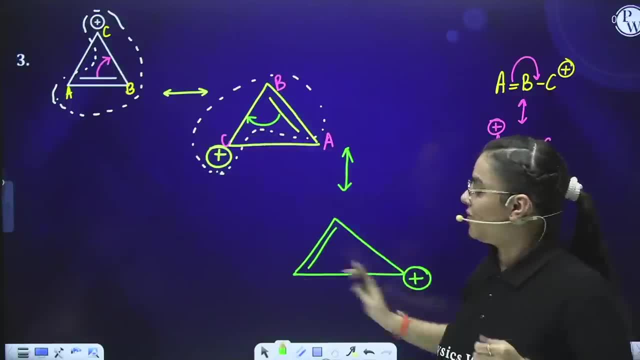 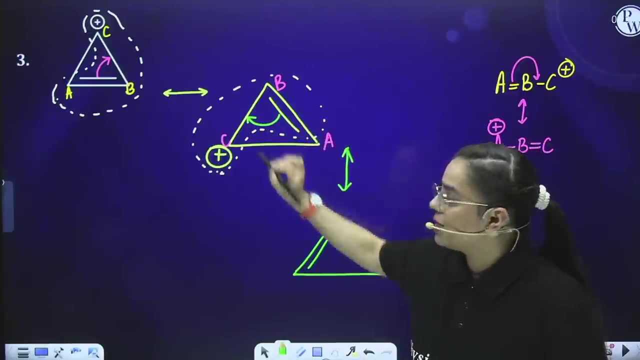 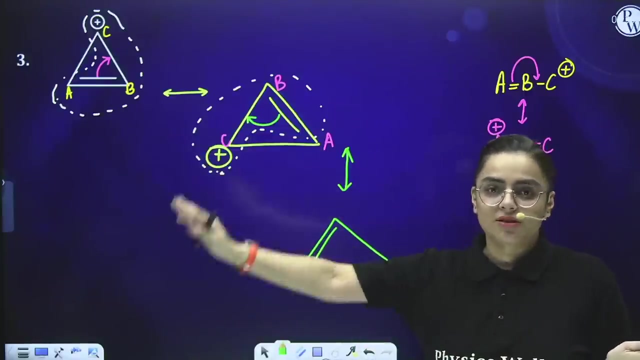 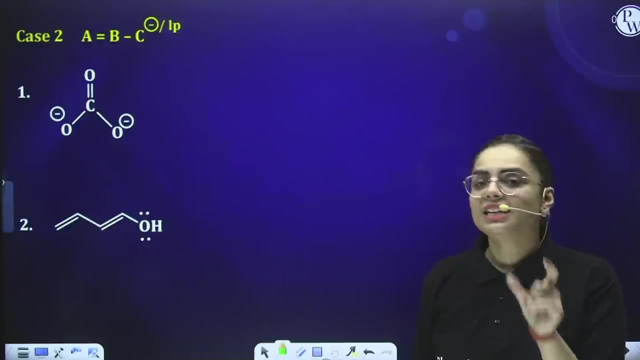 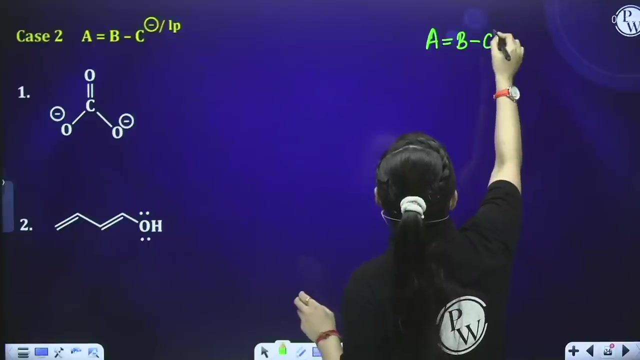 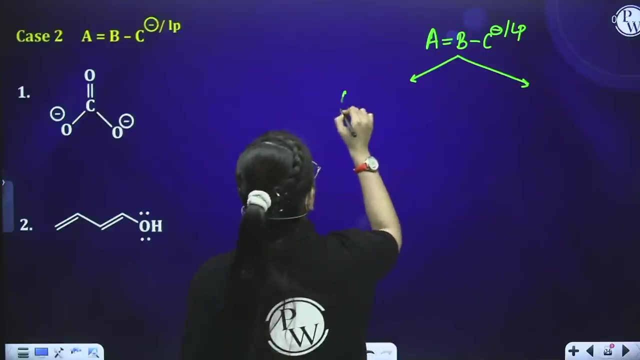 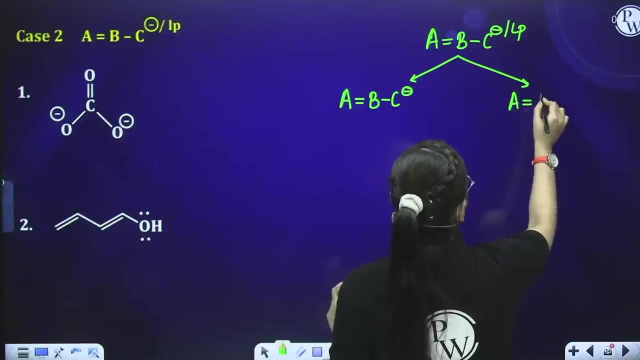 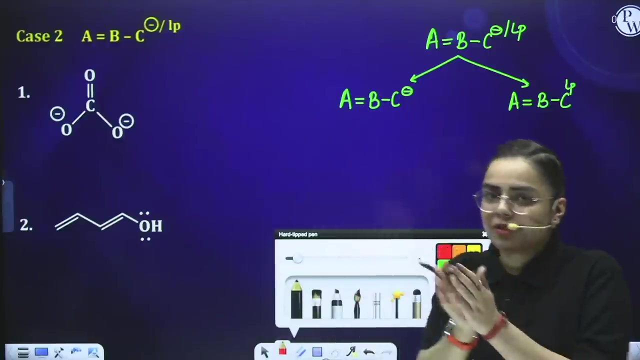 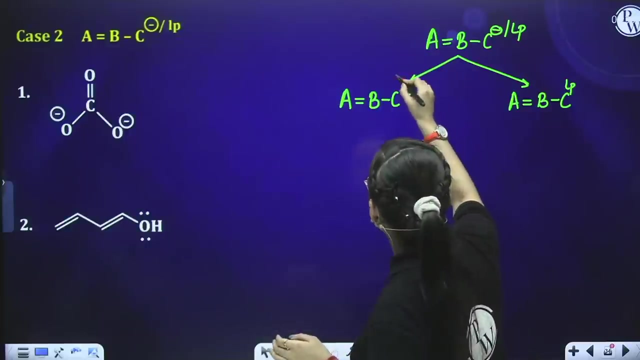 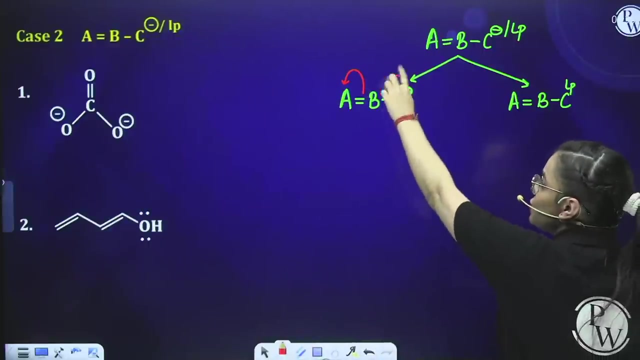 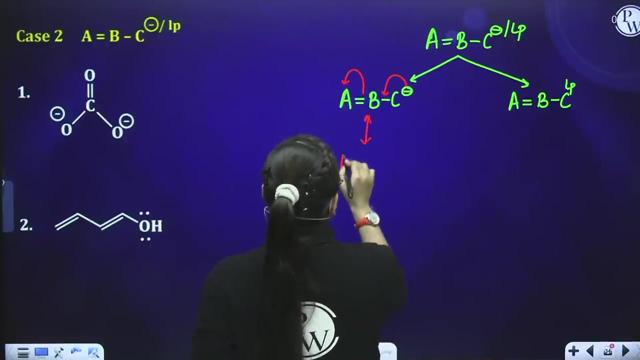 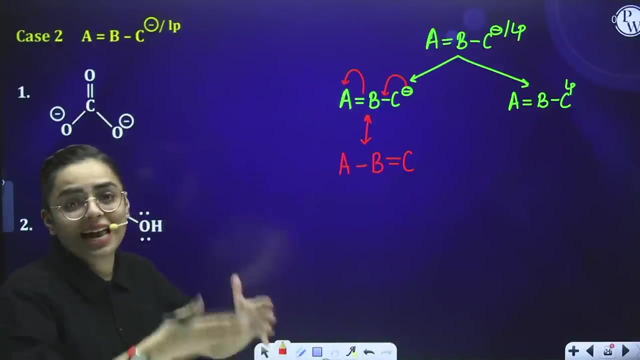 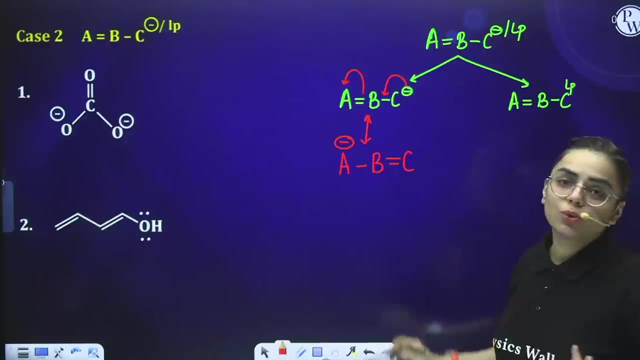 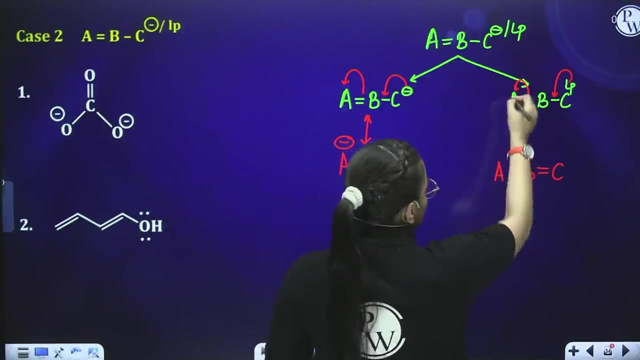 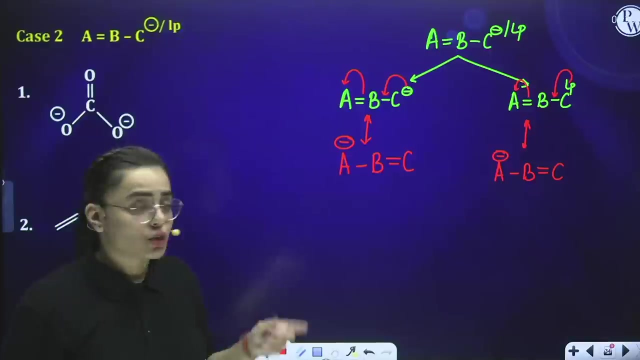